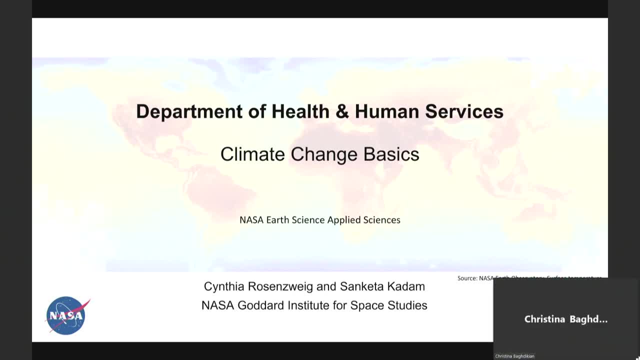 Hi everyone. My name is Sankita. I work in the climate impacts group at NASA GIS with Cynthia Rosenzweig. She's the head of our group. she usually gives this presentation with me, but unfortunately she's not here today. 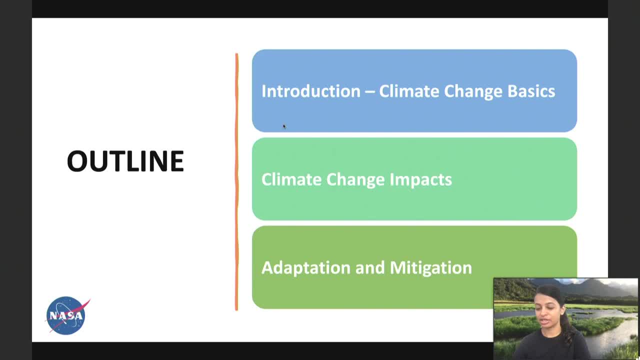 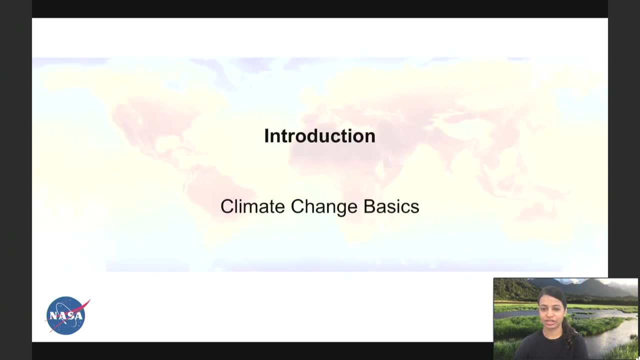 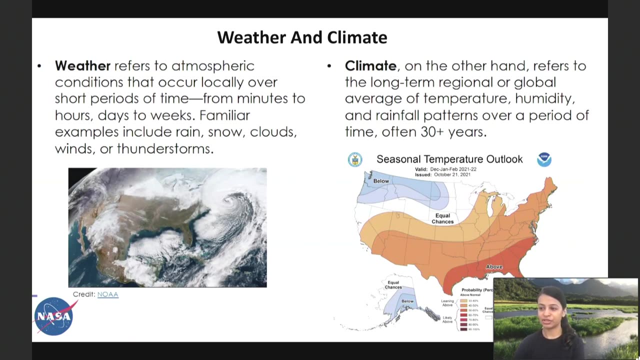 So today we'll cover three sections: introduction to climate change, basics, its impacts, adaptation and mitigation. So let's get right into it. The terms weather and climate are sometimes confused, though they refer to events on broadly different spatial and temporal scales. Weather tells you what to wear each day. Climate tells. 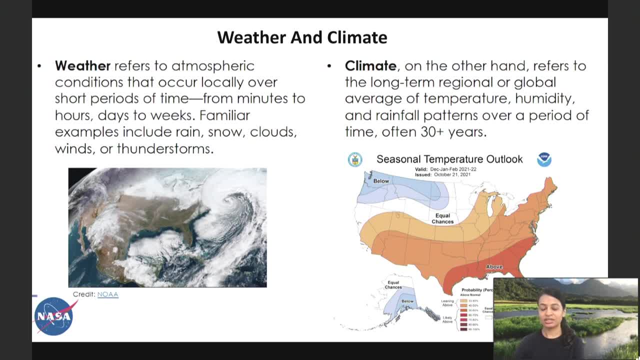 you what type of clothes to have in your closet. Similarly, the terms global warming and climate change are often used interchangeably but have distinct meanings. Weather refers to atmospheric conditions that occur locally over short periods of time, from minutes to hours, days to weeks. 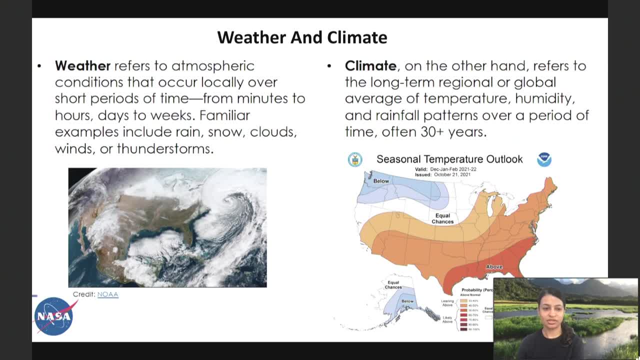 Some. Some familiar examples include rain, snow, clouds, winds or thunderstorms. Climate, on the other hand, is a long-term regional or global average of temperature, humidity and rainfall patterns over a period of time. Usually it's 30-plus years. 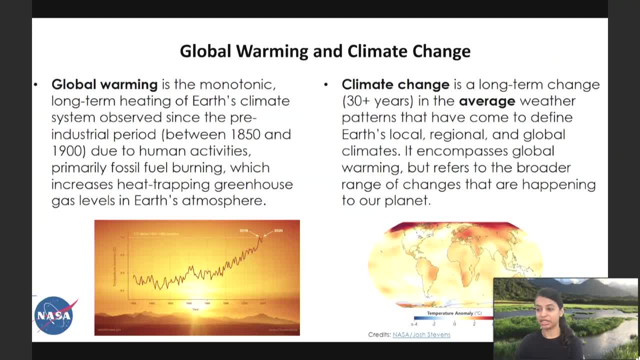 Weather can be affected by things like local humidity, air pressure on a day-to-day basis. Global warming is the monotonic long-term heating of Earth climate topic-system observed since the pre-industrial period between 1850 and 1900, due to human activities, mostly fossil fuel burning. 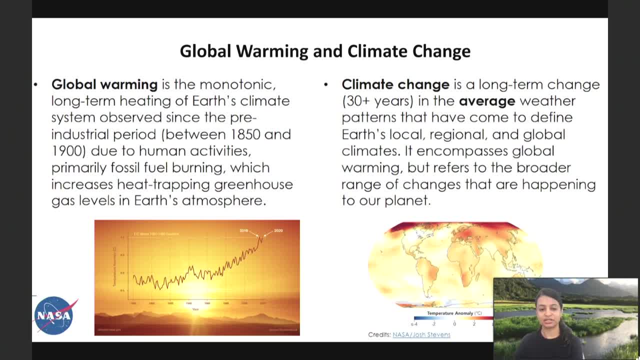 which increases heat-trapping greenhouse gas levels in the Earth's atmosphere. Climate change is a long-term change in the average weather patterns that have come to define Earth's local, regional and global climates. This, for example, hobbies 평 saya. 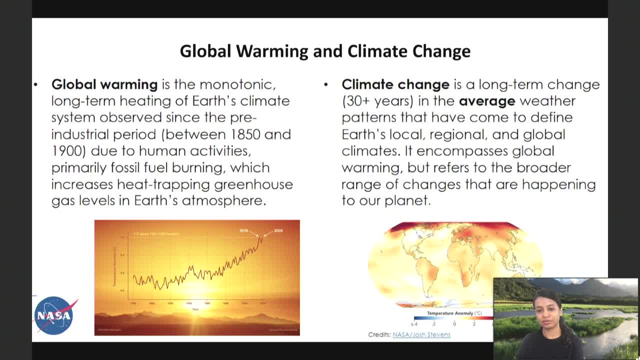 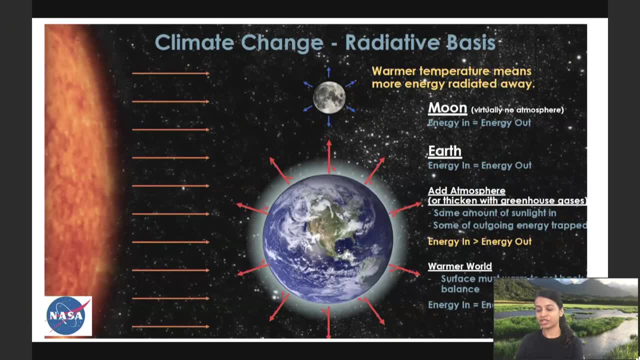 this usually includes global warming, but refers to the broader range of changes that are happening to our planet. Here is a brief introduction to the climate change radiative basis. The fundamental equation to understand is that object with warmer temperature radiates more energy away. So consider a simple setup of earth, moon and sun. 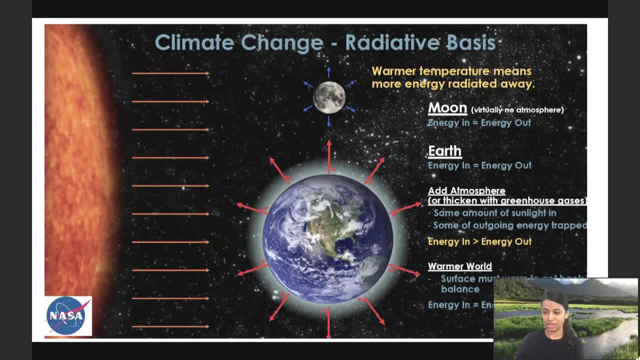 So moon has no atmosphere. In this situation, energy coming from the sun is being balanced or is equal to energy going out On earth. we have an atmosphere, So some energy is being trapped and directed back to earth because of that atmosphere. So more energy coming in than going. 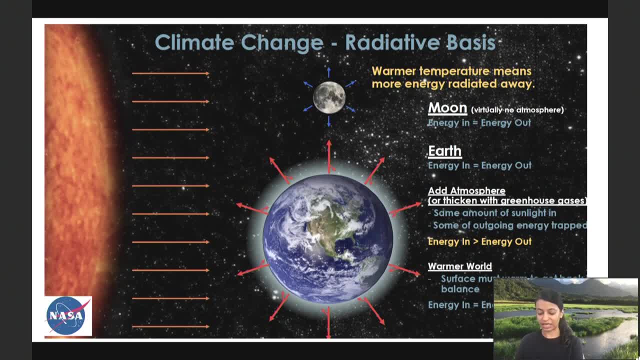 out and the planet has to warm up to balance or reach equilibrium. This is what we call the green heart. So the planet has to warm up to balance or reach equilibrium. This is what we call the green heart. So the planet has to warm up to balance or reach equilibrium. This is what we call the green heart. 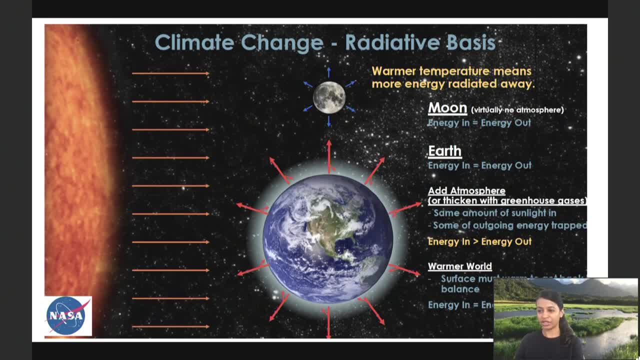 So current research in climate change is figuring out: where does the energy go? how do all the earth systems take that energy in and react to it? systems like oceans, ice, land surface vegetation- And this energy changes the way climate behaves. 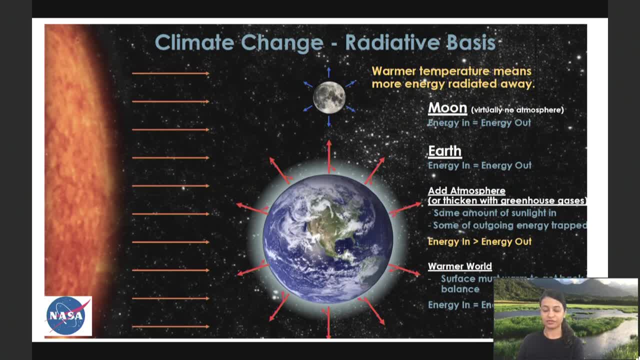 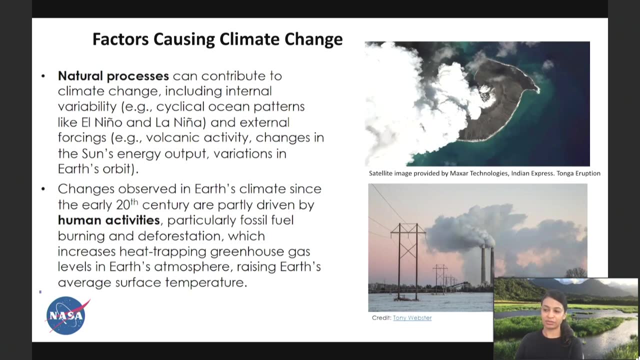 changes in rainfall patterns, wind, extreme events, feedback systems, et cetera, which in turn affects the society that we live in. So natural variability has always been a part of earth's climate system. Earth has gone through periods of cooling and warming. 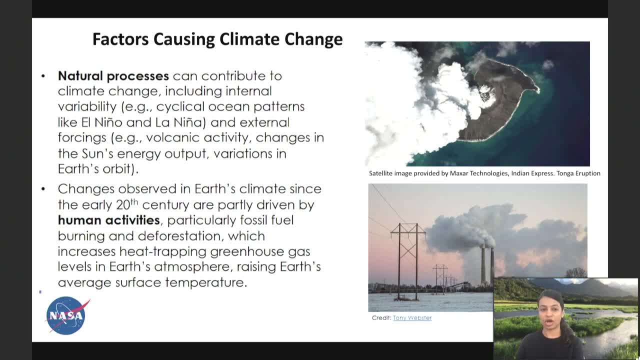 And to understand climate change, we need to understand the causes. Natural processes can contribute to climate change, including internal variability- Example: ocean patterns like El Nino and La Nina- and external forcing. So we need to understand the causes. Natural processes can. contribute to climate change, including internal variability- Example: ocean patterns like El Nino and La Nina- and external forcing. So we need to understand the causes. Natural processes can contribute to climate change, including internal variability- Example: ocean patterns like El Nino and. 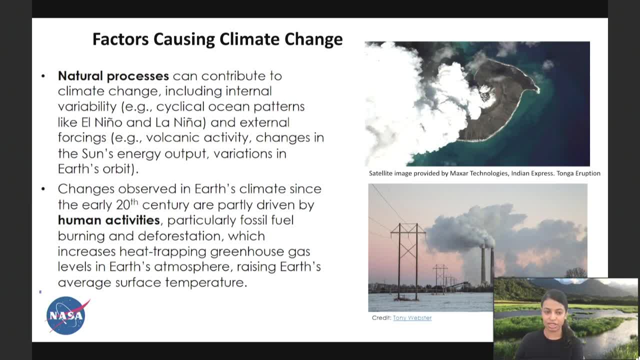 La Nina and external forcing. So we need to understand the causes. Natural processes can contribute to climate change, including internal variability. Example: ocean patterns like listen, changes in sun's energy output, variations in the Earth's orbit, changeswife observed in earth's climate since the early 20th century are partly driven by 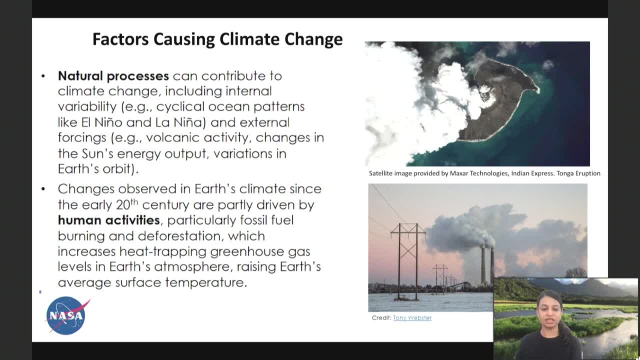 human activity, and particularly fossil fuel burning and deforestation. These natural causes are still in play, but their influence is too small and too slow to explain that rapid warming that we have in the climate system. So we need to actually get the robots high energy. 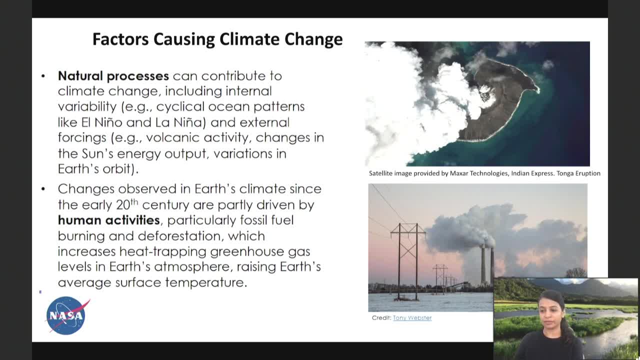 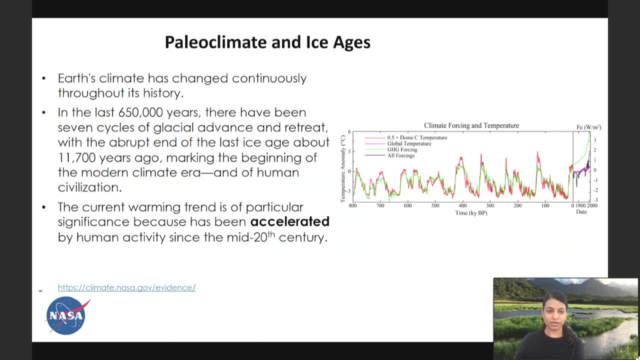 and적 problems compromised by the natural forces. So the results of environmental that we have seen recently in the early 20th century. So Earth's climate has changed continuously throughout its history. In the last 650,000 years there have been seven cycles of glacial advance and retreat. 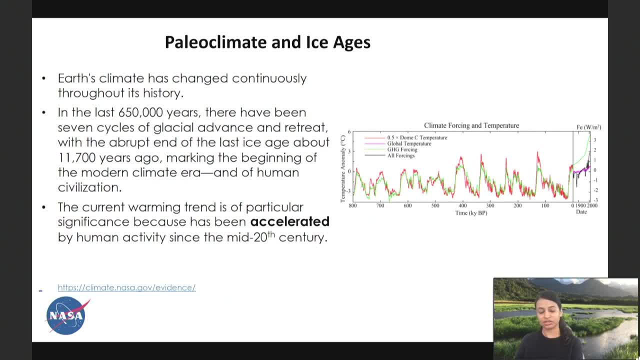 with the abrupt end of the last ice age about 11,700 years ago, marking the beginning of modern climate era And of human civilization. It's important to note that the current warming trend is of particular significance because it has been accelerated by human activity since the mid-20th century. 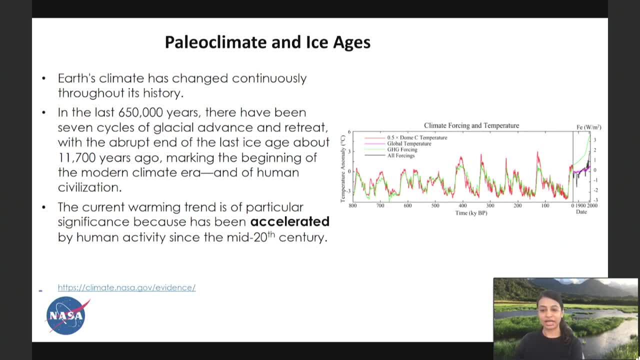 And that's what the graph on the right is showing, is from the 1900 to 2000 and beyond. we see an accelerated upward trend in warming In paleoclimate and ice ages. through studying ice cores, we know that CO2 concentrations during the warming periods that followed the ice ages 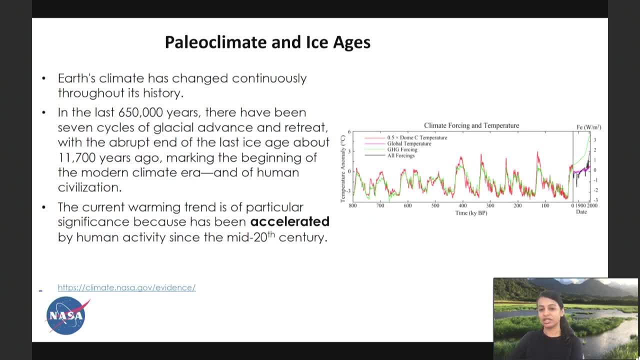 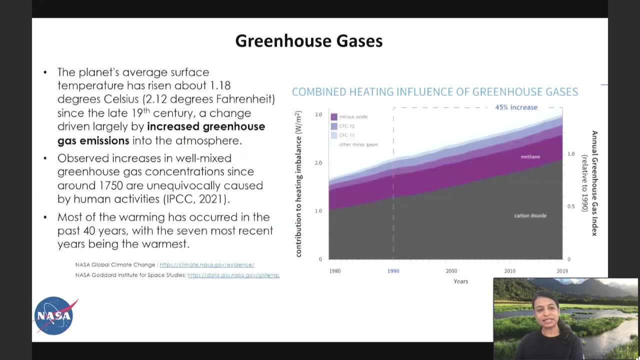 that we see on the graph here has never exceeded 300 parts per million, which, when I checked yesterday, we are at 420 parts per million, which is pretty high for Earth's history. The planet's average surface temperature has risen about 1.18 degrees Celsius. 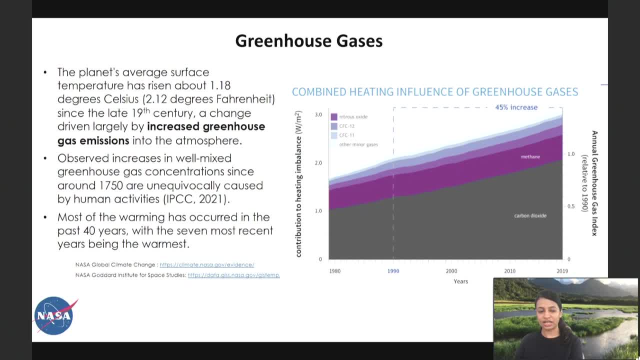 since the late 19th century, A change driven largely by increased greenhouse gas emissions into the atmosphere. Observed increases in well-mixed greenhouse gas concentrations since around 1750 are unequivocally caused by human activities, And most of the warming has occurred in the past 40 years. 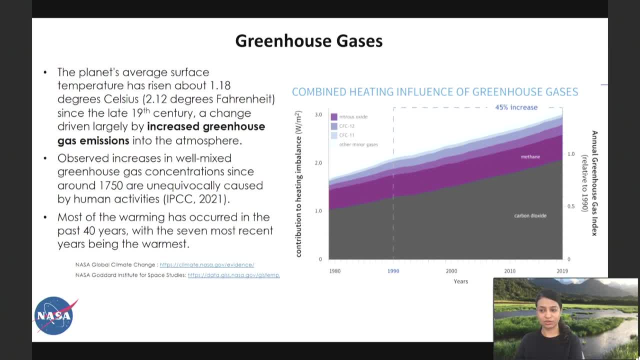 with seven most recent years being the warmest, which 2016 and 2020 were the warmest years. So why does carbon dioxide matter? CO2 is a very important component of climate change. CO2 is a very important component of climate change. 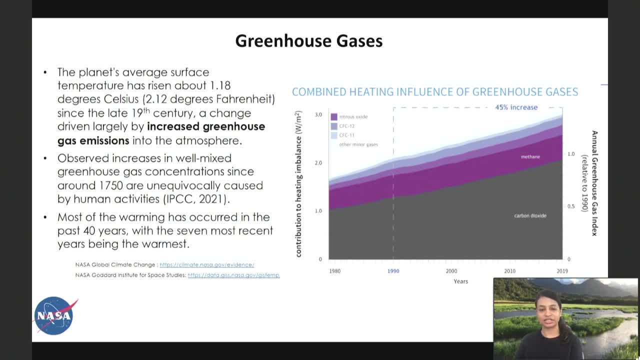 CO2 is a very important component of climate change. CO2 is the most important of Earth's long-lived greenhouse gases. It absorbs less heat per molecule than, say, nitrous oxide or methane, but it's more abundant and it stays in the atmosphere longer. 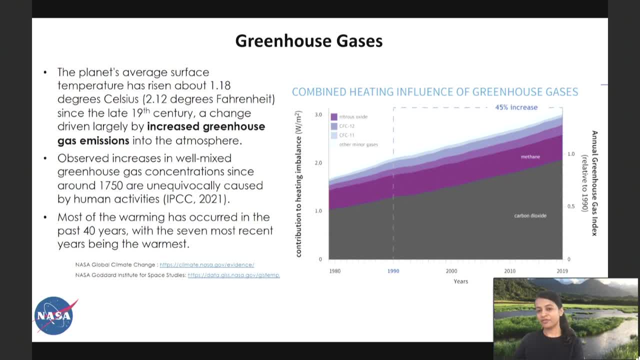 It's about 300 to 1,000 years, And the graph here on the right shows the heating imbalance caused by the combined influence of greenhouse gases. But what we can see here is that carbon dioxide- carbon dioxide is so abundant in the atmosphere. 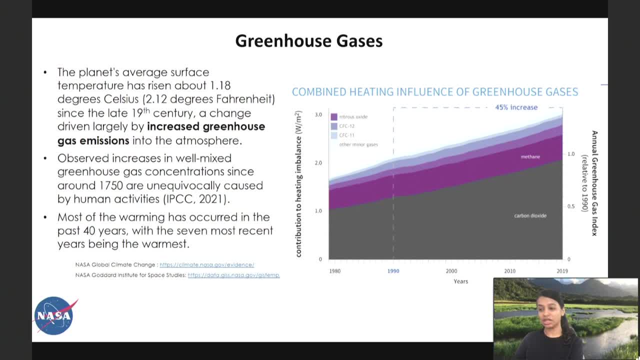 that it is responsible for about two-thirds of total energy imbalance, And since the 1990s we have seen about a 45% increase in the combined amount of all these gases in the atmosphere. So prior to industrial revolution, the CO2 concentrations were fairly stable at around 280 parts per million. 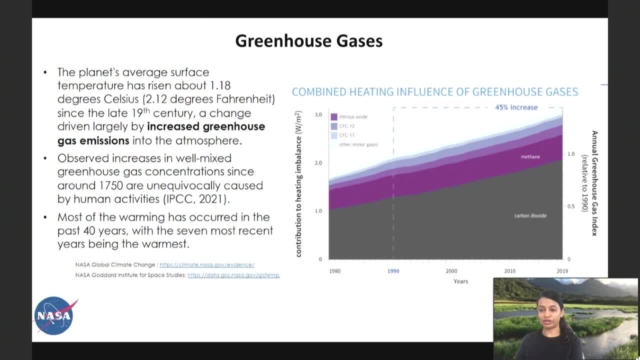 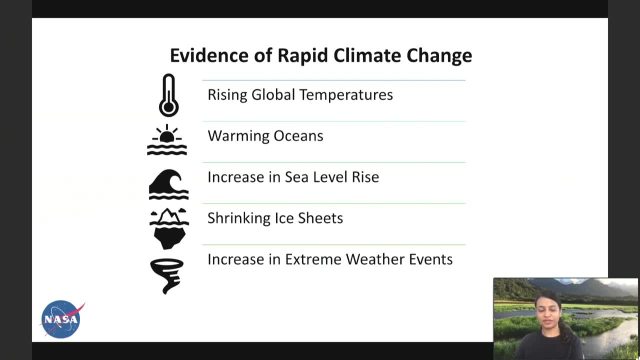 By 2020, they had risen to more than 48%, Following the multiple lines of evidence. philosophy, scientists study various systems for evidence of climate change, such as rising global temperatures, warming oceans, increase in sea level rise, shrinking ice seeds. 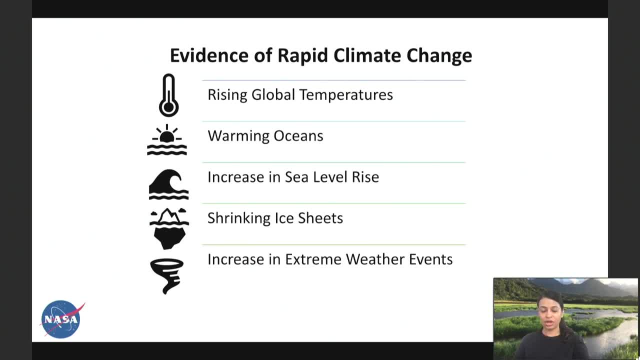 and increase in extreme weather events. Oceans, we know, act as a heat sink, But recently we have seen that the top 100 meters of ocean has shown warming of about 0.34 degrees Celsius. More than 90% of global warming goes into the oceans. 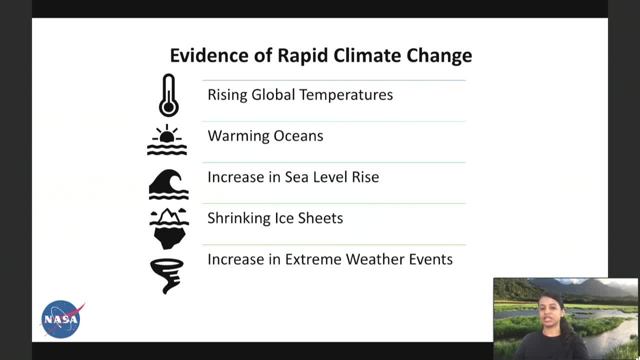 which means that the warming oceans also result in shrinking ice sheets and more sea level rise. It's virtually certain that hot extremes have become more frequent and more intense. The frequency and intensity of the warming of oceans and intensity of heavy precipitation events have both increased. 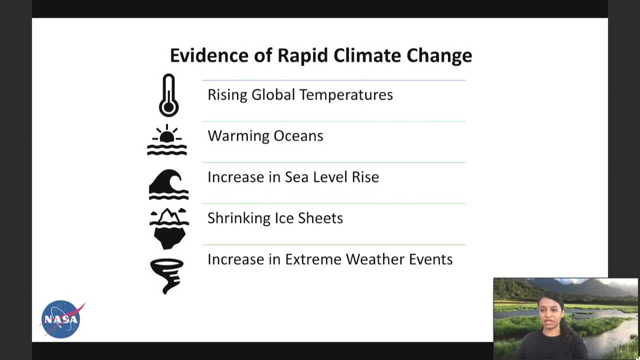 And these are all observations, events that we are seeing right now. today, The impacts of climate change are no longer a distant future. It's no longer 2050.. And in the future, these are the impacts that we are seeing today. 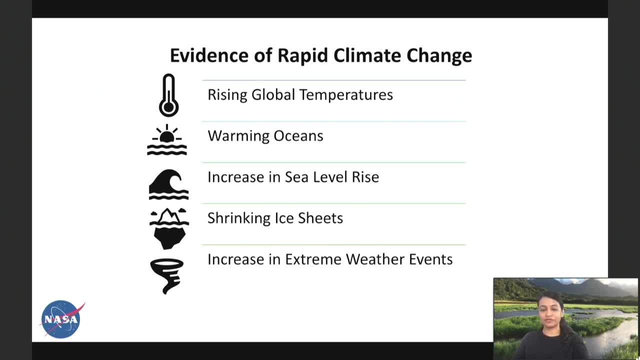 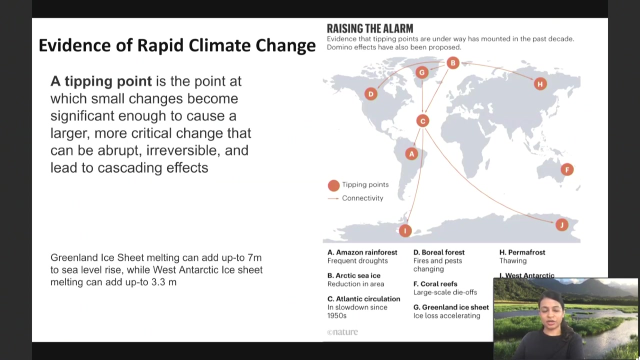 The global proportion of category 3 and 5 tropical cyclones has increased. We had an extremely active hurricane season in 2020 and 2021, with record-breaking 30, or more than 30 named storms in 2020.. Climate scientists separate factors that affect climate change into three broad categories. 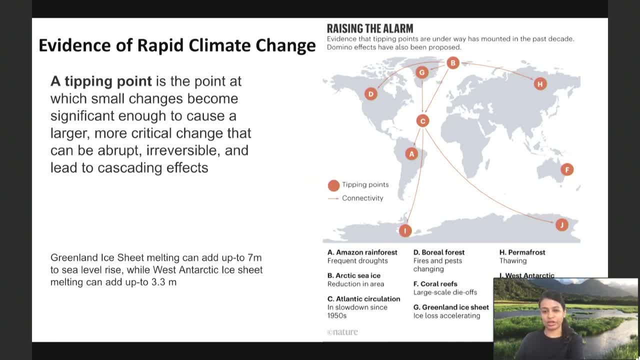 It's forcings, feedbacks and tipping points. Forcings is usually the energy imbalance caused by the initial change. Forcings are the initial drivers of climate, such as solar irradiance, greenhouse gas emissions, et cetera. 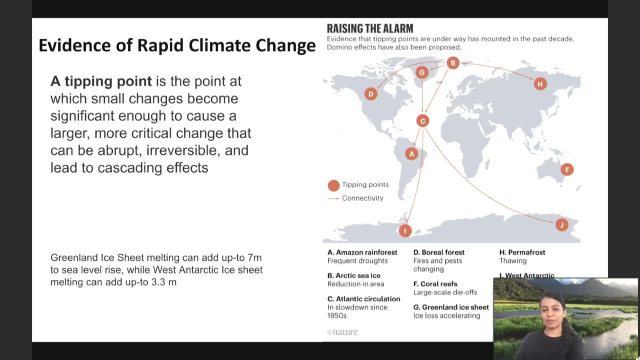 Feedbacks are processes that can either amplify or diminish the effect of a forcing. So, for example, ice albedo have a warming effect or positive feedback, And we can talk about that more in the FAQ section. A tipping point is a point at which small changes become significant enough to cause. 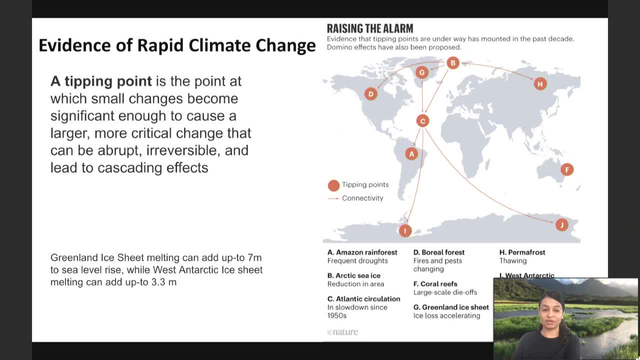 a larger, more critical change that can be abrupt and, very importantly, irreversible and lead to cascading effects. So, for example, Greenland ice sheet melting- completely melting, can add up to seven meters to sea level rise, while West Antarctic ice sheet melting can add up to 3.3 meters to sea level rise. 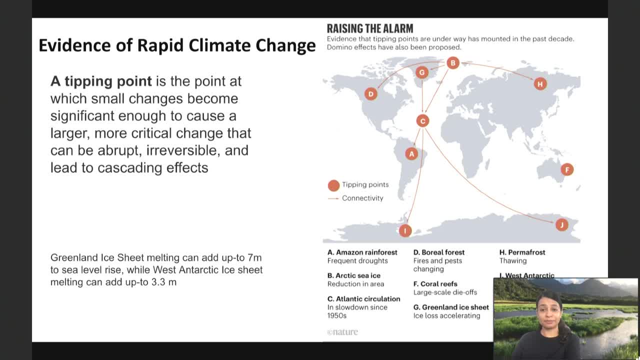 And on the right here we see a map of different tipping points Around the world. we see the Amazon rainforest, the Arctic sea ice, the boreal forest, the coral reefs, the permafrost, the Atlantic circulation. passing an irreversible tipping point would mean that our climate 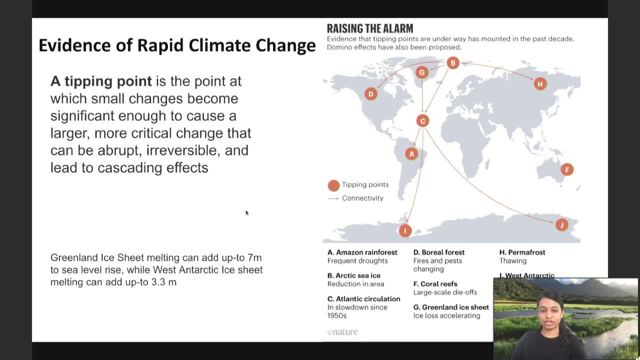 system cannot revert back to its original state. Another example that I wanted to mention here is the AMOC, or the Atlantic Meridional Overturning Circulation, which is the sea here that we see on the map. So Gulf Stream, that is part of this AMOC, is being weakened by climate change. 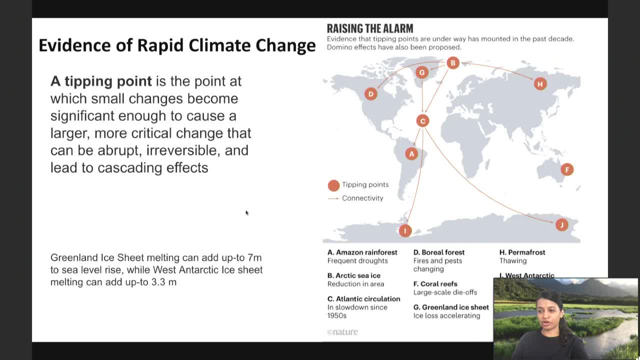 It's a system that brings warm water up to Europe from the tropics and beyond. The AMOC forms part of a wider network of global ocean circulation. It transports heat all around the globe, And recent research suggests that AMOC has been weakened by about 15 percent. 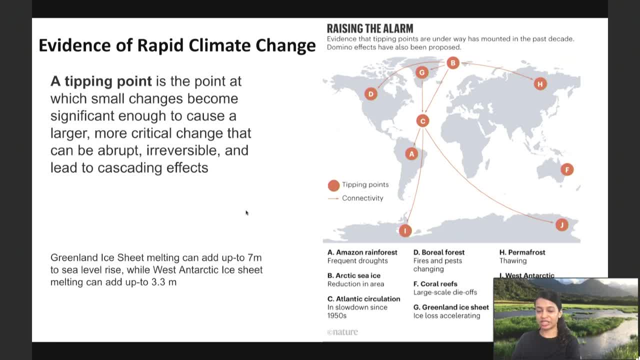 And a complete shutdown would cause widespread cooling around the whole of the northern hemisphere, And it can. the winter temperatures can fall by up to four degrees Celsius, But the models are not predicting this for at least another 100 years, And this would require that the global warming level reaches four degrees Celsius. 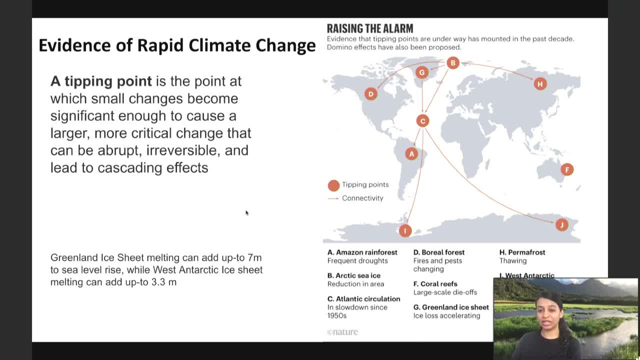 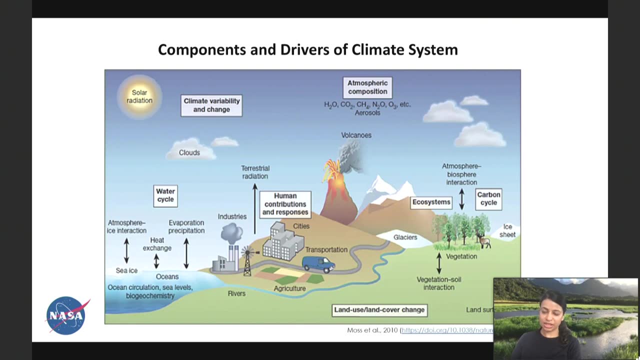 So there's a lot of uncertainty around a complete shutdown of AMOC, But we definitely have evidence that it's weakened and it's slowing down. When we're talking about systems, what we're trying to do is understand the interactions between the components of this climate system. Climate system interacts with oceans, ice, ecosystems. 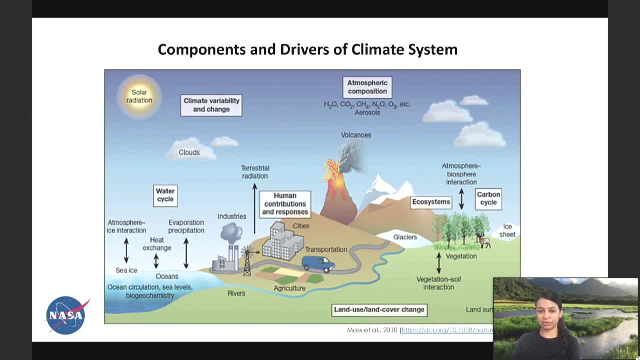 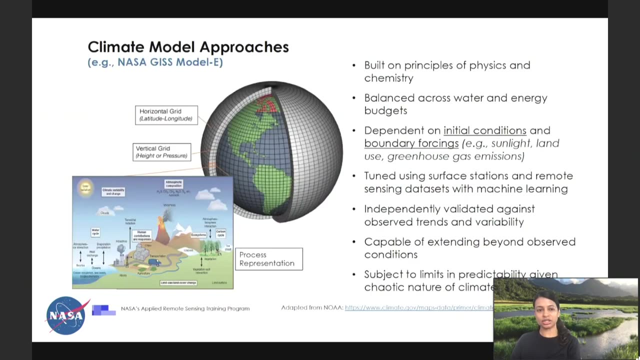 And that is what is happening in the rest of the world. We're developing a very complex and exciting technology. You know, we are even using the human world to understand how this climate will affect our ecosystems. What we also see here are the human driven components, like land use change, vegetation change. 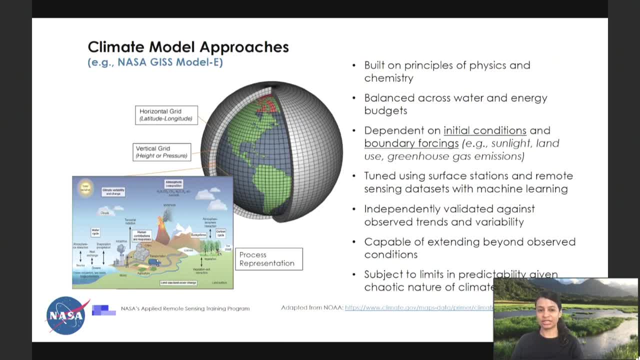 They also have impact on the overall system. They're all connected and they all interact with each other. equations: We, particularly at NASA, work on the NASA GIS climate model here at the Goddard Institute of Space Studies using supercomputers. This climate model is built on principles. 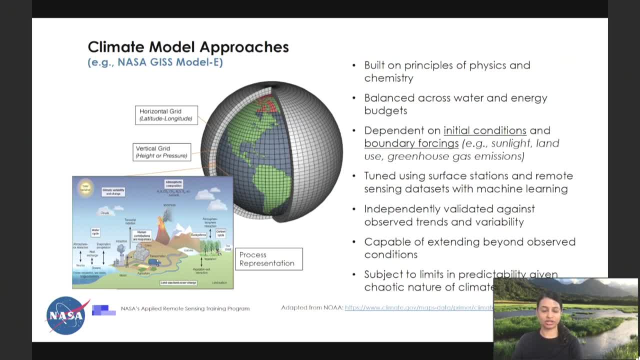 of physics and chemistry. It's balanced across water and energy budgets. It's dependent on initial conditions and boundary forcing, so we give it initial conditions of the amount of greenhouse gas emissions in the atmosphere, the amount of sunlight received. what is the land use? It's tuned using surfacitations and remote sensing data sets with machine. 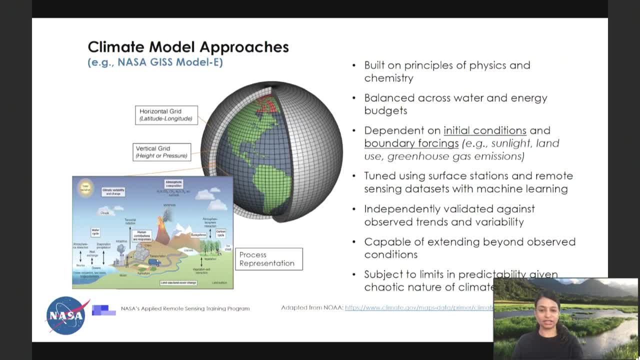 learning. It is independently validated against observed trends in variability, so against observations and past trends. The models are capable of extending beyond observed conditions. So we not only project into the picture the future, we also project into the past. It's called hindcasts and that's how we compare to 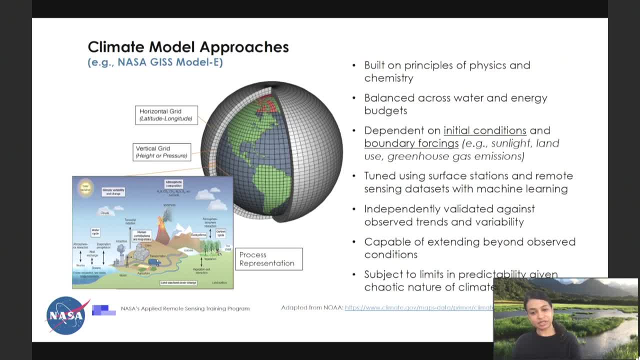 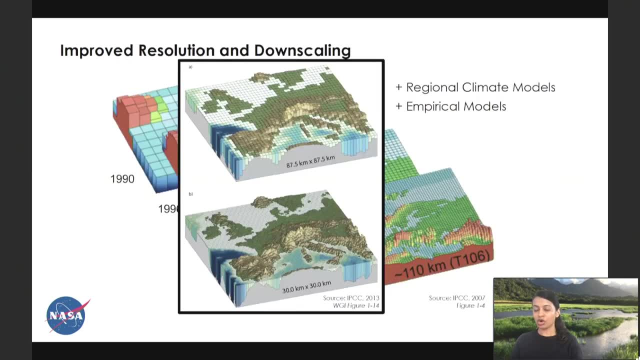 observations. It's subject to limits and predictability, given chaotic nature of the climate system. Over time, with more computational power, we have improved our resolution of these models. from 1990s to now We have come. we've come far. We've come from 500 kilometers to about. 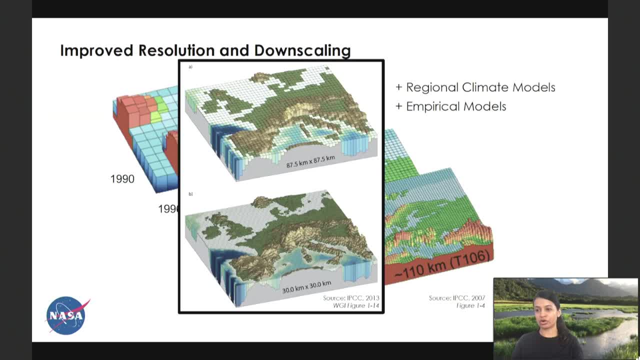 100 kilometers and we always have more ways to go. but we can also further extend it by using regional climate models and empirical models, that they use statistical approaches to downscale the climate model to a more lower resolution. So we go down to up to 25 to 50 kilometers now. 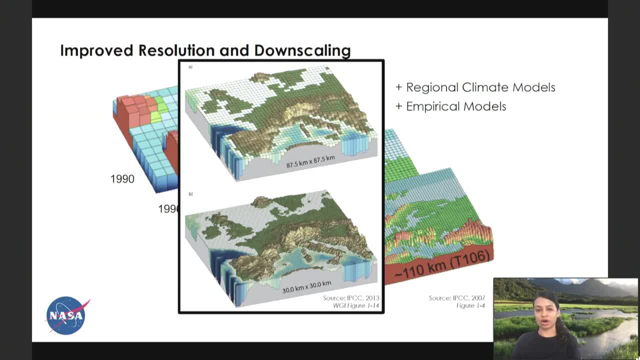 And so climate models were designed to understand the response to combined and individual driving factors Like methane, CO2,, et cetera, but to also understand the impacts of policy choices, to get a forewarning of the need of adaptation and based on what's coming, They are not designed. 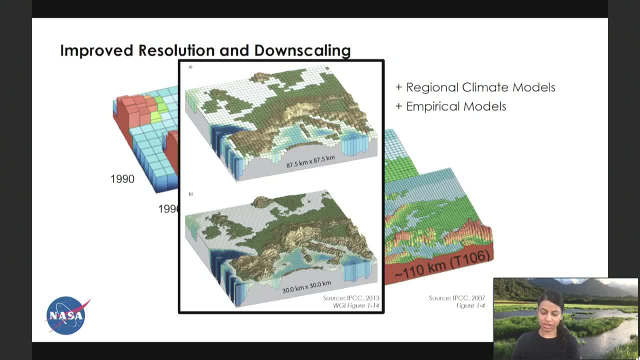 for perfect short-term and long-term predictions. So, for example, for daily or hourly forecast, we usually look at weather models versus climate models. They are not designed to study local climate models, but they provide truly local information because of the resolution available, and hence that's the necessity of bottom-up approaches when thinking of solutions. 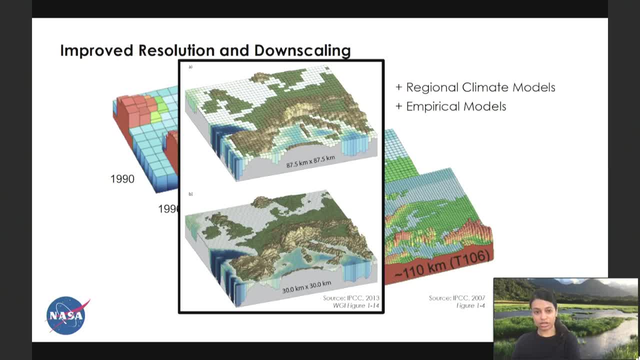 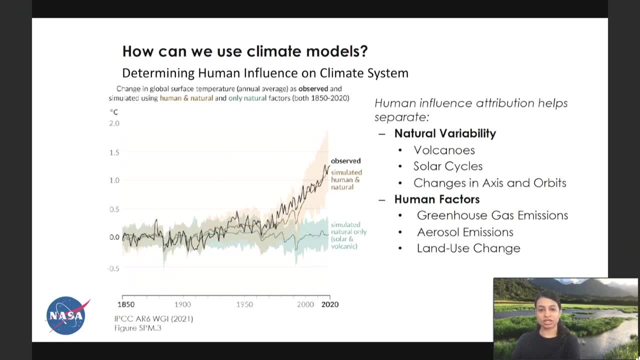 on smaller scales, and we will learn about this more in the adaptation section. So how can we use climate models? Mostly, we have seen that it's been very useful in determining human influence on climate system. In the green here on the graph, in the green cloud, we see simulations using climate models where only natural variability was included, and this shows a stable climate. 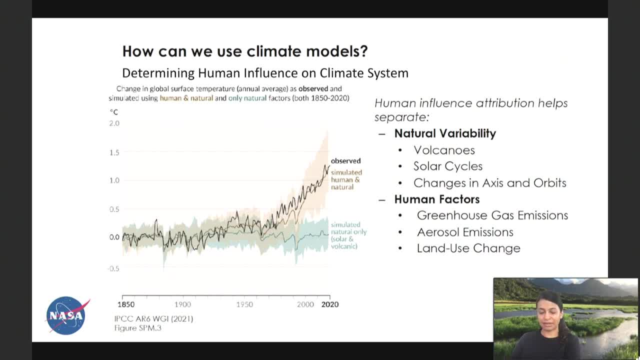 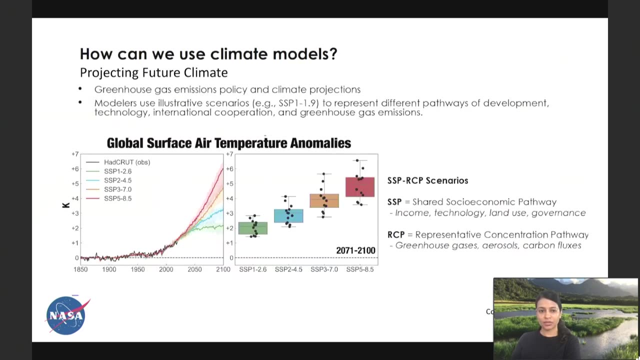 But when we look at the actual observations, which is in the black here? climate models only follow this in their hindcast. when we factor in greenhouse gas emissions, aerosol emissions, showing the human influence on climate system. Looking forward into the future, we use scenarios to represent pathways of development, technologies and, most importantly, the amount of greenhouse gas emissions into the future. 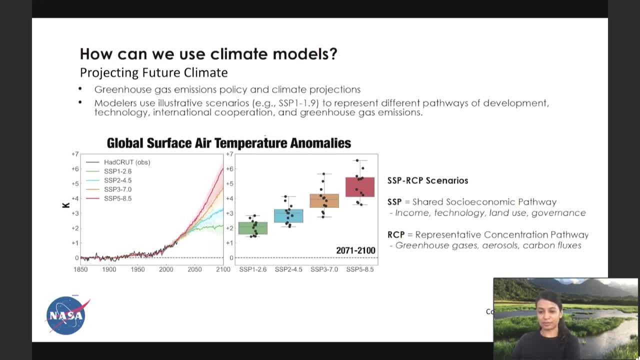 So in this graph here from IPCC, we see that IPCC, that is the Intergovernmental Panel on Climate Change- that brings together about hundreds of scientists and experts and policymakers from all around the world and they release a report. And they release a report on the current state of climate change, the latest science and information. 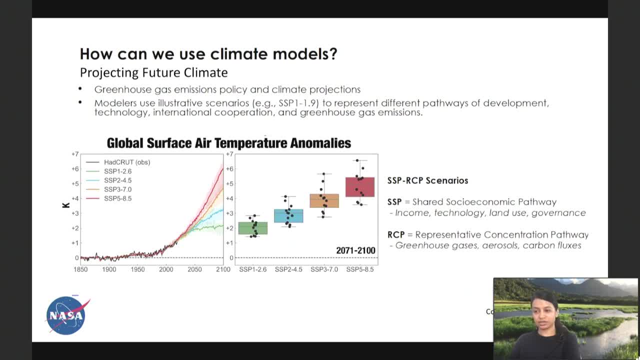 And what we've seen in this is that the SSPs, which is the shared socioeconomic pathways, which shows you the scenarios of different income, technology, land use and government strategies into the future, are combined with RCPs, which is: 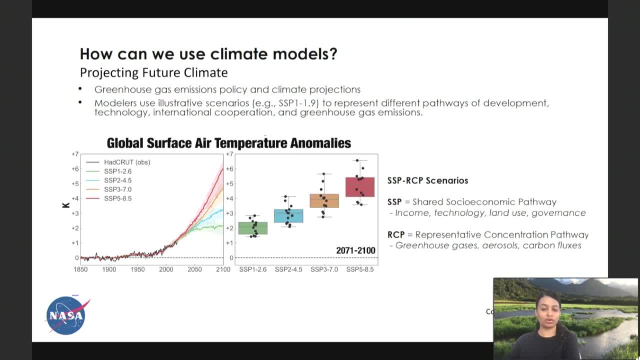 Which is the representative concentration pathways that show the carbon fluxes, the greenhouse gases, the aerosol emissions. This graph uses climate models from CMIP6, which is the Couple Model Intercomparison project, phase six, Which is a set of common protocols followed by climate modelers all around the world. 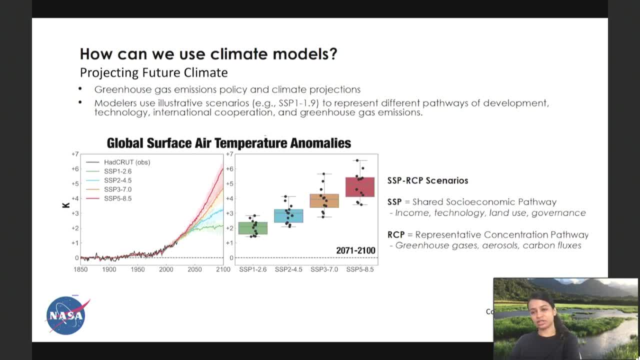 And it is important to note that the uncertainty rates appear to be pretty relative around the globe- And some of the mentally nourished studies in this- And this is also something that I'm very 남자- And some of the mentally nourished studies in this. 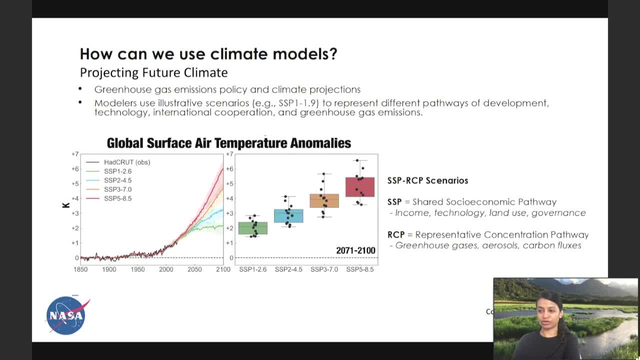 And some of the mentally nourished studies in this And some of the mentally Voor gesture And some of the mentally rude الجzentlyiger Jarrood University And some of the mentally rude Jarrood University, that the uncertainty range in each scenario is across models, which is less than compared to 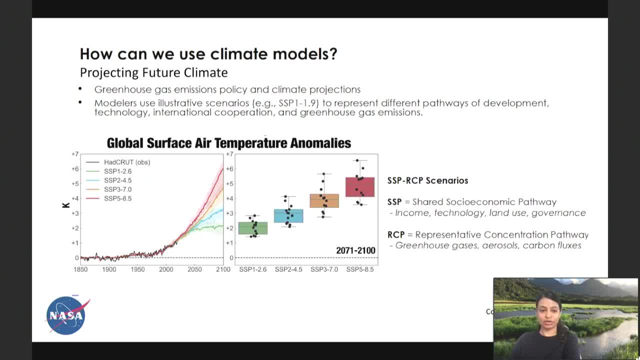 the uncertainty range across scenarios. So if we were to have a world where the greenhouse gas emissions were lower or curbed in time, we would have lesser warming than compared to the scenario where it's a business as usual. So the red line you see in the graph SSP 5, 8.5, we call it. 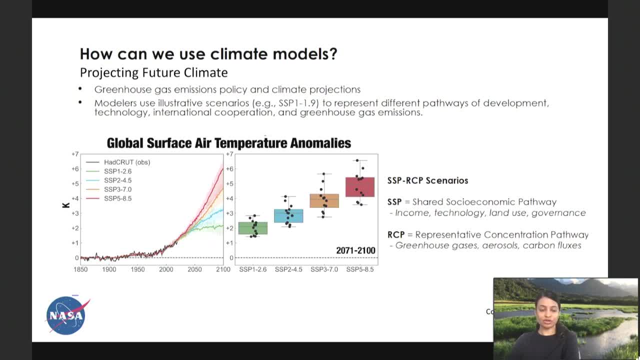 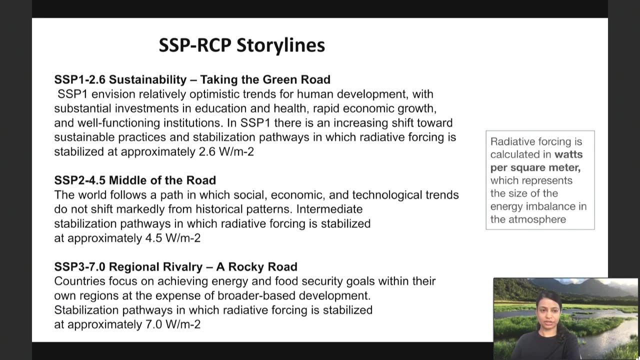 business as usual scenario That gives you a higher warming than a world where we are curbing our emissions. So let's look at these SSP RCP scenarios in depth. So the first one is the SSP 2.6, which is the sustainability or taking the green road scenario, which envisions relatively 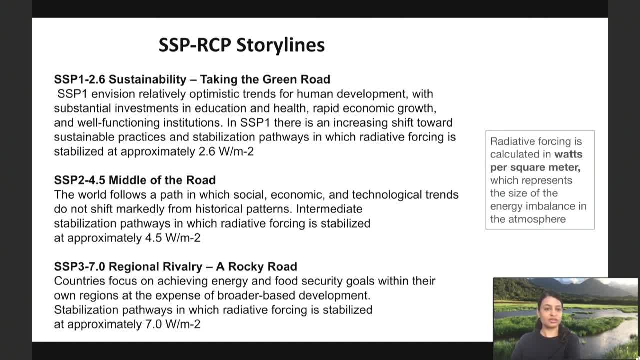 optimistic trends for human development, With substantial investments in education, health, economic growth and well-functioning institution. In SSP 1,, there is an increasing shift towards sustainable practices and green practices And the stabilization pathways in which radiative forcing is stabilized at approximately 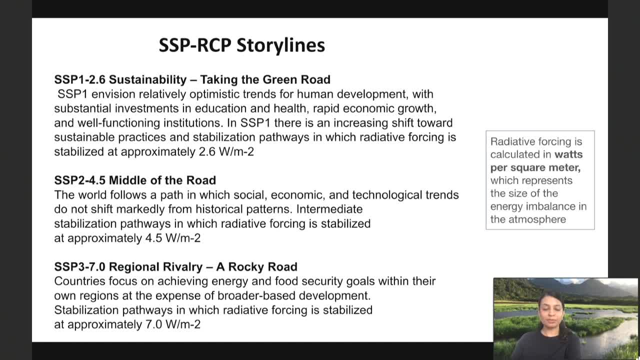 2.6 watts per meter squared. This simply means that we reduce our greenhouse gas emissions and curb our greenhouse gas emissions. The second is called the middle of the road. The world follows a path in which social, economic and technological trends do not shift markedly from historical patterns. It's an intermediate. 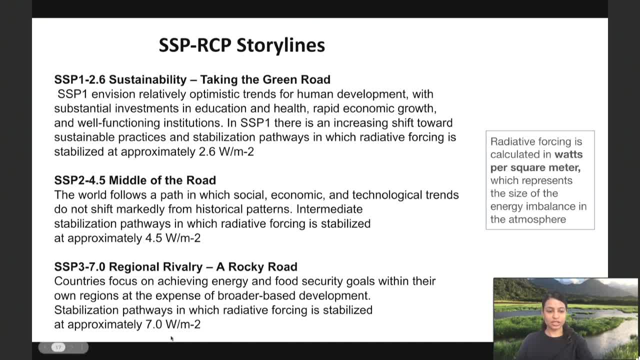 stabilization pathway in which the radiative forcing is stabilized at approximately 4.5.. So, and in a medium emission scenario, And the high is the 3.7.0, and the low is the 27.бо feet, which is the regional driver near the Rocky Road where countries focus. 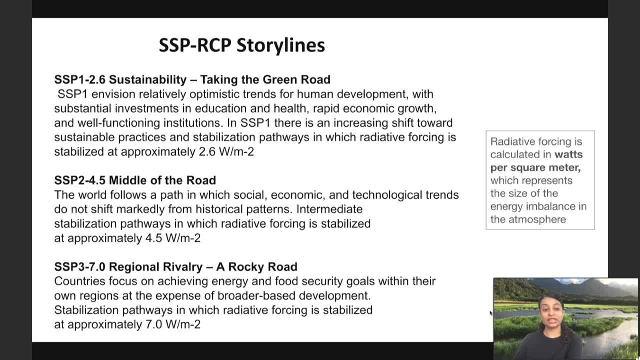 thin, achieving energy and food security goals within their own regions at the expense of broader based development. And so this is just showing a pathway that a world can take, and depending on what pathway we take, our global warming temperature is tied to it. This is just showing the climate projections by global warming level. Everyone is familiar with health parameters, So better air strength. 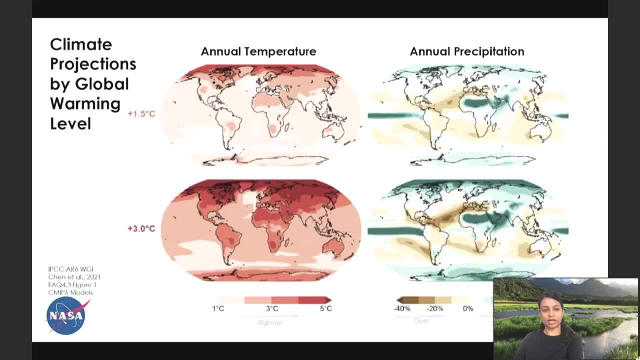 This is just showing the climate projections by global warming level. On the left we see annual temperature and on the right we see annual precipitation. The first row shows 1.5 degrees C's of warming and the one below shows 3.5 degrees C's of warming- global warming. 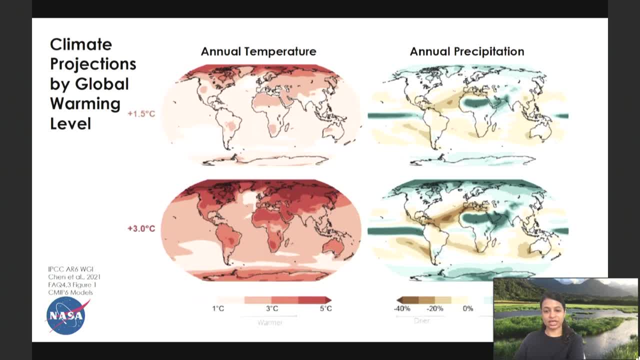 In each scenario we see that there are some regional patterns. You can say the dry regions get drier, wet regions get wetter on the annual precipitation map but definitely we see that it's not consistent globally. Some regions are definitely feeling the impact more than others. 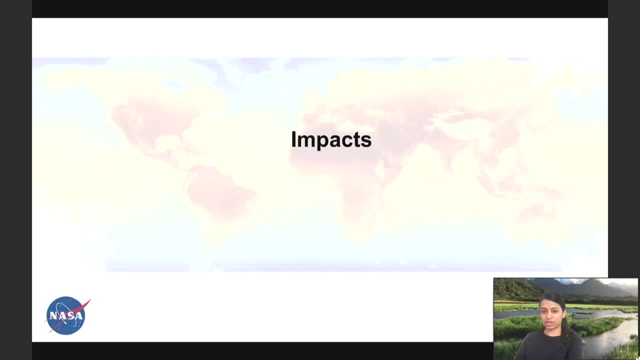 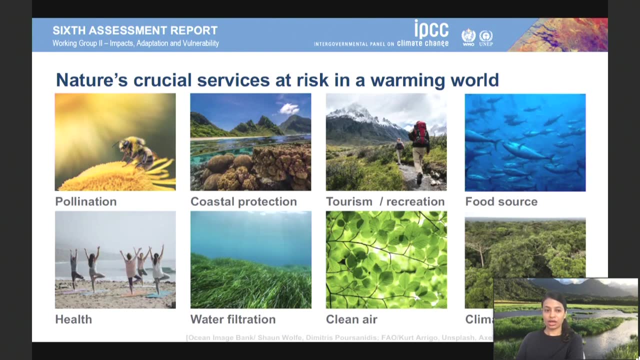 Let's get to the impact section. Impacts are noticed across many systems, Nature's crucial services at risk in warming world. you have pollination, coastal protection, tourism, food source, health, water filtration, clean air. These are just some of the sectors that will see impact, but we also see increases in things like wildfires that are being studied on the western United States. 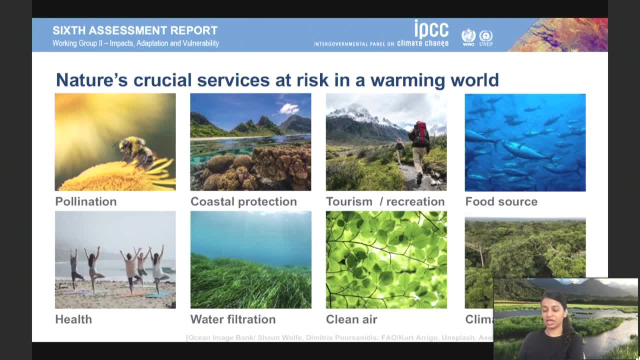 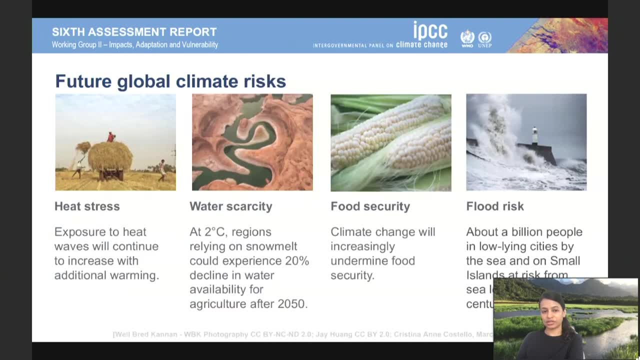 Impacts on transportation systems in urban areas, for example, due to increasing hurricanes. These are other future global climate risks. You have heat stress, water scarcity, food security and flood risk. We know that exposure to heat waves will continue to increase with additional warming and this has direct impact on health. 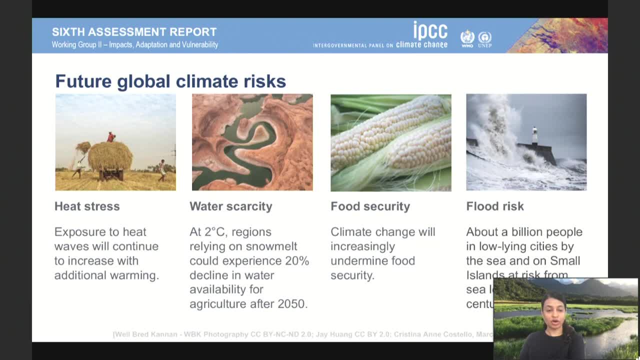 We know that at 2.3 degrees C warming regions relying on heat waves will increase with additional warming and this has direct impact on health. snowmelt could experience 20 percent decline in water availability for agriculture after 2050.. California and the western United States have been experiencing the worst droughts. 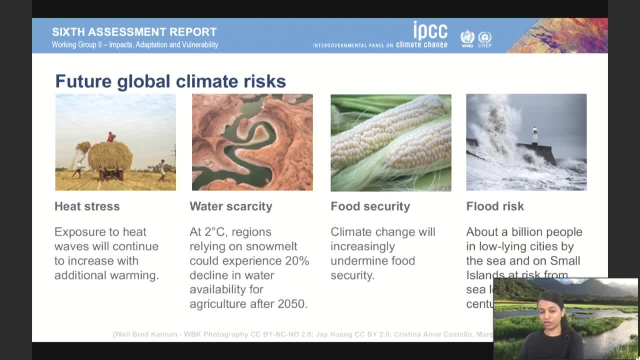 in the history in the past few years, Though we know the droughts are getting worse and it directly impacts our food systems and agriculture, So we know that climate change will increasingly undermine food security in already vulnerable countries and regions in the world. Flood. 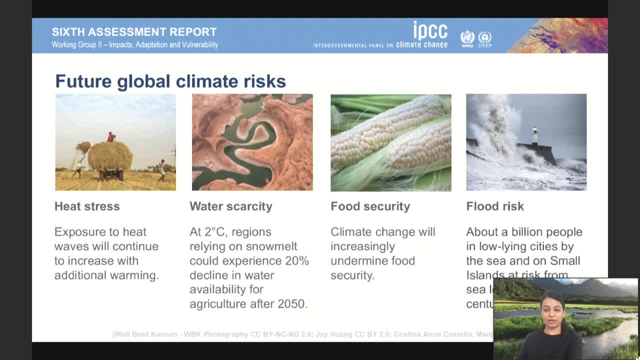 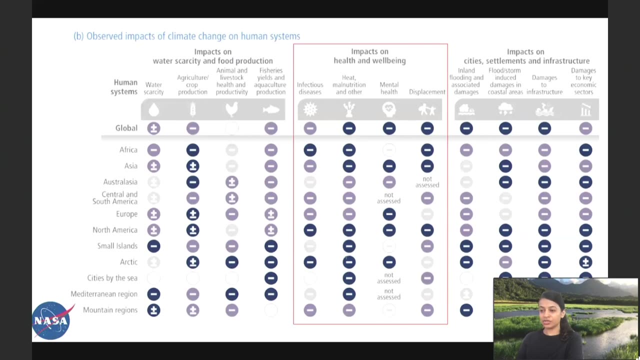 risks. about a billion people in low-lying cities by the sea and on a small island are at risk from sea level rise, but also extreme events like hurricanes and cyclones. Here I wanted to focus on the impacts on health, and this is a chart from the 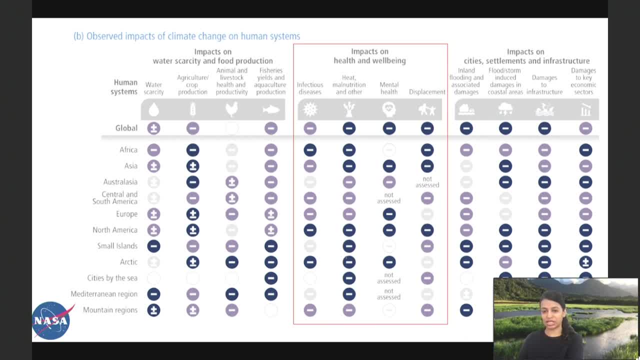 recent information that was published by the New York Times. It is a chart from the recent recent IPCC report that I mentioned before, which is AR6, released a few weeks ago. This shows the impacts on health and well-being by region, the dark blue being high- negative. 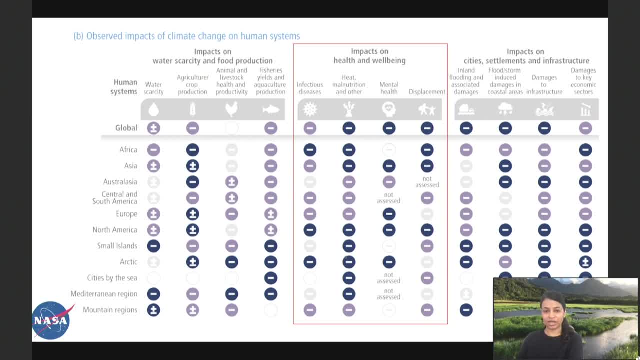 impact And we can see here for Africa you have high negative impact on infectious diseases And we've seen through studies that there are higher cases in malaria that have been noticed due to change in rainfall patterns and spatially and temporally We are seeing 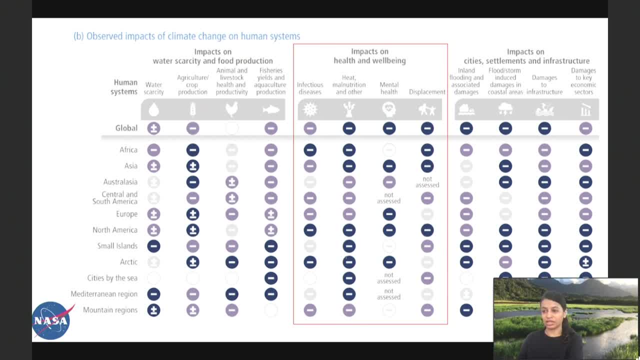 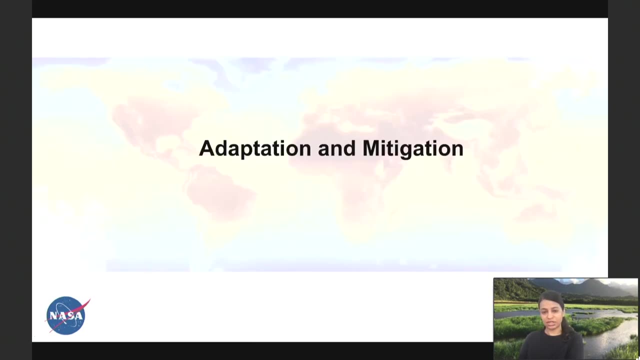 the adverse impacts of high heat and humidity on health. in the United States already, We are also seeing displacement due to floods and hurricane, which is projected to only increase in the future. Adaptation and mitigation- and what does that mean? But before that, 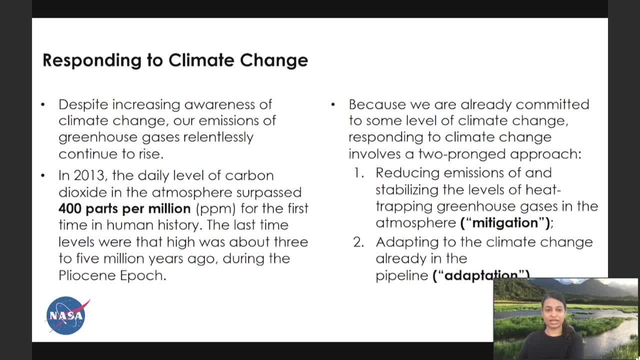 let me just say that, despite increasing our awareness of climate change, our emissions of greenhouse gases relentlessly continue to rise, And so our response to climate change needs to have a two-pronged approach, which is reducing emissions and stabilizing the levels of heat-trapping greenhouse gases. 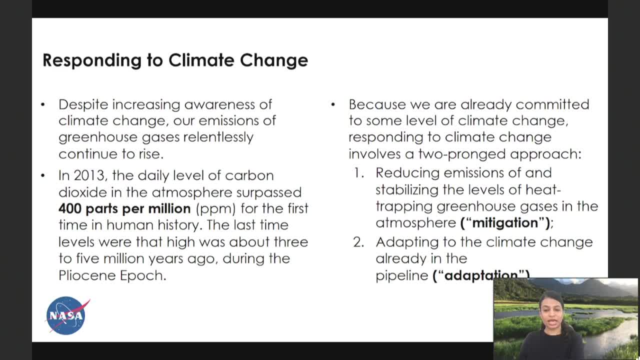 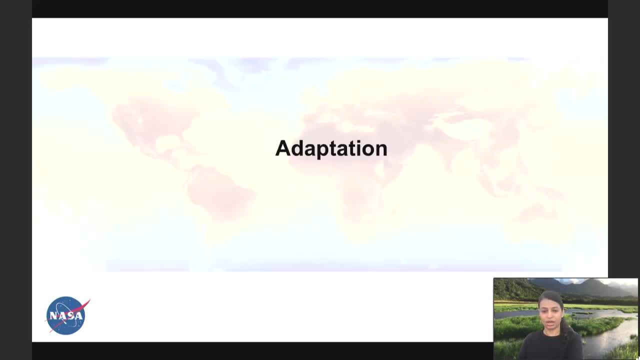 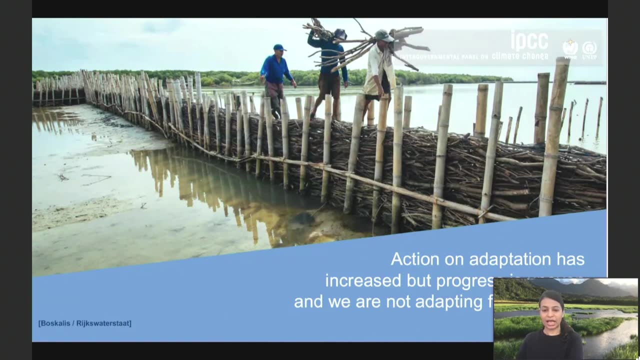 In the climate change field. we call it mitigation, And the second is adapting to the climate change, which we call adaptation. So let's look at adaptation. Action on adaptation has increased, but progress is uneven and we are not adapting fast enough. This is according to the new IPCC report released. 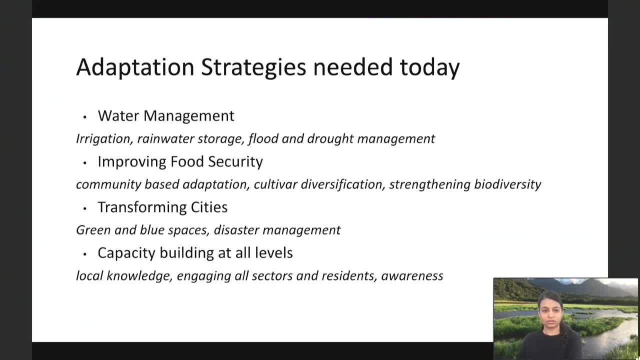 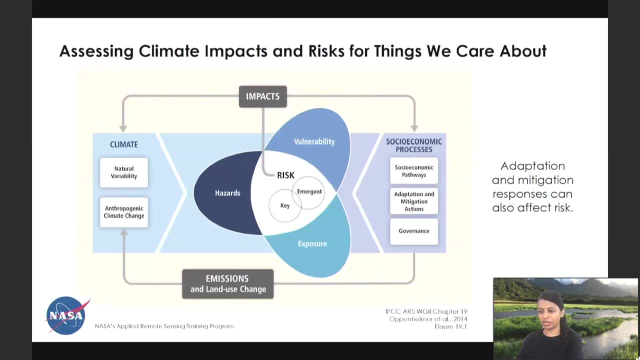 a few weeks ago. Hold on, I think I missed this. I'm sorry. I'm going to go back to the slide, because this is important Before we get into adaptation. Syedna Bikaner and mitigation. I wanted to talk about what is risk and how do we explain climate risk. 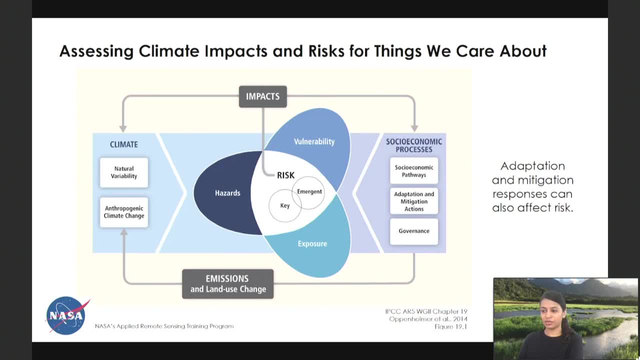 or assess climate risk. It's the intersection of hazard, which is climate hazard in our case- vulnerability and exposure. For example, a climate hazard like drought. the risk that a farm can face will depend on its vulnerability, how it was designed. the economic system. 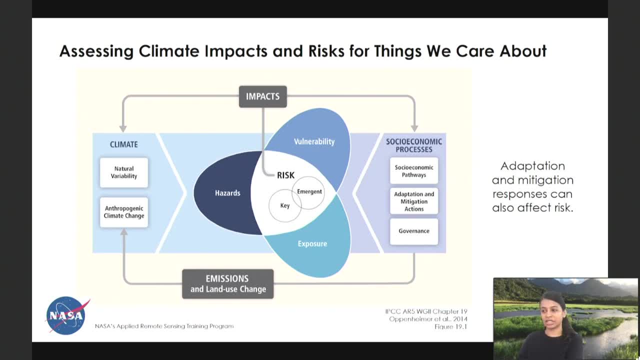 the initial conditions that contribute to its exposure or where it is. And what's important to note is that we have, on the other hand, socioeconomic processes that feed into risk, like socioeconomic pathways, the adaptation actions and mitigation actions, and the existing governance structure. How do we assess risk? We usually follow a framework for a climate. 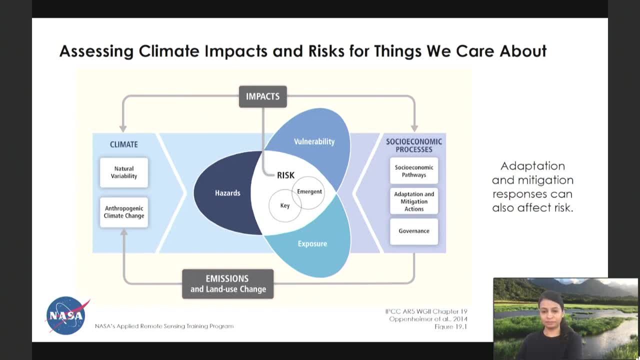 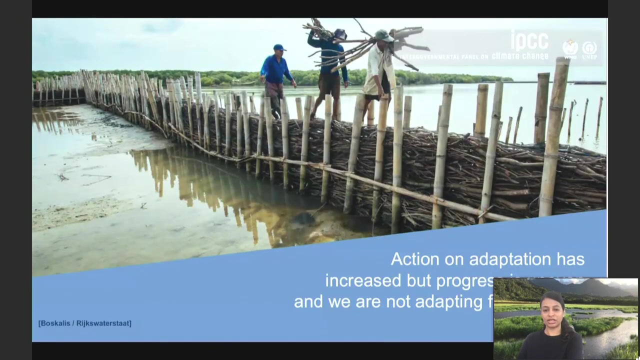 risk situation. We represent the current system that we're studying, we represent the current climate of that system and then we represent future climate changes, project future climate and then project future climate impacts to the set system, then identify and test adaptation and risk management solutions. Okay, now let's get into adaptation. These are some. 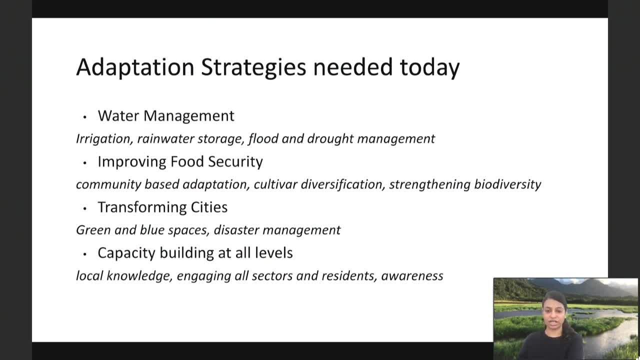 of the strategies that are needed today. Okay, now let's get into adaptation. These are some of the strategies that are needed today And are identified by this IPCC report. Again, these are some strategies. that are many more. We have water management, which includes irrigation, rainwater storage, flood and drought. 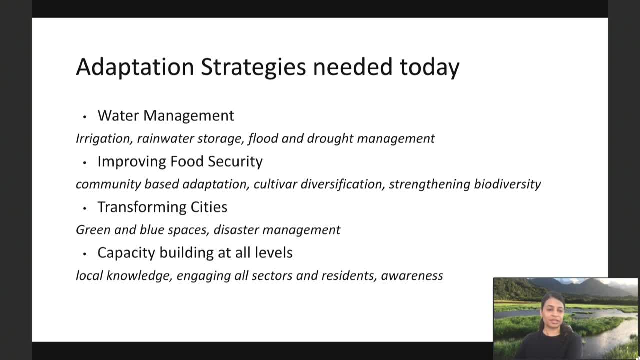 management. improving food security, such as community-based adaptation. strengthening biodiversity. cultivar diversification, which is really important for the ecosystems and the diversity of soil. Transforming cities, which is green and blue spaces. disaster management programs. capacity building at all levels, which means local knowledge, engaging all sectors and residents. 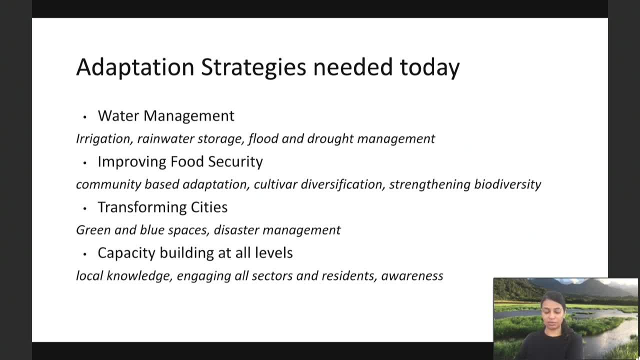 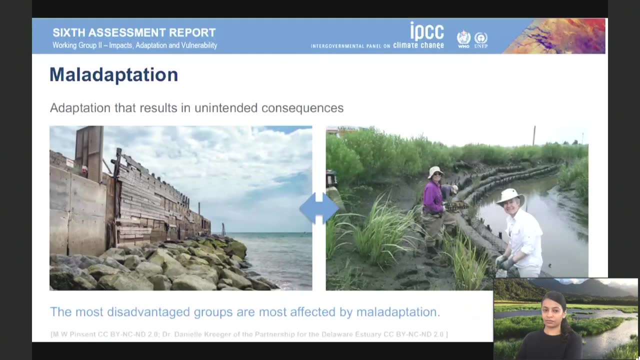 and creating awareness. And this is where I wanted to talk about the bottom-up approach and include community in planning decisions and in creating solutions to really understand the local conditions. Maladaptation. So maladaptation is when a climate change adaptation action backfires. 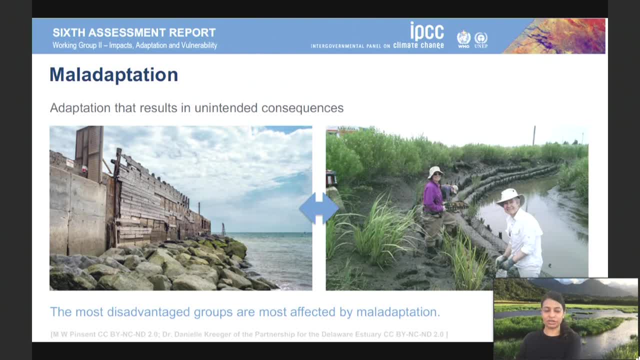 and have opposite of the intended effect, or which means it increases vulnerability or reinforces existing inequality. For example, solutions around, say, agricultural modernization offered to only those who own the land versus those who work on the land, can reinforce and enforce existing inequality and, in turn, increase vulnerability of the already vulnerable. 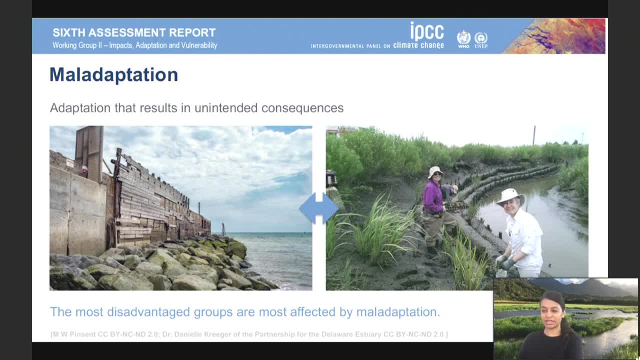 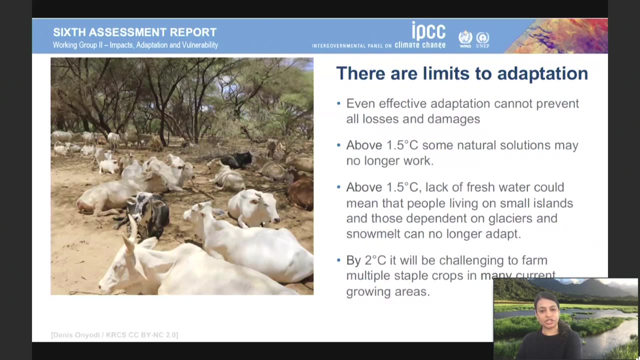 populations. Studies show that if you don't address systemic inequalities when you're designing adaptation solutions, it can lead to division, conflict and maladaptation and have unintended consequences. So there are limits of affair patients, of course, even an effective adaptation. cannot prevent all losses and damages. It's not just for the well-being of the population. It's like if you have an effort, you can both lead the way for the success of the business. So if you are having an effort and you have an effort, and you can see the benefit of it. 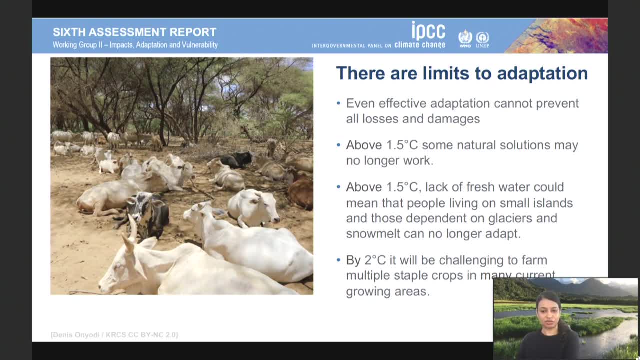 damages Above 1.5 degrees C of warming. some natural solutions may no longer work because your Earth system has already changed Above 1.5 degrees C. lack of fresh water could mean that people living on small islands and those dependent on glaciers and snow melt can. 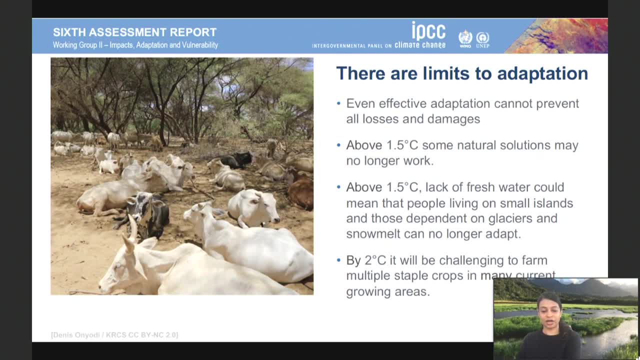 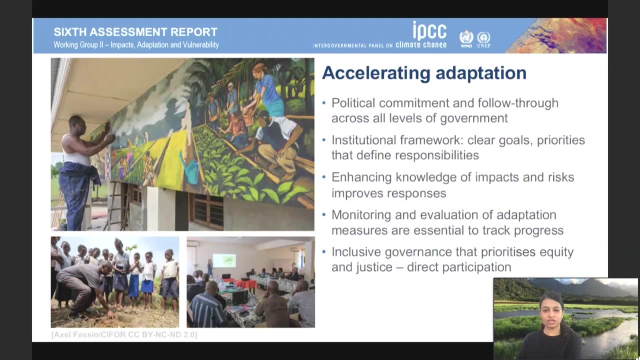 no longer adapt because of just not having access By 2 degrees C warming. it will be challenging to farm multiple staple crops in many current growing areas due to high heat. So accelerating adaptation. what does that mean? We need political commitment and follow through across all levels of government institutional framework, enhancing knowledge. 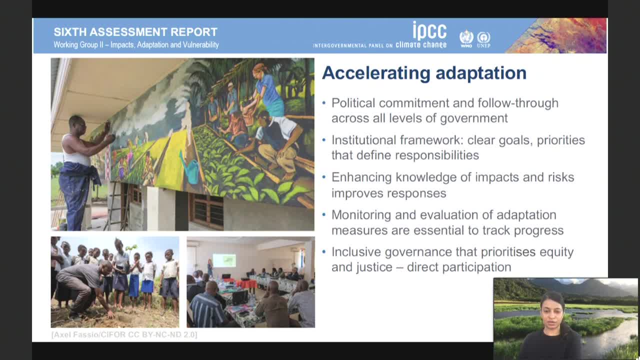 of impacts and risk. And that can start with this right, with creating awareness of climate change basics, understanding impacts, understanding risks, monitoring and evaluating of adaptation measures, and to track progress to make sure that you're not maladapting to. 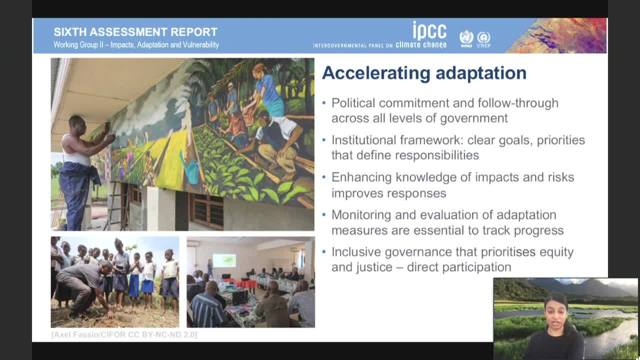 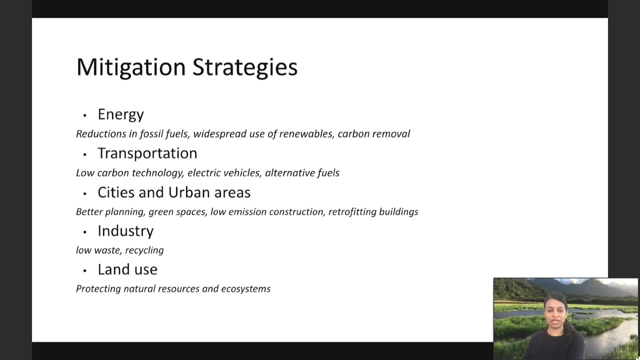 make sure that the solutions that you've offered are actually working. And again, inclusive governance that prioritizes equity and justice. So what is mitigation? Some mitigation strategies and again some. there are many- include energy, which is direct reductions in fossil fuels. 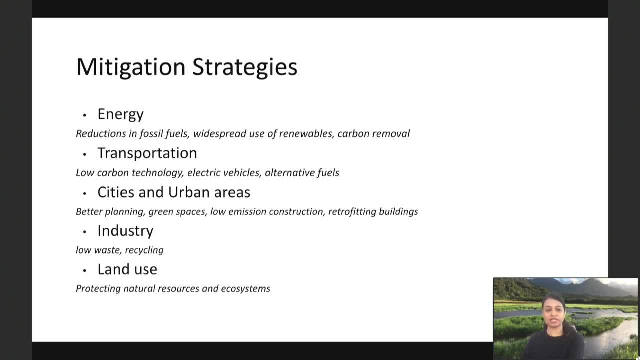 widespread use of renewables, reducing greenhouse gas emissions in transportation, which can mean low carbon technology, electric vehicles using alternative fuels In cities and urban areas. it can mean better planning green spaces, low emission construction, retrofitting buildings In industries and other industries. it can mean creating low waste and recycling. 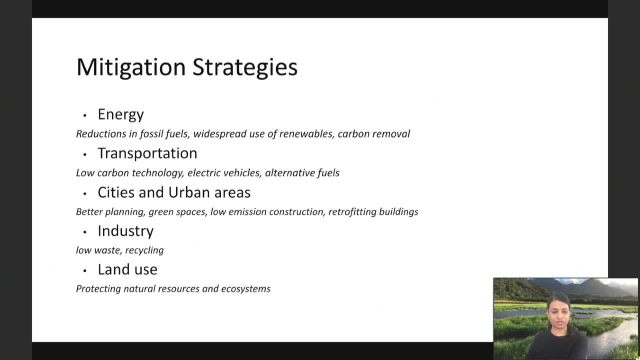 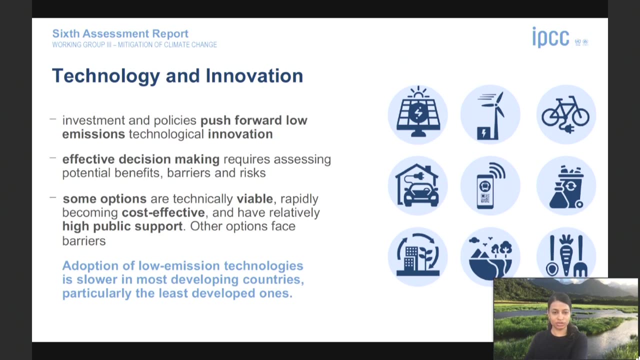 And in land use. it can mean protecting natural resources and ecosystems, which is important in nature-based solutions when looking at both adaptation and mitigation. So technology and innovation: it's important to invest in new technology, push forward low emission technology, invest in carbon removal technologies. 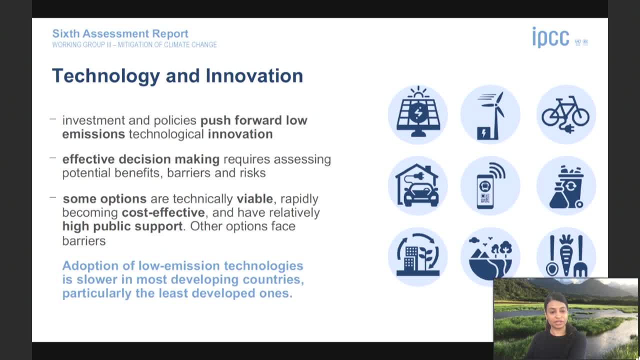 Some options are technically viable and rapidly cost effective. There are a number of options, But I think it's really important here to note that adoption of low emission technologies is slower in most developing countries, particularly the least developed ones, And lack of resources. 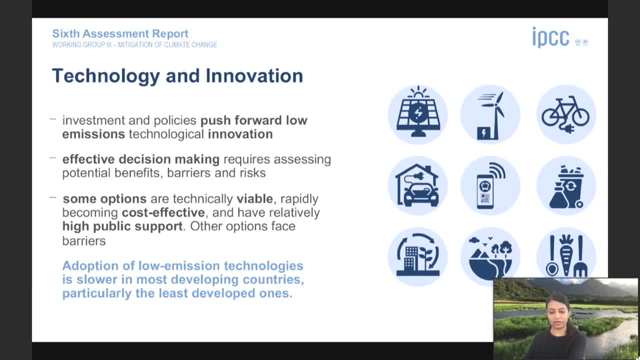 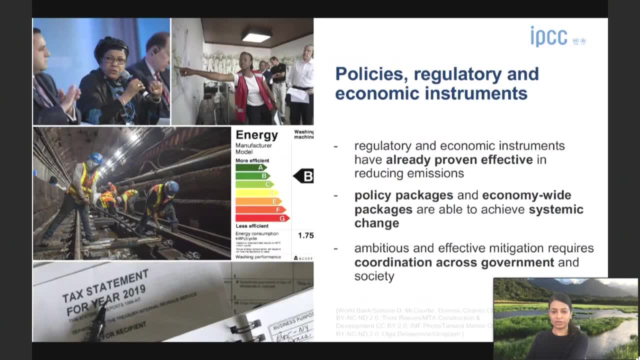 funding and financial viability is really important here for all regions across the world. Policies, regulatory and economic instruments have already proven effective in reducing emissions, but there are potential solutions that can make a difference to health care and climate well-being in the future. It is really really important for coordination across governments and society to have ambitious 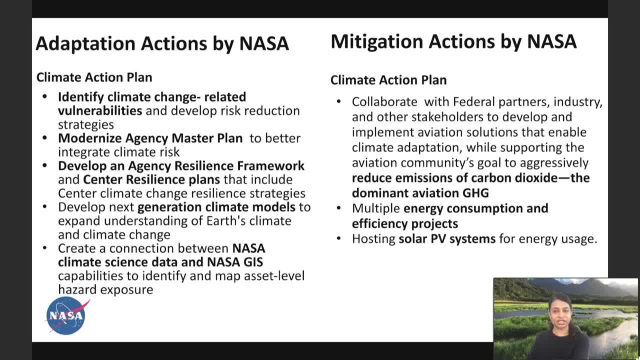 and effective mitigation strategies. Here are some of the adaptation actions and mitigation actions by NASA. in our climate action plan, We identify climate change-related vulnerabilities and we develop what is called a risk reduction strategy. We are planning on modernizing our master plan to better integrate and update our energy. 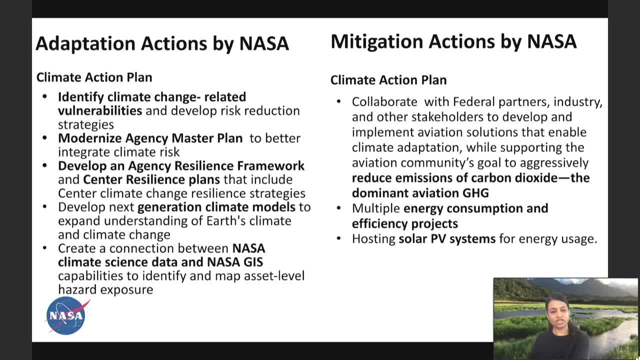 adapt to climate risk. We are developing agency-wide resilience framework and center resilience plans that include resilience strategies, develop next-generation climate models, which is the NASA GIS model that I talked about, And just to expand understanding of Earth's climate system. we're trying to create a connection between the climate science data and the GIS. 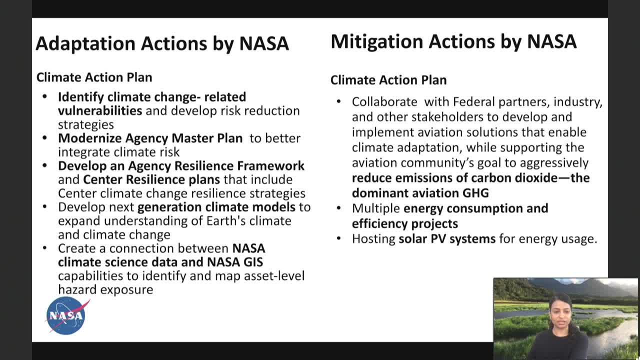 capabilities to identify and map asset-level hazard exposure. On the mitigation side, the goal is to aggressively reduce emissions- the dominant aviation emission here, which is the GHG- By looking into alternative fuel technology. we are also looking in multiple energy consumption and efficiency projects hosting solar PVs for energy usage, et cetera. 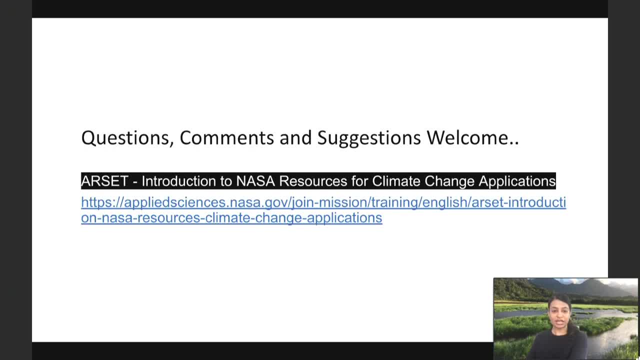 And that's it. That's my last slide. Any questions and comments are welcome. This is a link to an entire training for climate change basics and also includes remote sensing data. If folks are interested, please go and take the training And back to Christina. 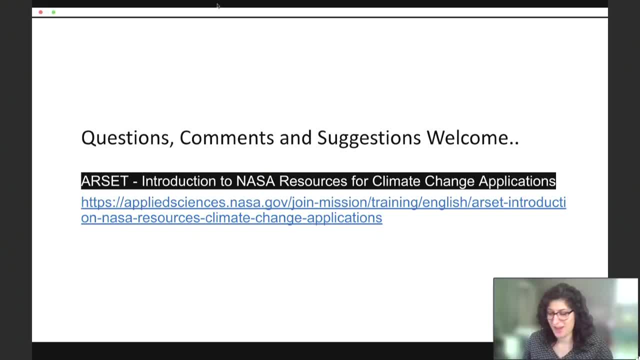 Christina Wodtke. Thank you so much. That was a super interesting presentation and even for some of us who have kind of been in the corner, I think it's going to be a really interesting presentation And I think it's going to be a really interesting 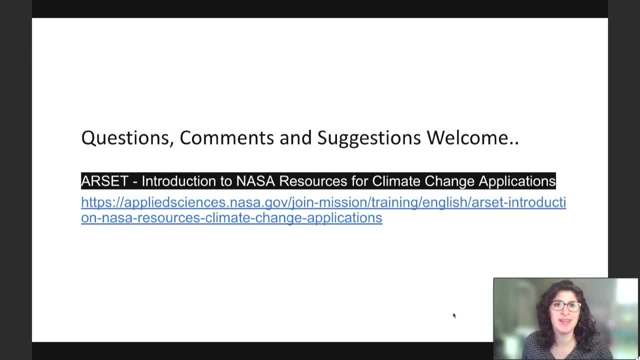 presentation and even for some of us who have kind of been in the corner, I think it's going to be a really interesting presentation and even for some of us who have kind of been in the climate world for a while, it's nice to kind of start from the beginning and hear the whole. 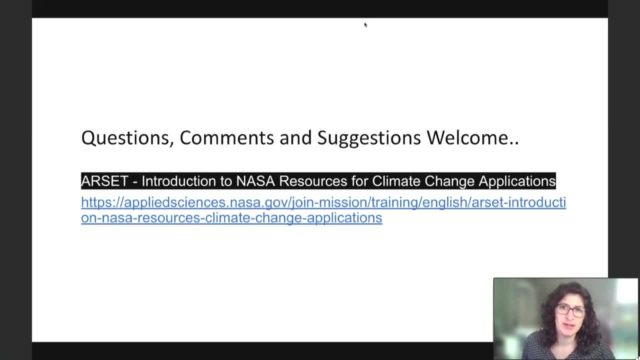 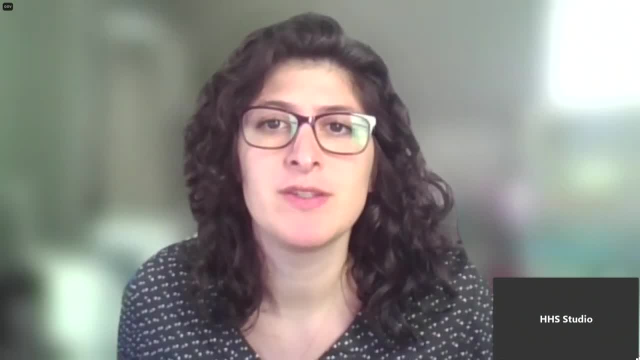 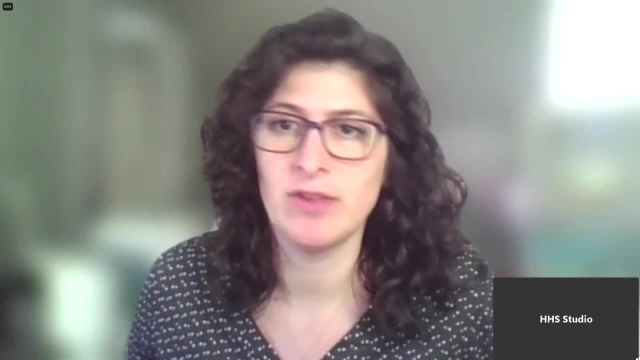 picture, So that was super helpful. We did get some questions. I do want to start here. So you mentioned a little bit of uncertainty and unpredictability. Are the models getting more accurate or less accurate because of the accelerating climate? unpredictability: 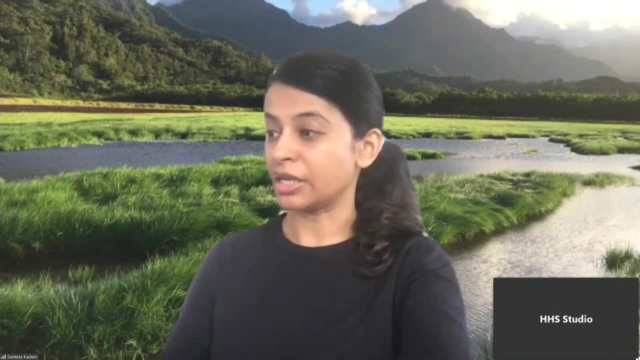 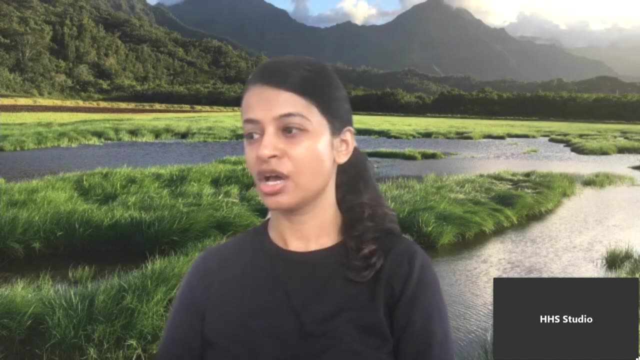 Christina Wodtke. So the models are definitely improving over time. The major source of unpredictability, I would say, is the greenhouse gas emissions enforcings. What we don't know is what the path the world will take in the future. We know the climate science, We know the 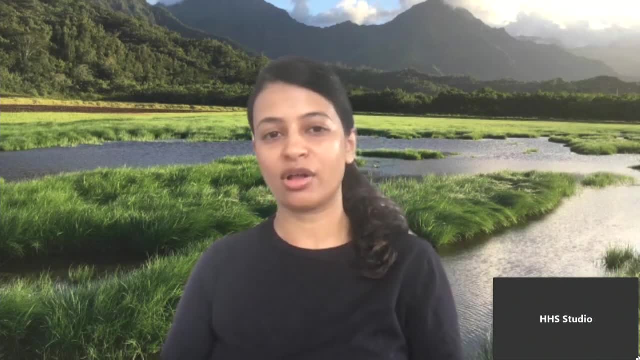 climate systems. We know the earth systems And even though they are always in flux, they're changing And it's the change that we've never seen before. The scientists are still very confident in modeling that The uncertainty really comes from the greenhouse gas emissions enforcings. 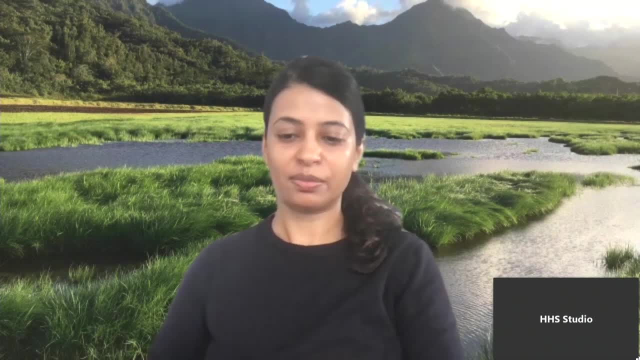 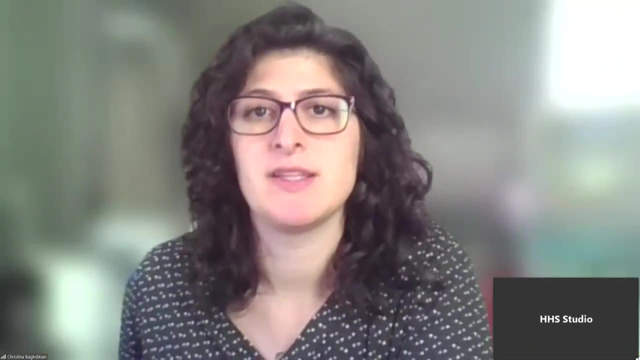 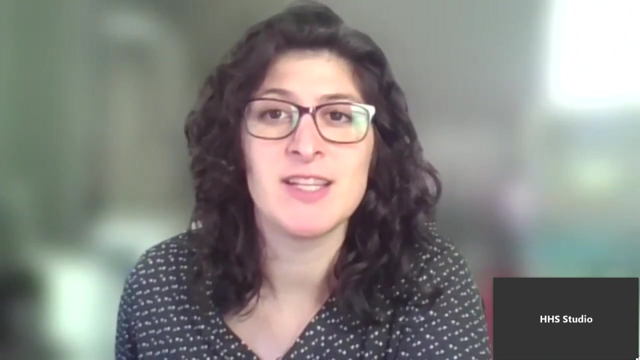 Christina Wodtke. So the models are definitely improving over time. The models are definitely improving over time. So I guess this is kind of a build on to that question. You were talking about the SSP And if you can remind us what the SSP is in your answer. I'm on the SSP storyline. 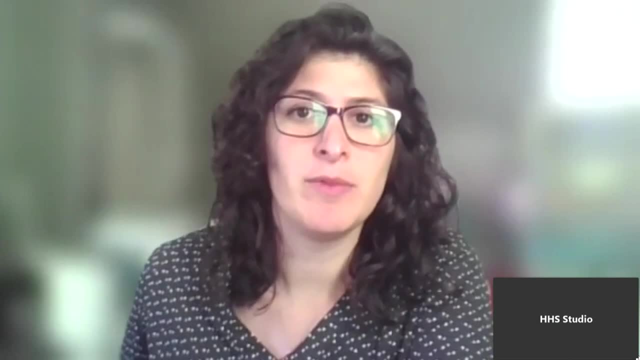 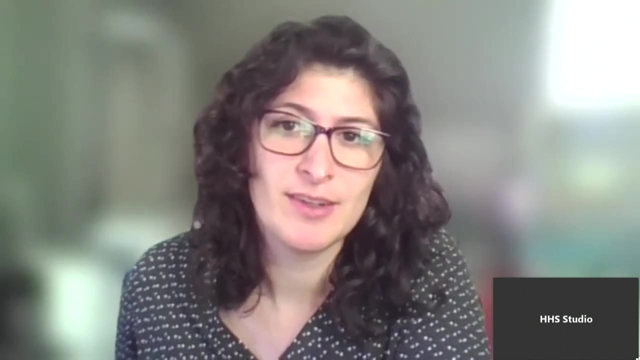 predictions. Are we currently on the taking the green road, the middle of the road or a rocky road? And then what can we do to improve to ensure that we do end up on the green road? Christina Wodtke Well. 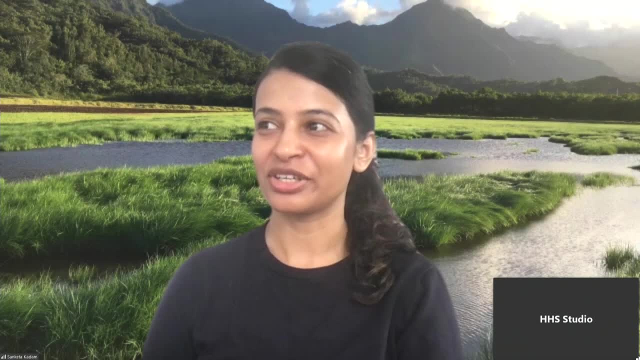 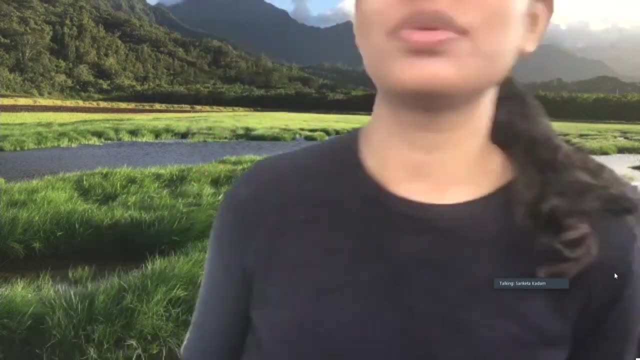 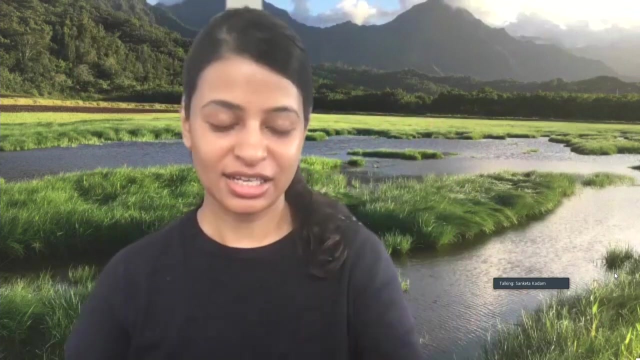 That's a loaded question, right. We really need to do a lot more to make sure we end up on the green road. We are currently- I wouldn't say we're- on the business as usual, which was the high SSP 58.5.. And let me just go back and say the SSP is the shared socioeconomic pathways. 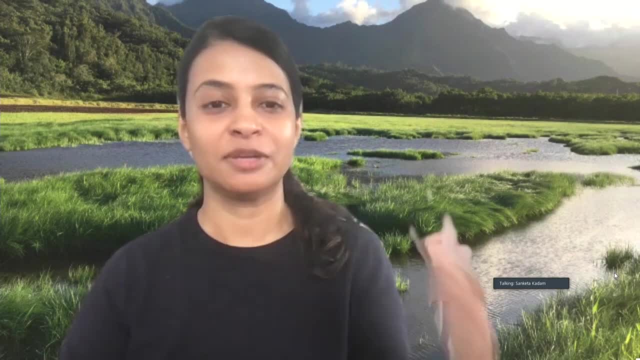 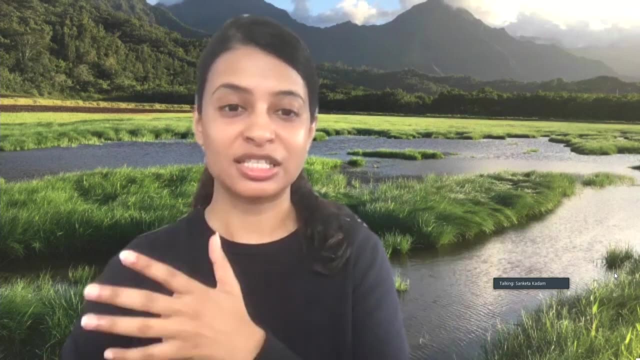 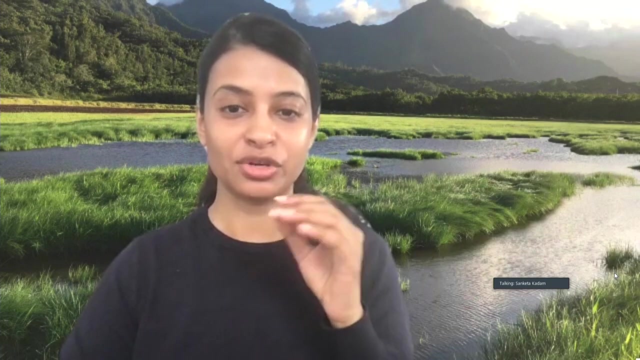 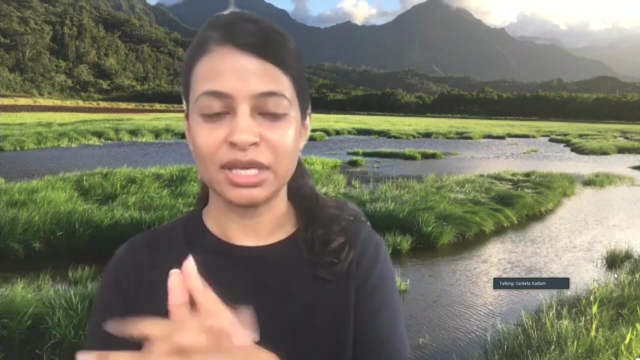 which include not only the development pathways that the world will take, but the definition itself includes the combined RCPs, which is the representative concentration pathways, which means that the greenhouse gas forcing- So it's a combined scenario with the development and the greenhouse gas forcing. I hope that makes sense And I would definitely say that we are not. 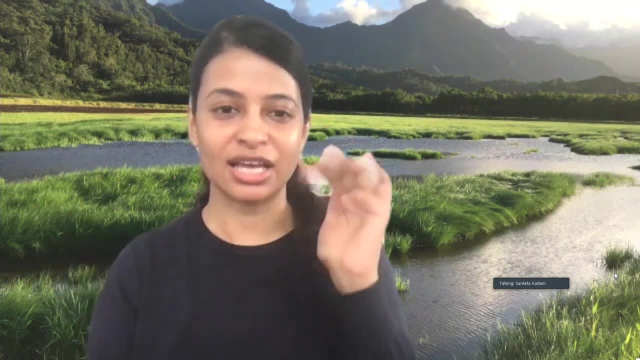 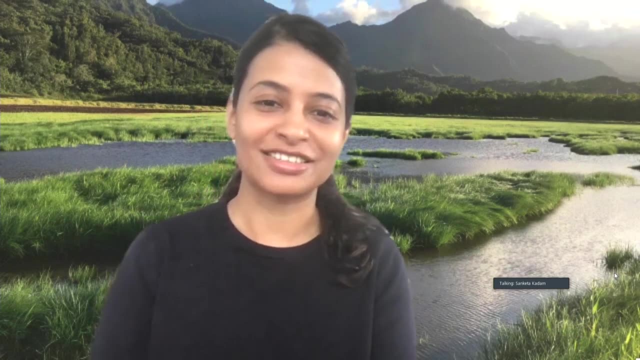 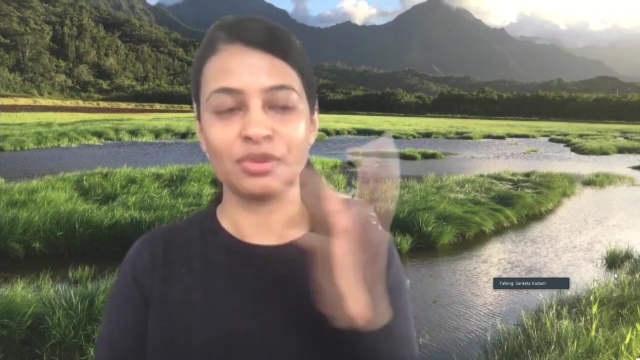 on the business as usual or the highest most scenario, which is, I don't know, it's a positive that we should look at, but according to scientists and the latest literature, to be on that high most scenario, we would have to basically reopen coal plants and reopen most of. 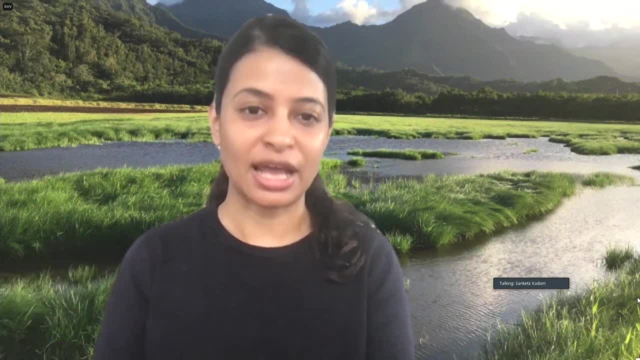 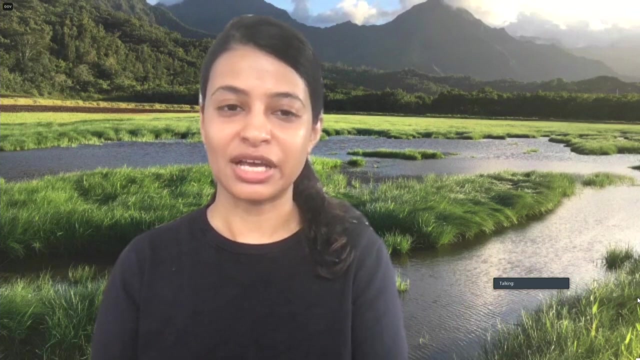 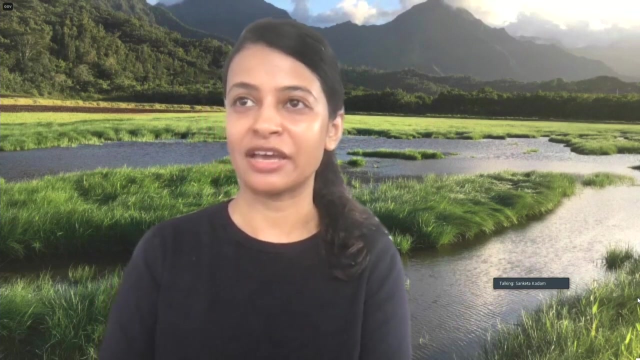 our closed fossil fuel plants, which is not happening. So we're definitely not on that road, but we are also not on the lowest taking the green road. So somewhere in between we need to really get together and make some really heavy changes to our systems. 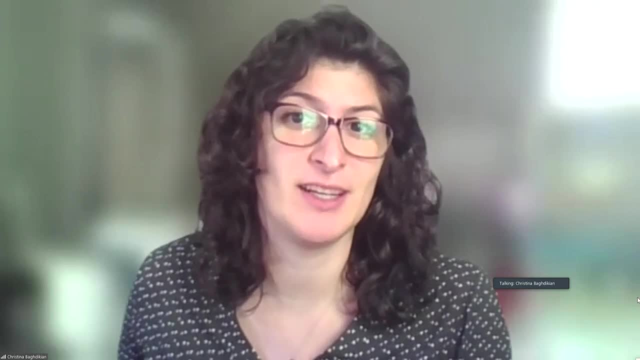 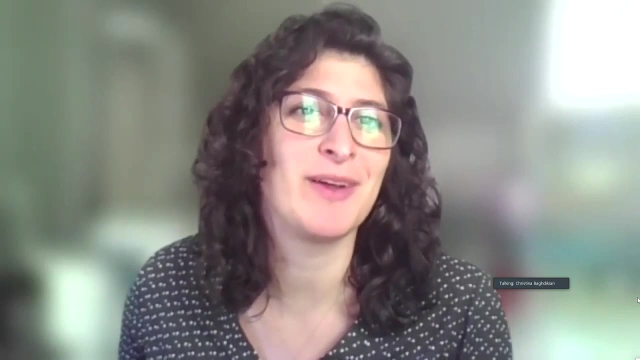 Thank you. We can't go backwards, but we must go forwards. it sounds like, And I think having these conversations are one of those ways and making sure folks know what we're talking about when we're talking about climate impacts and all these changes. So I appreciate you answering. 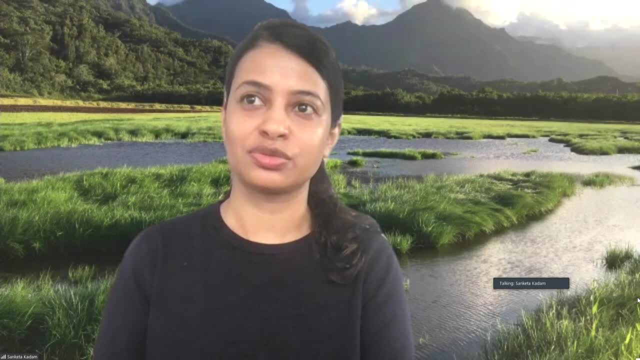 these questions. Yeah, I think that's what's more important. The most important is to just create as much awareness as you can, you know, and push climate literacy, And it's for us it seems like, oh, it's a basic concept, But if you don't make people 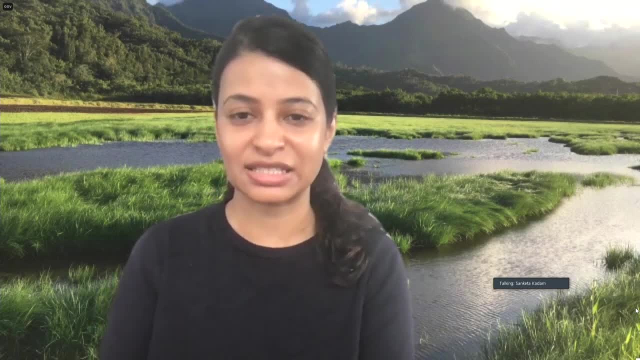 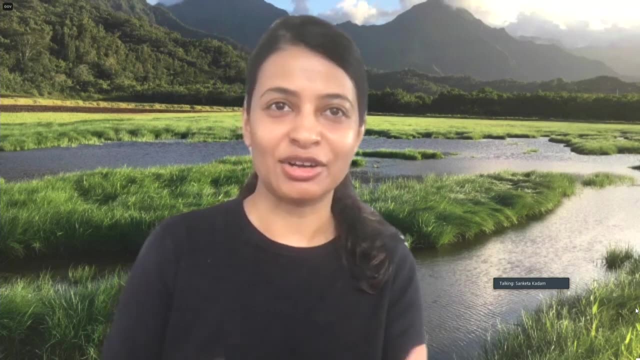 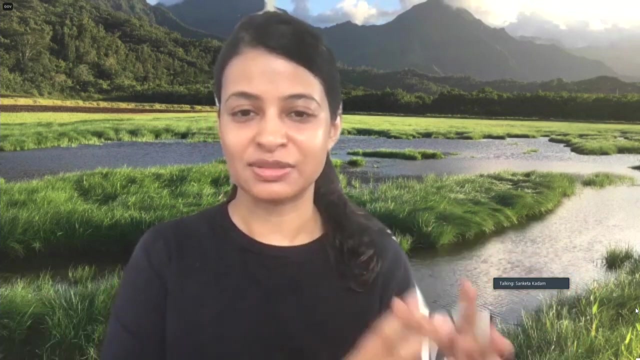 aware of what is actually happening to our system and the impacts that it can have? we don't really. sometimes, you know, I've seen people confuse recycling or air pollution with climate change And then just having that distinction of- okay, greenhouse gas emissions impacting the climate system or having those definitions of what's like weather. 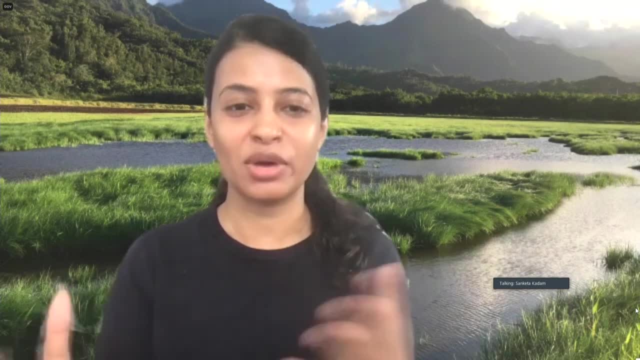 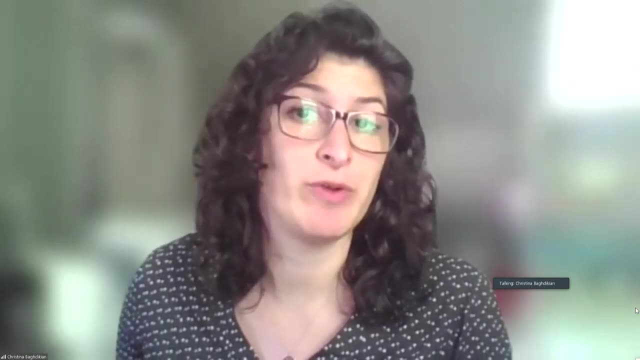 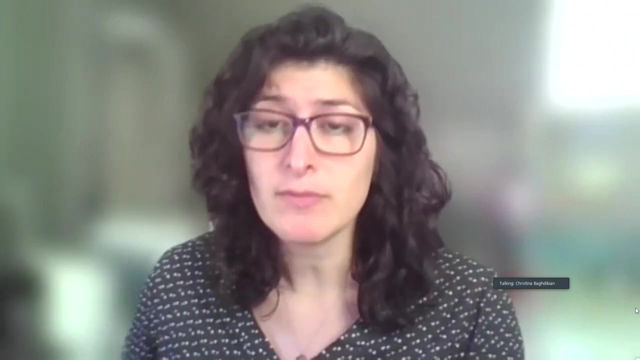 is different than climate, global warming is different than climate change. just knowing those basic things really help For sure, And I actually think folks including myself will be referencing your slides for some of those hazard risk exposure type information in the future. Speaking of those terms, another. 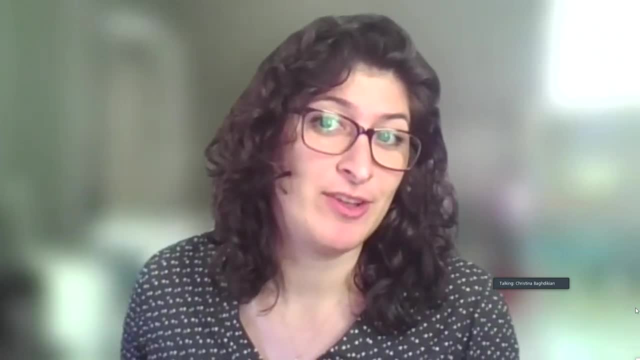 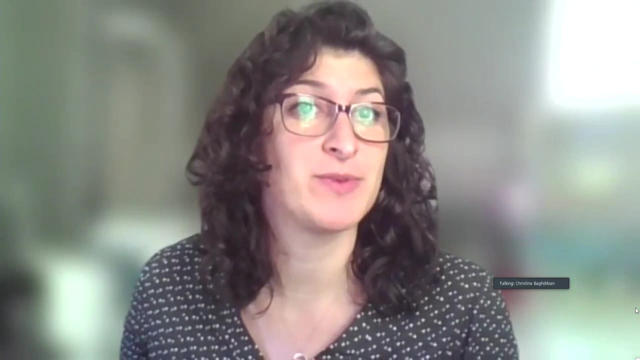 question that came in is: what is asset level hazard risk? Or I think you said what is asset level hazard exposure, Or hazard assessment? I think is what the phrase was. Oh, risk assessment, Is that what we're talking about? 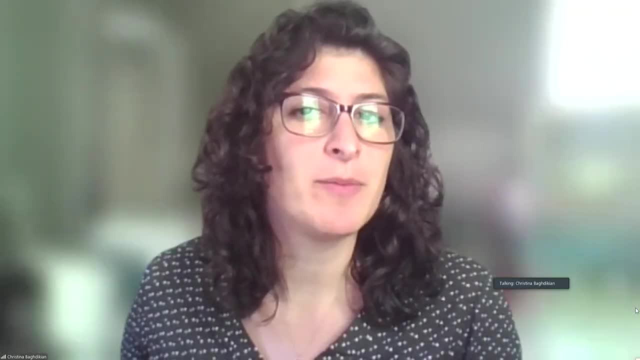 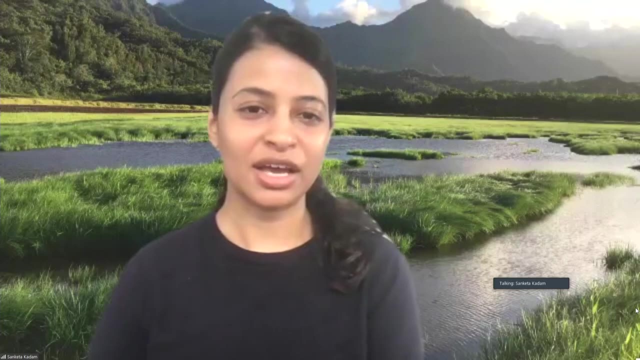 I think the question might be typed funny, but I think it was: what is asset level hazard assessment? Is that what you used in one of your later slides? Oh, I think yeah, when I was talking about NASA's plans. What we do is we look at what. 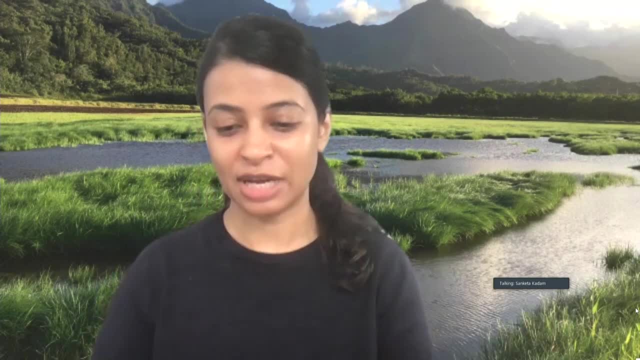 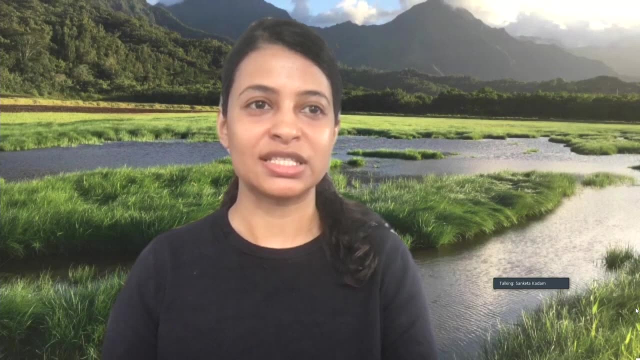 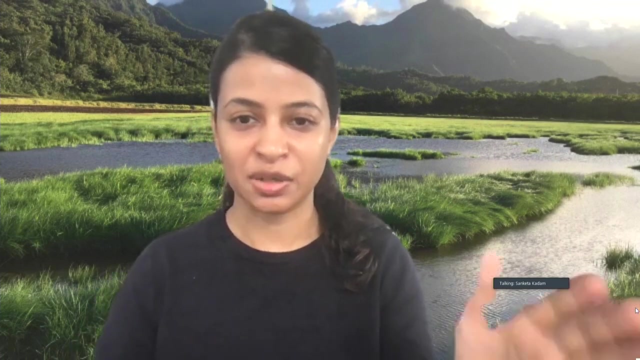 our physical assets are And we look at the assets, let's say, that are exposed to climate risk, So it can be things like buildings, or what is the extent of the equipment that the NASA facilities have, so operations and maintenance, but also equipment that are exposed to the climate. 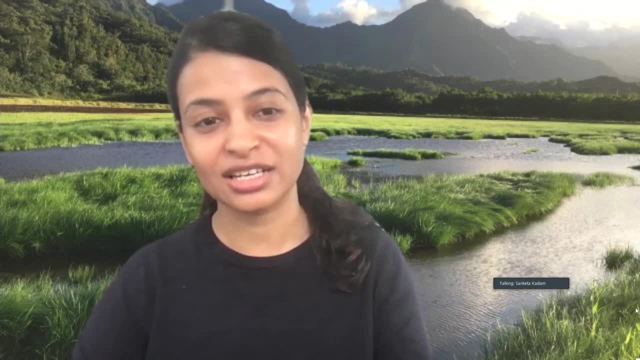 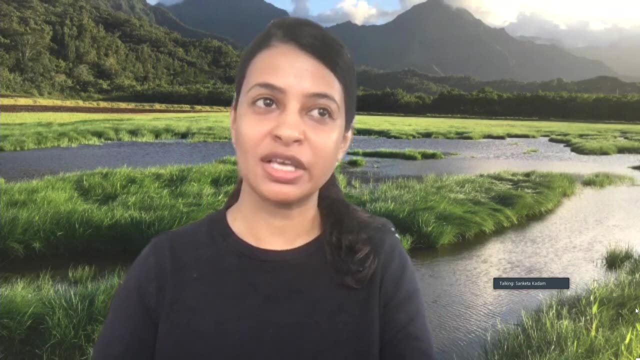 risk? I hope that was the question and I'm answering it correctly. I'm not really sure, But we also look at assets. When you talk about asset exposure, we also look at people- employees that come into our facilities to work in places like JPL and Ames when there's a wildfire. 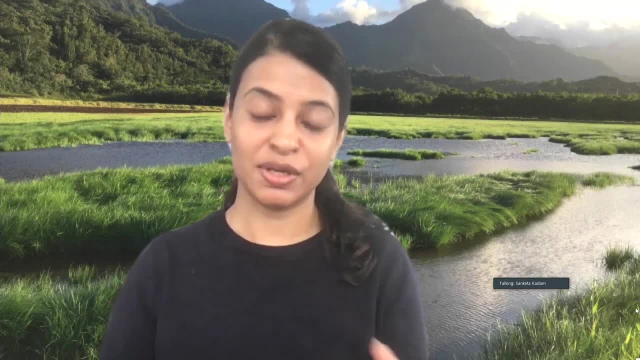 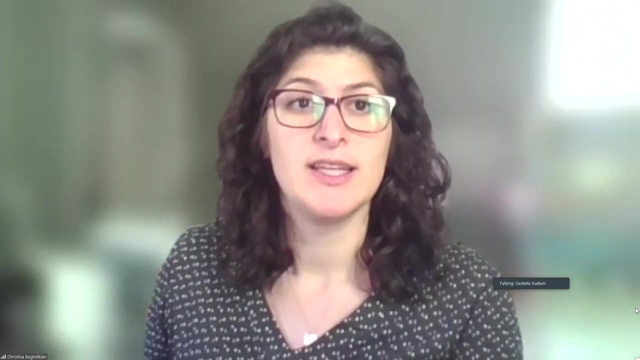 have intense air quality risks. So, even when they're working in a building, what is the exposure to bad air quality for the people working, but also for the buildings and the facilities and the equipment? I think that makes sense. Yeah, Yeah, I think that was the question And I think 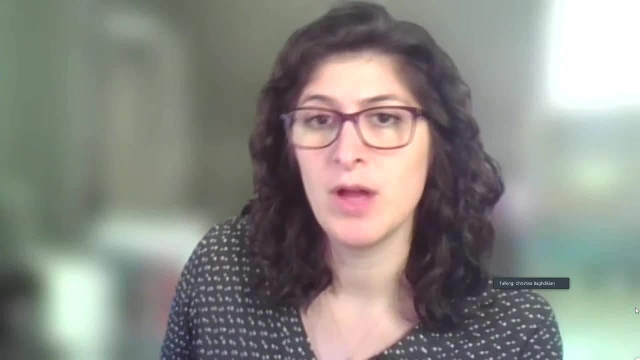 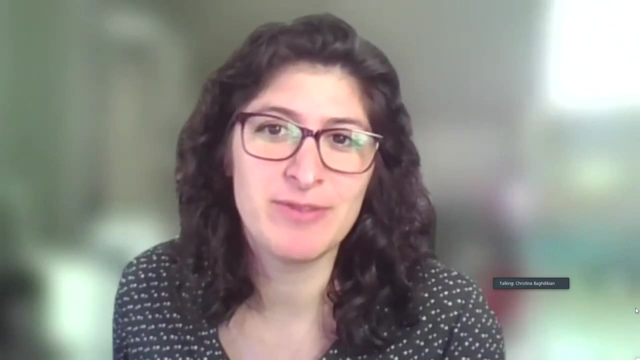 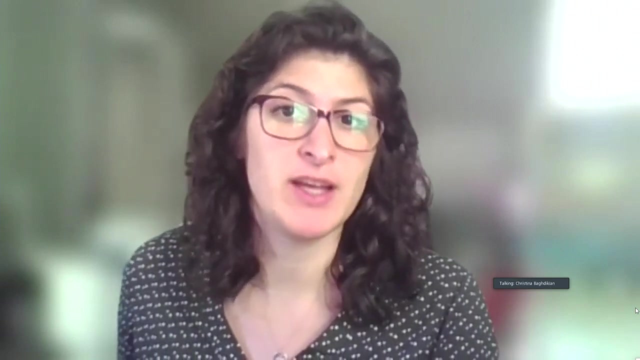 you've gotten to what an asset is, So that's that is helpful. Another question, if you're up for it: What is the timescale for downscaled GIS models are aiming to address? still at 30 years? They're asking because public health planning is having a hard time managing 10 year timescales. 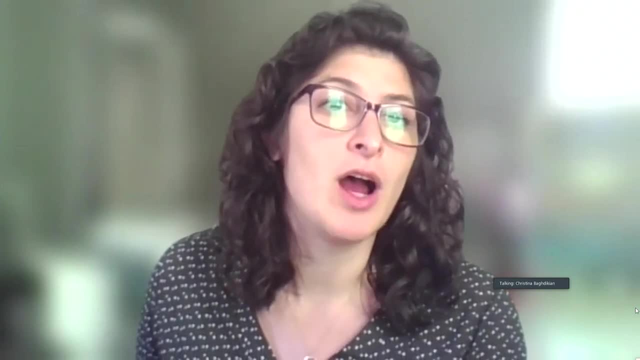 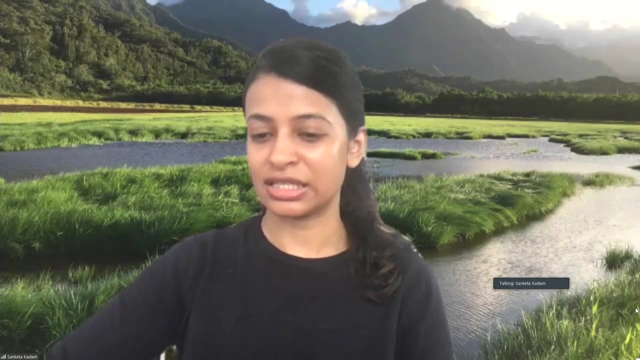 So is there progress in that direction that I guess, to have a shorter timescale models? So yeah, I mean I may not have explained this correctly in the slides And that's a good feedback point And I would change it in my slides to mention that models will actually 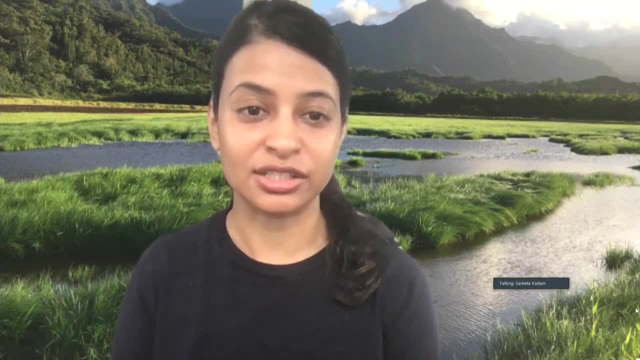 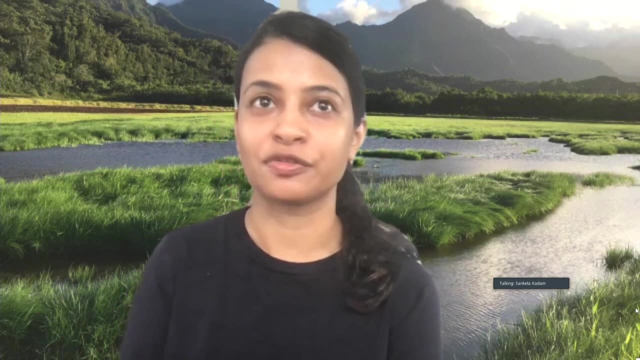 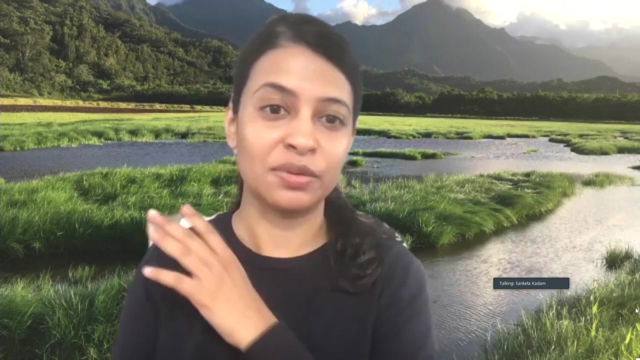 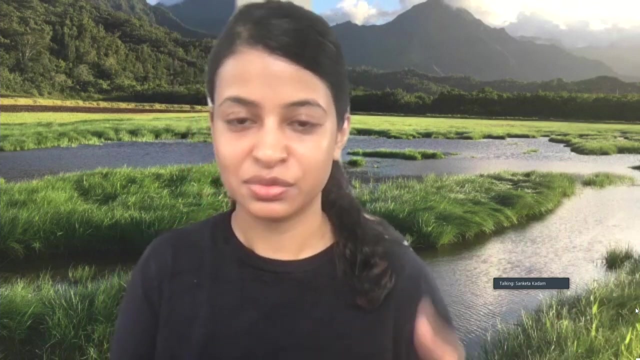 project on daily timescales. So, for example, if I'm looking at at the GIS climate model, I will have information which are daily outputs from 1950 to 2100.. So you can look at the next two years, five years, 10 years, whatever timescale that you work on. 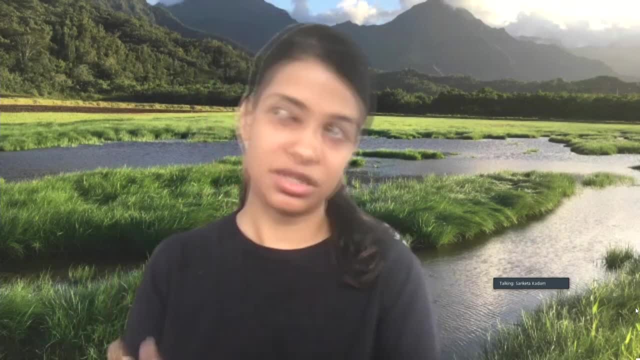 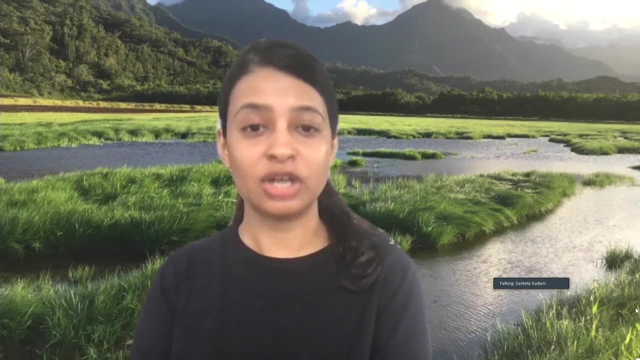 But the outputs are available daily at, I want to say, 27 kilometers. if you go to a regional model, that's the lowest you can go. But there are also for North America, lower resolutions- sorry, higher resolutions- available. you have five kilometers available as well. it's called a LOCA. 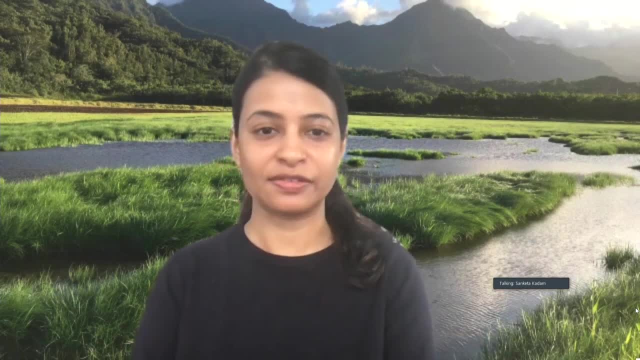 model And that's the lowest you can go. But there are also for North America, lower resolutions, higher resolutions available. you have five kilometers available as well. it's called a LOCA model, But it's from the older CMIP5 climate models, but they are available. So regional models go as. 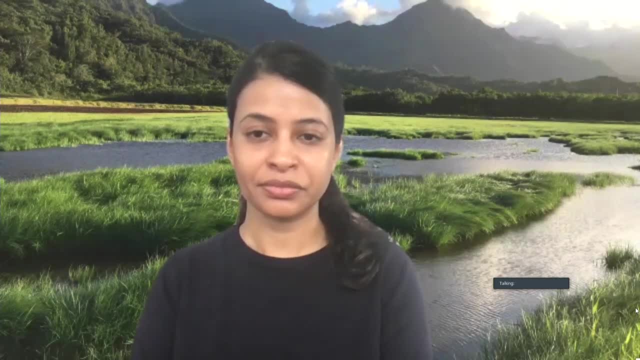 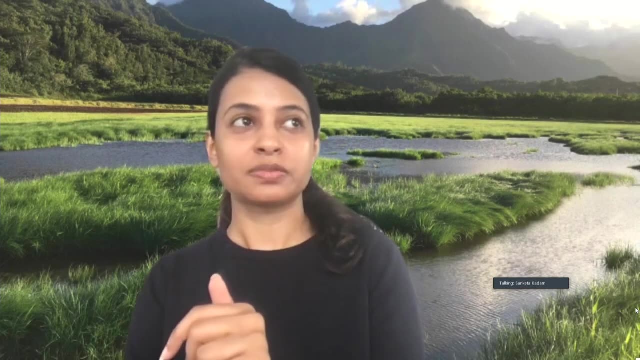 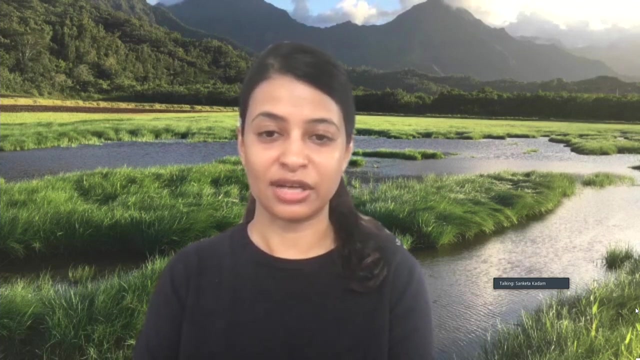 low as five to six kilometers also, But they are daily. So you can. you know, if you want to look at temperatures or say extreme heat days in the next year, you can, in the next five years, in the next 10 years, you can definitely do that. 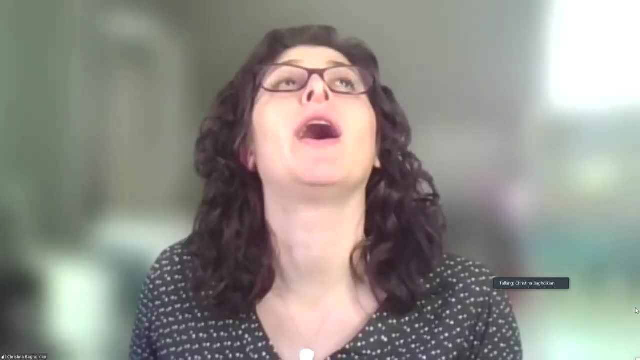 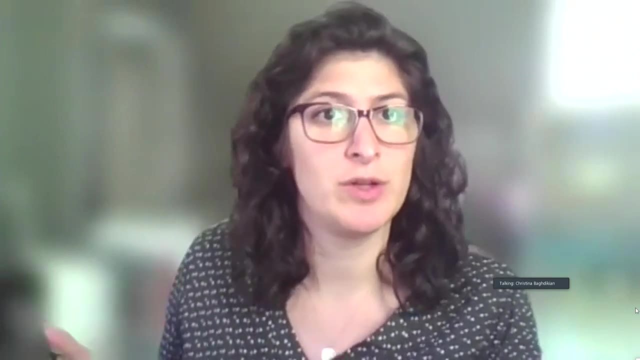 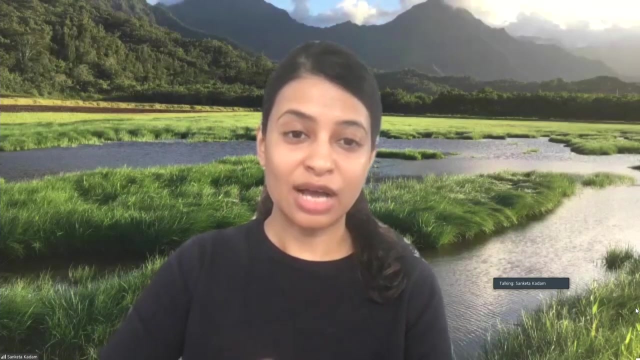 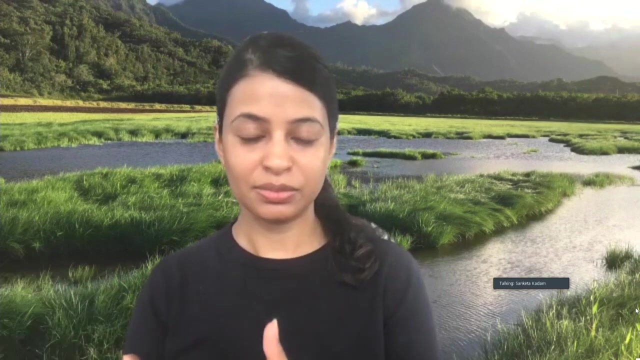 Jomana Musmar-. Okay, So would it be correct to say that the global models are on the longer timescales and then the smaller you get in scale, you can do a little bit quicker or shorter duration. shorter timescales- No. So the downscaled regional models are also from 1950 to 2100, same temporal resolution. 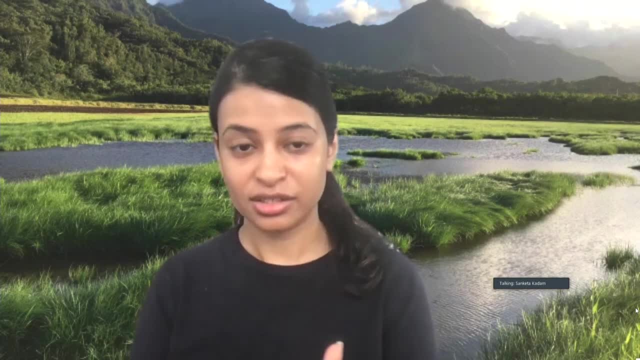 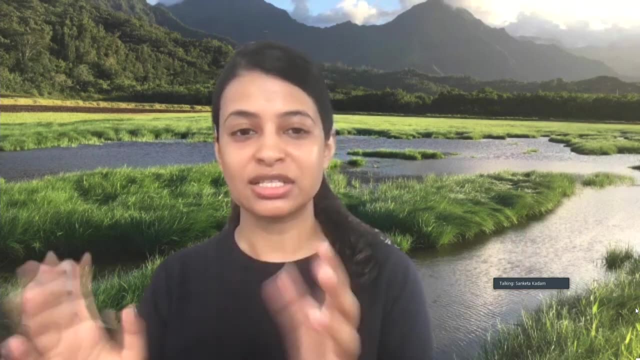 What's different is when you're forecasting weather, which is, say, if it's going to rain tomorrow. those are weather models, Those are not climate models. So there's a difference between the different types of models that you're using. Jomana Musmar- Thank you for clarifying. 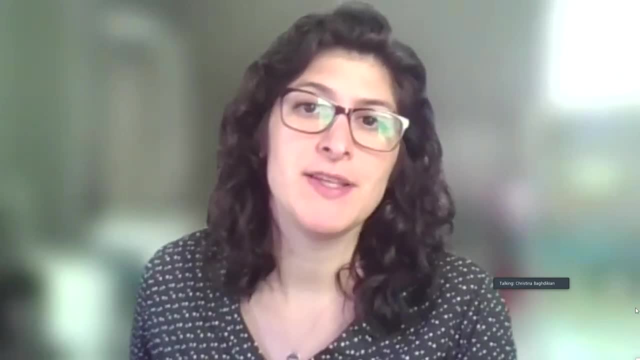 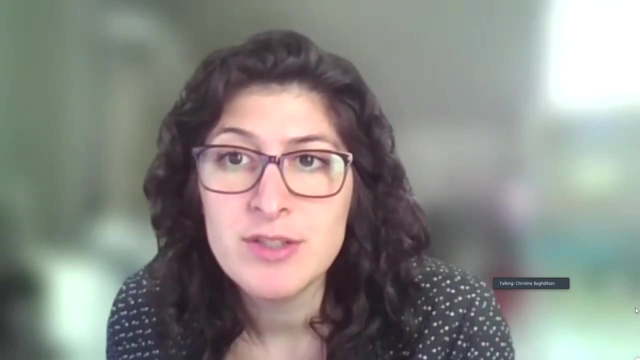 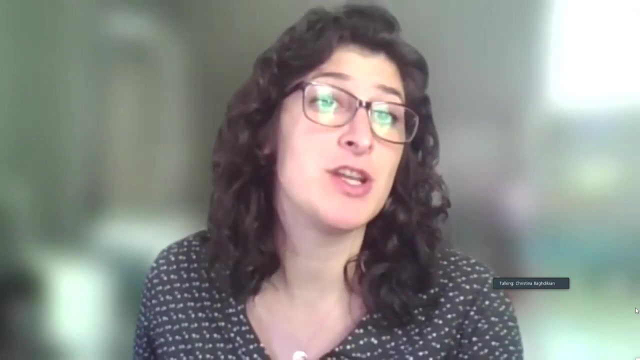 Okay. So another question: do we have opportunities to better engage with more diverse perspectives, for example Indigenous wisdom, in attention to the very helpful science and governance? So I guess is there a way to draw upon Indigenous wisdom and experience in water, then of or przez, And then if there's some work in this field where that can be olive-cleaning, to show that it won't have lower gradient shrimp. so there's a way to draw upon indigenous wisdom, experience and not only also may be Prop seller and impacts, but also Florist mod, meaningless. 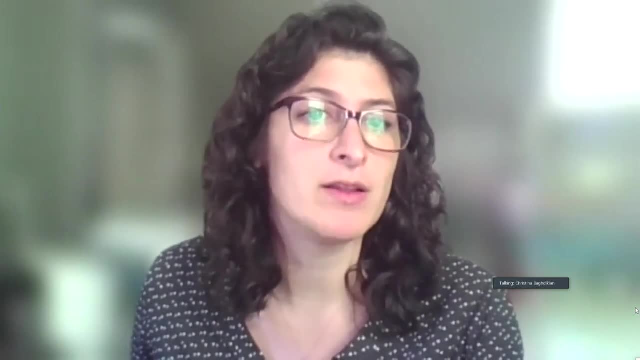 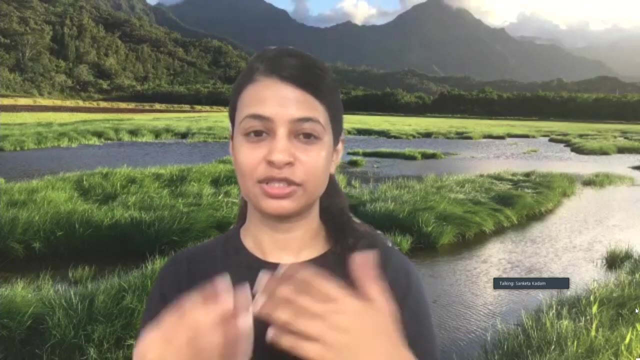 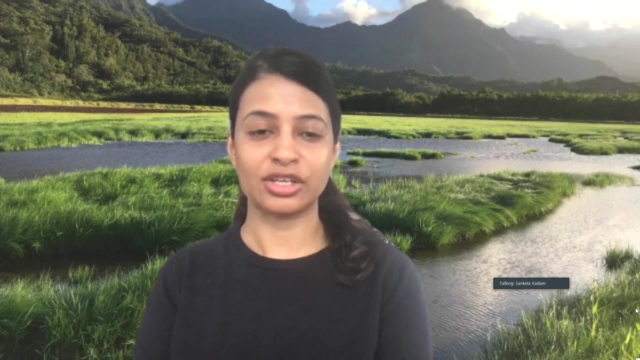 and whatnot, to inform the science and policy? Oh, definitely, I would say yes. So personally, and I will say this first, personally I come from an agricultural community back in India and I really promote indigenous practices back from where I am. 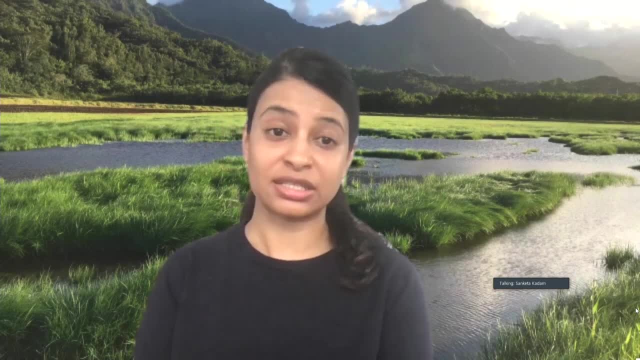 And we've seen this over time- that those indigenous practices are sustainable, They're good for the environment, They're good for the crop yield as well. So yeah, definitely, With the scientist side and the science information side, we do what we call co-production and co-generation of information. 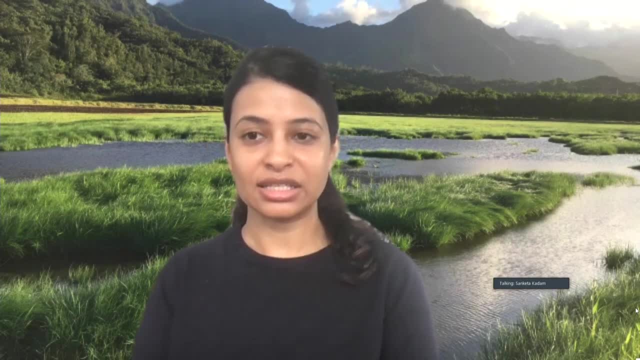 And what that means really is that, as scientists in a field of climate change, it's really important for us to take into account perspectives of planners, of different governments, of different community organizations, to really understand the risk from a local perspective, And, as scientists, what we really try to do is co-generate this information. 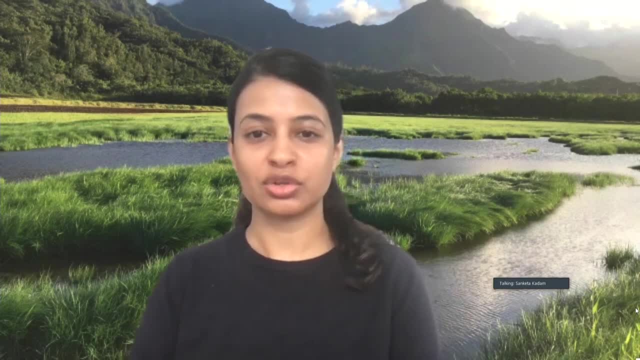 based on what is needed, what is required, but also how can we update the knowledge that you have and vice versa. right, Like you share your knowledge and we share our knowledge, And we really believe in the co-generation of climate risk information. 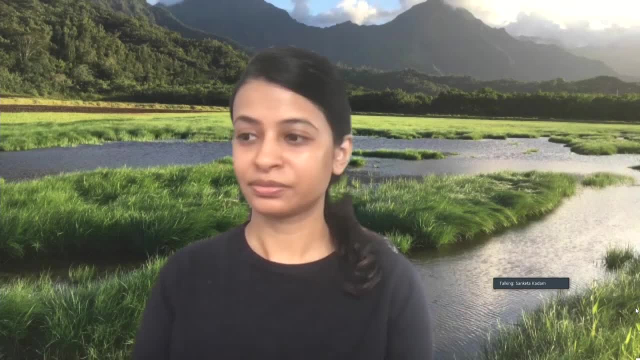 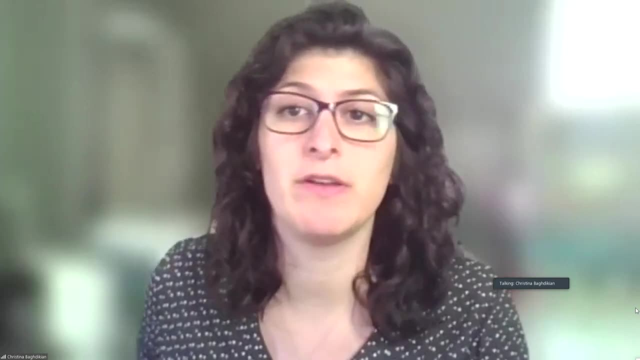 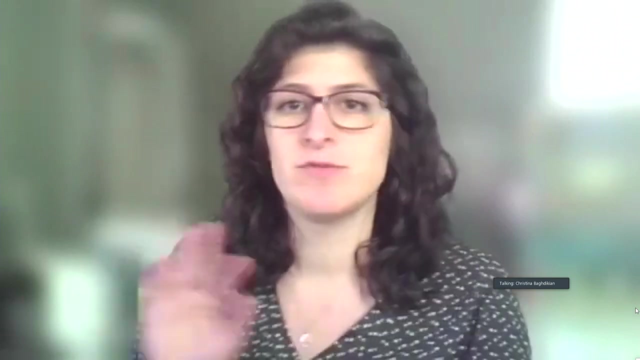 Because there's no other way to really understand risk. That's an excellent answer. And, yeah, that was an excellent answer. The co-generation of information, I think, is a really excellent way to capture and share information. Just a pause to say that, for those of you who joined us late or are just joining us, 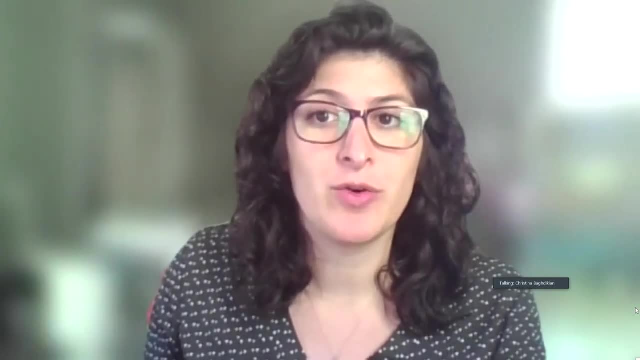 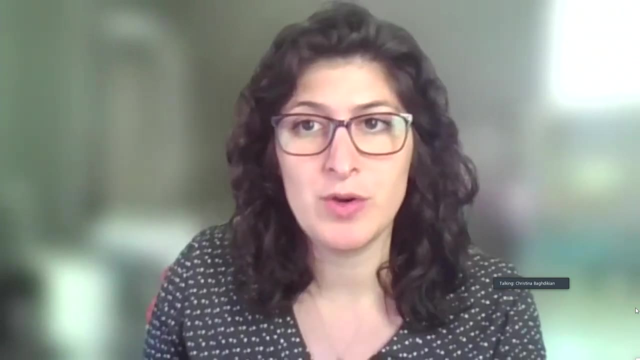 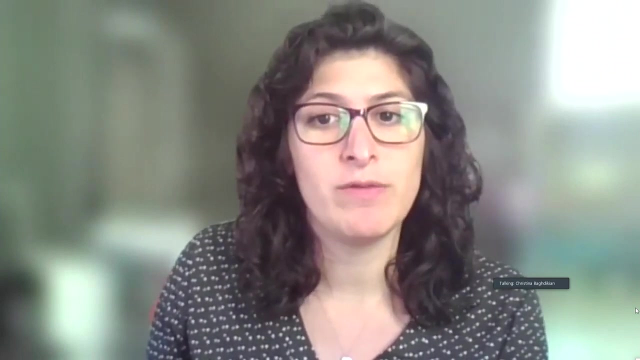 we are capturing questions at the gogreen at hhsgov email, So please feel free to submit your questions to gogreen at hhsgov And, in the future, if you'd like to see the whole video or to share the recording later. 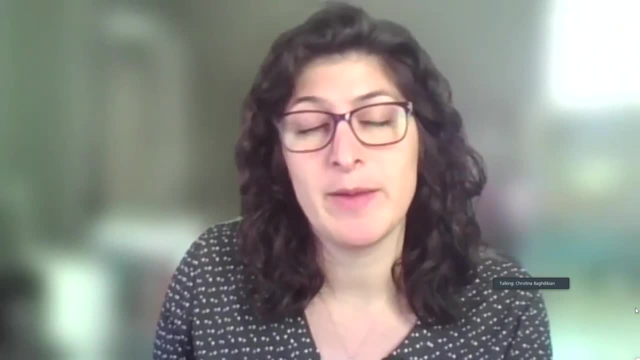 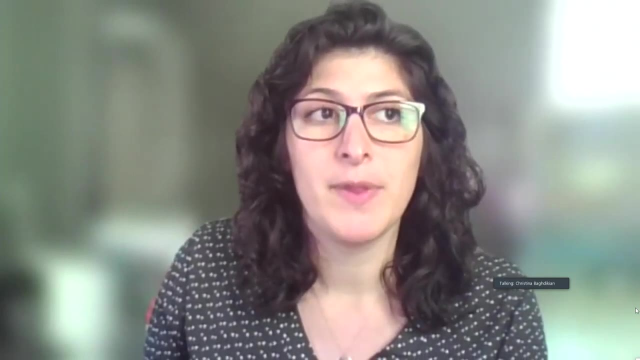 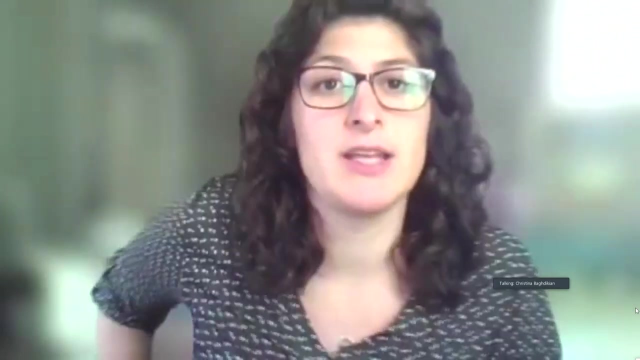 the video will be posted to the Office of Climate Change and Health Equity web page And, if you can, please sign up for our listserv. So thank you. Thank you So you can get the alert once the video is posted, because it does take a couple of days for us to get to get that process and posted. 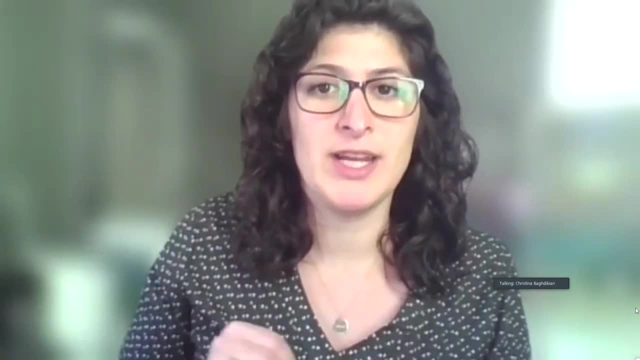 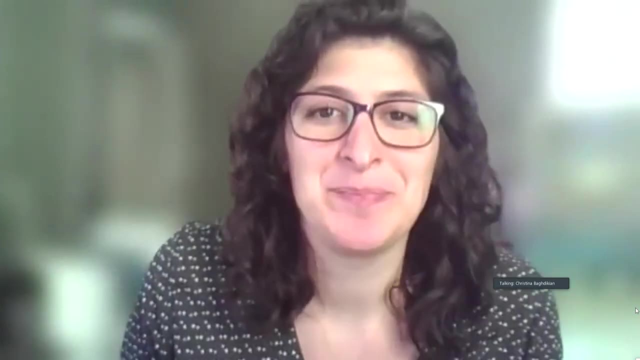 So send your questions via email to gogreen at hhsgov and sign up for our listserv so you know when the video is posted, so you can re-watch and share. All right, We have another question. There's actually a few more questions. 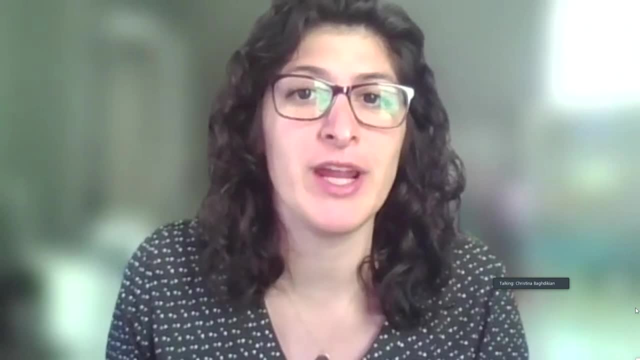 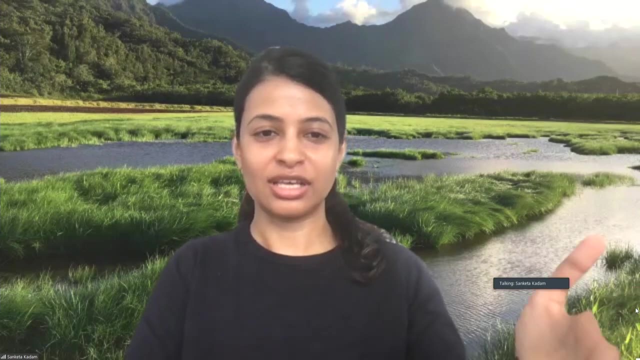 What approach does NASA take to climate change? That may be different from other Agencies like NOAA and HHS, So I had a slide on this, on the actions that we take both on adaptation and mitigation side. I, as a scientist, really work on the climate modeling space and the climate impact research space. 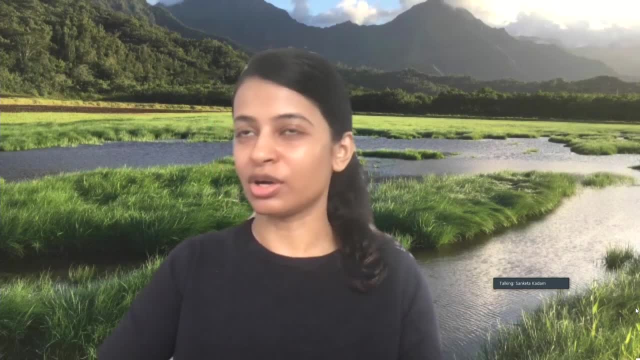 And I would say that you know, as I don't know what actions the HHS takes or the NOAA or the other federal agency takes. I know definitely NOAA works a lot in sea level rise, But yeah, I think for us climate modeling is and remote sensing missions, right. 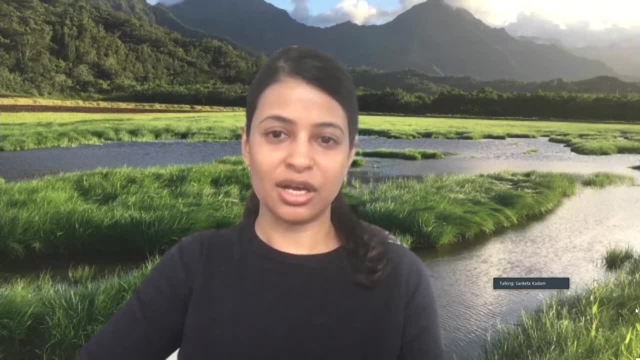 Like you, are able to, in real time, not only observe the actual impacts and changes, but also study them and analyze So through the satellites and the missions. So I think that would be a difference, and I don't really. 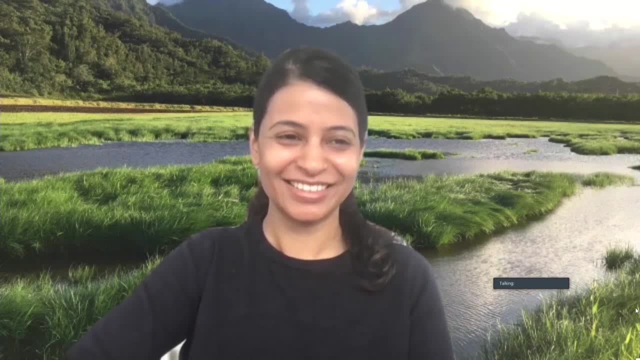 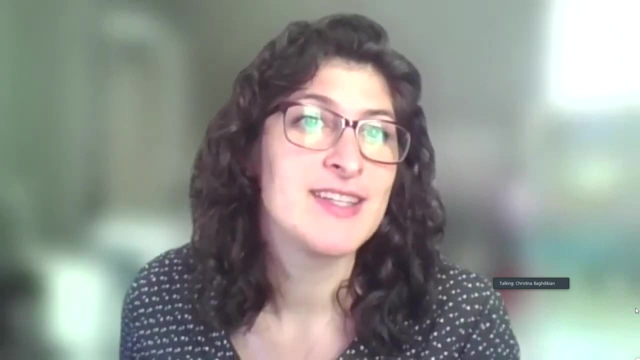 Yeah, I don't really know how to answer that question. Okay, No, I think it's a tough question. If I can help extend your answer a little bit, I guess that it would be what you said. and everybody, all these different departments and agencies, are working within their missions. 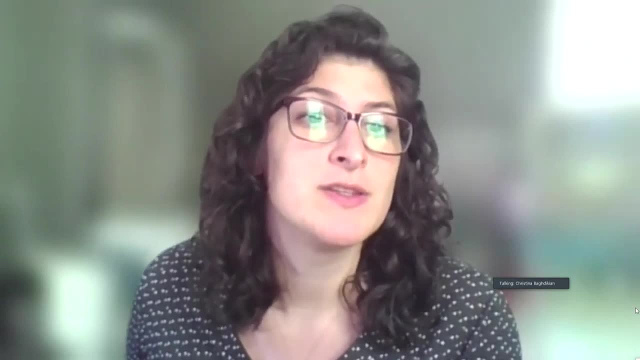 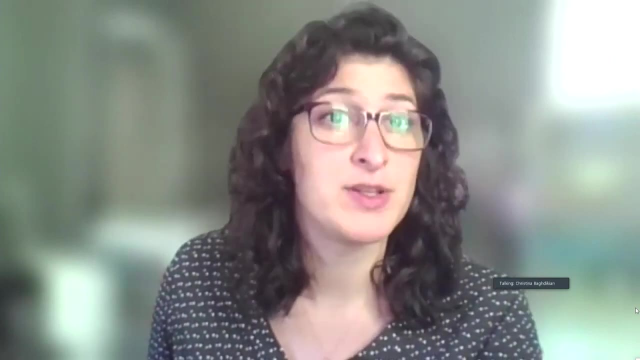 and mandates to answer the questions within their purview as it pertains to climate change. So at HHS, you know we're thinking about health. where others are thinking about what are the systems that are changing and measuring and modeling and whatnot? 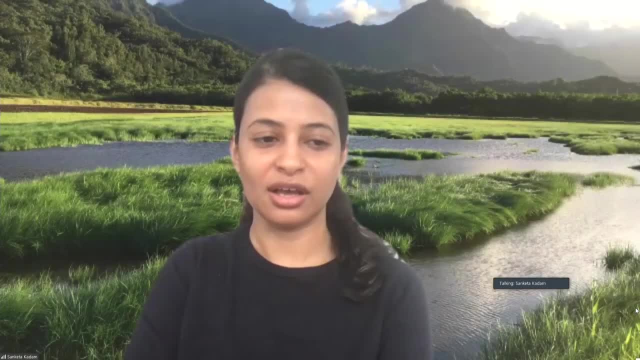 So that was a great answer And we definitely want to promote interagency interactions right, because we can always learn from each other and share data, and share knowledge Absolutely, And it all builds on each other, which is why we're so happy that you're here to talk. 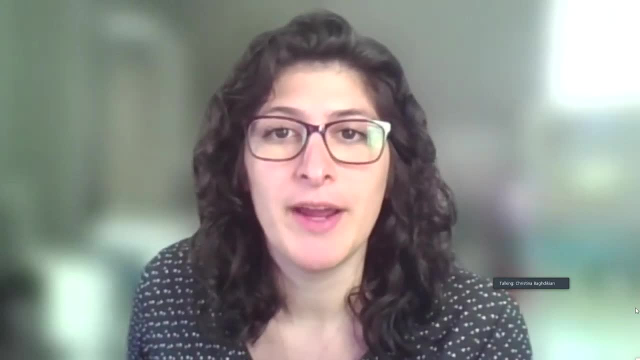 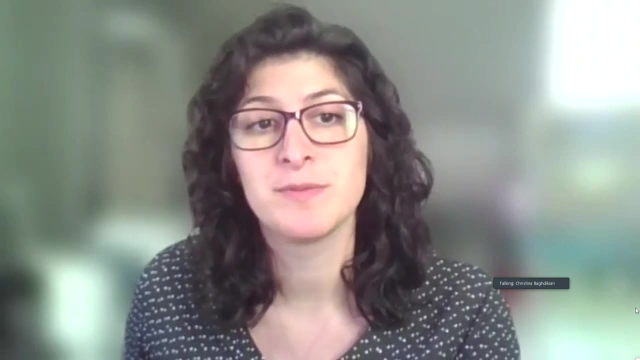 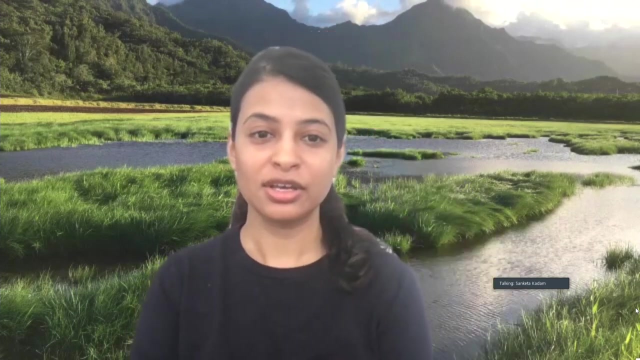 with us today. All right. Are there any studies that predict potential for food production To move north as climate warms? So that's a great question. I wouldn't say off the top of my head it's moving north, but I can, and this is such a. 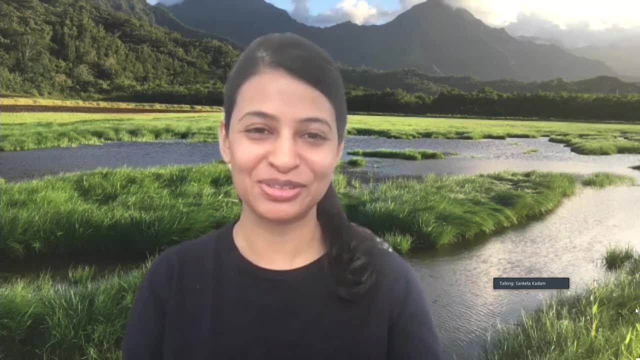 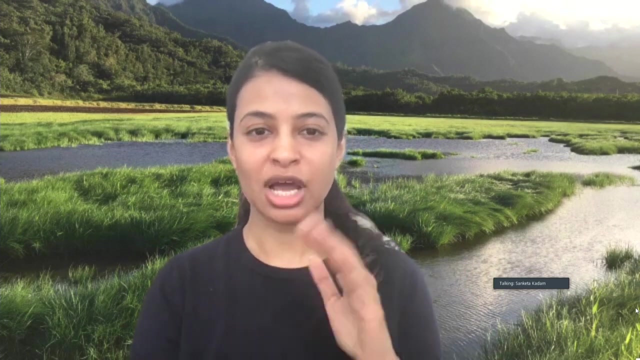 scientist thing to do. but I can cite or give a link to this paper that a colleague of mine worked on last year which really projected the changes in crop yield for maize and wheat, And this was for the high scenarios and this is for the SSP: 5.8.5. 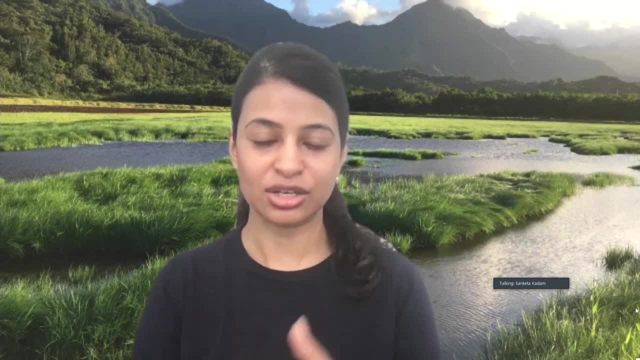 And you know, every time we project we have to follow a certain scenario. We have to see the projections, for what will it be? for the lowest emission, intermediate emission, high emission, because really we don't know where we will end up. 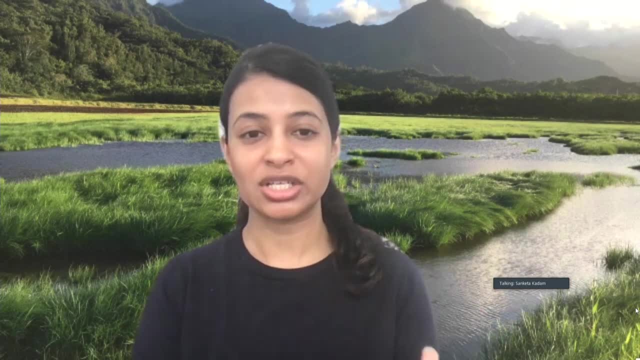 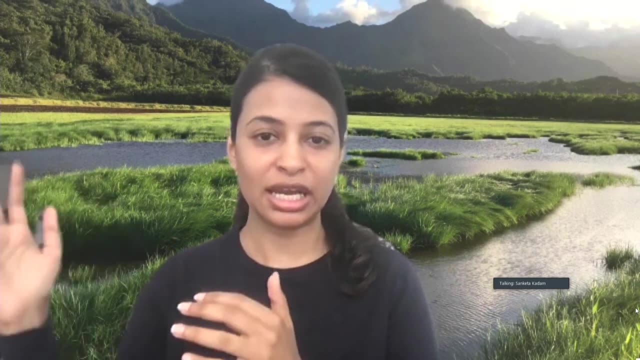 So for the high scenario, this paper really talks about the changes in crop yield and it's very interesting. It's interesting to see that in 2050 or 2070s, 2080s, some of these regions will see an actual 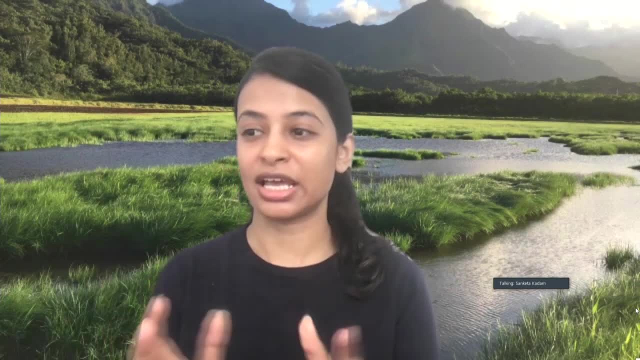 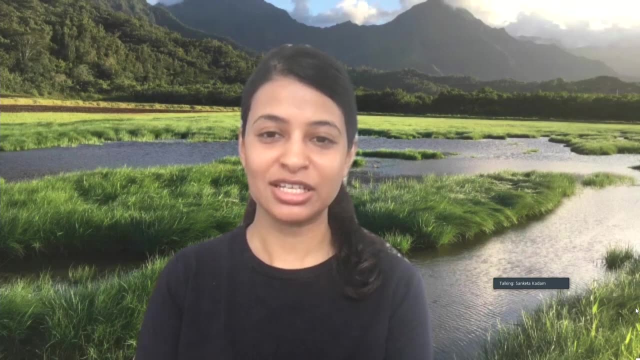 increase in production and some will see a decrease in production And I will love- I would love- to send that paper. It's by Jonas Jägermeier, if you want to Google it, and there's a really pretty graph. 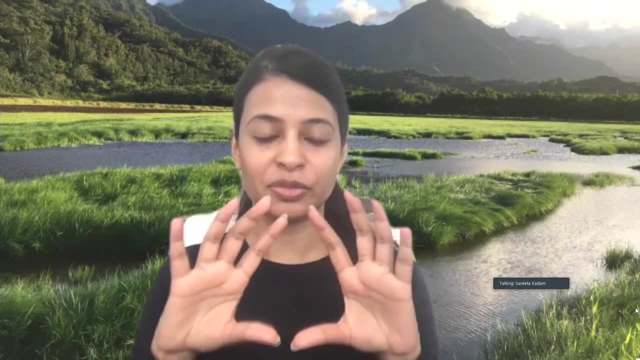 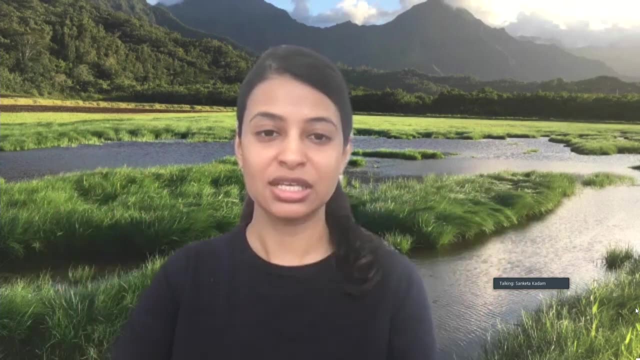 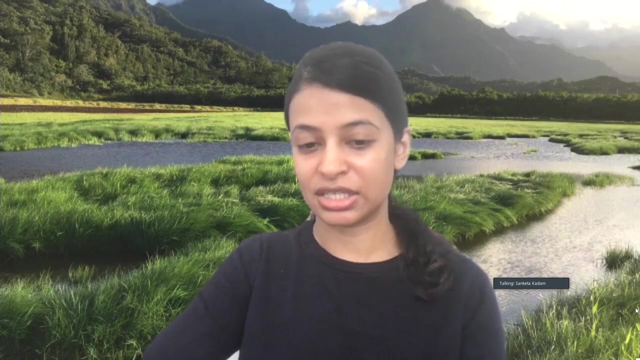 and I should have probably included it in the presentation of the production of the global map, And you can see the changes in yield. So that's an interesting question. We do have a lot of studies. yes, definitely. if you're more interested, there is AGMIP. 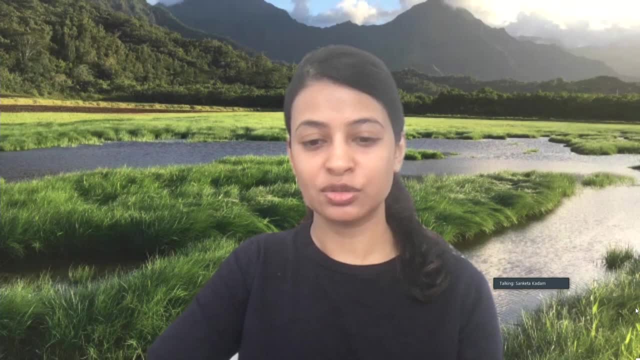 A-G-M-I-P section of our group. It's at NASA, GISS, and they only study on food production and crop systems, So they'll have a lot more studies that you can look at. Awesome, Thank you, And if you share the paper with us, we can see if we can link to it in the chat. 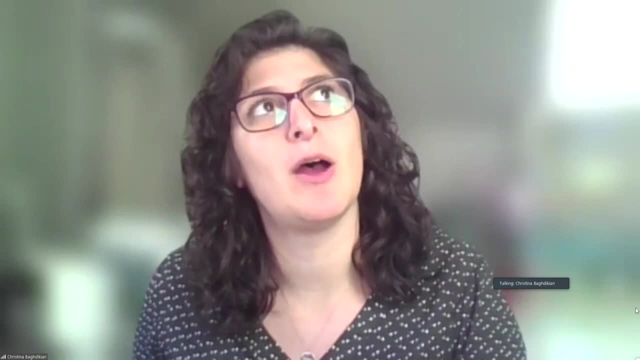 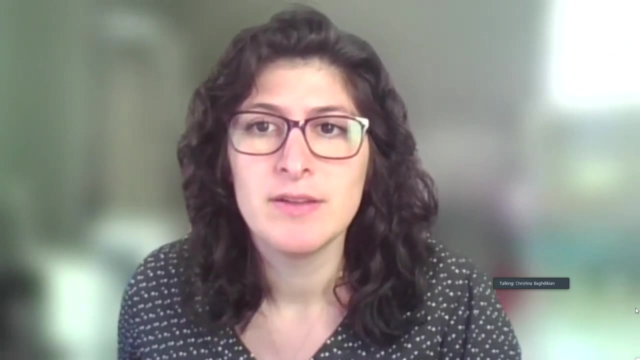 And I'm going to put it in the chat, Thank you. Thank you, And I'll put it in our listserv announcement when it goes out. All right, Let's see. Do the climate models factor in potential tipping points like great glacier melt and? 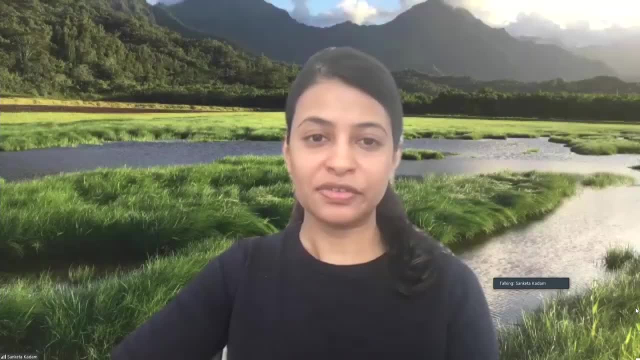 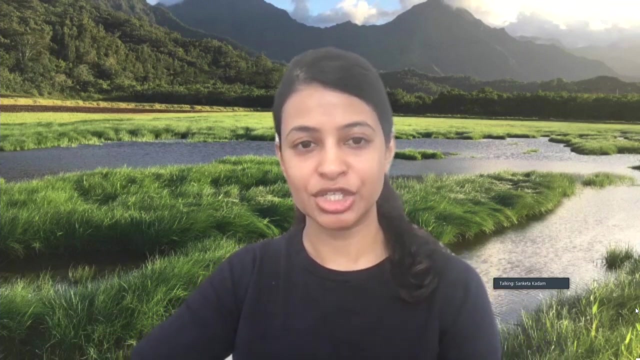 deforestation. Yeah, so they do definitely factor in, and by factor in I mean they will predict and try to project those tipping points, Like I said, for when we're talking about the climate models. Yeah, Yeah, Yeah, Yeah. 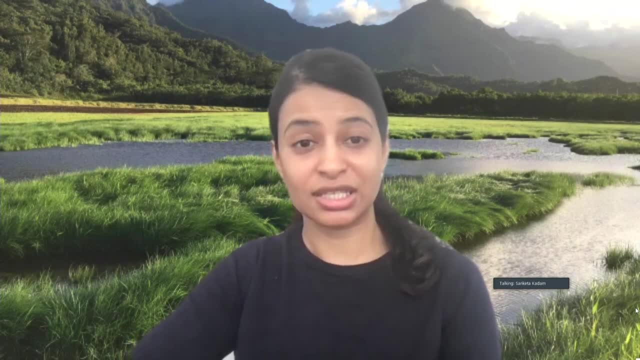 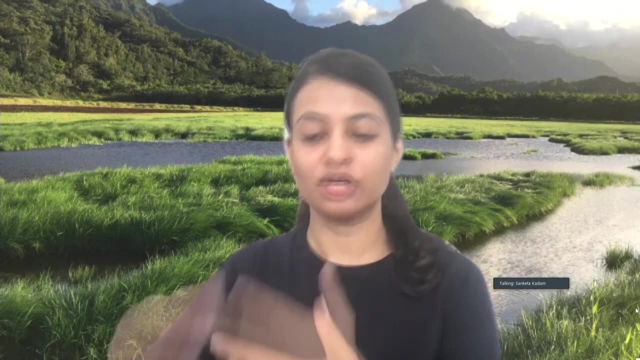 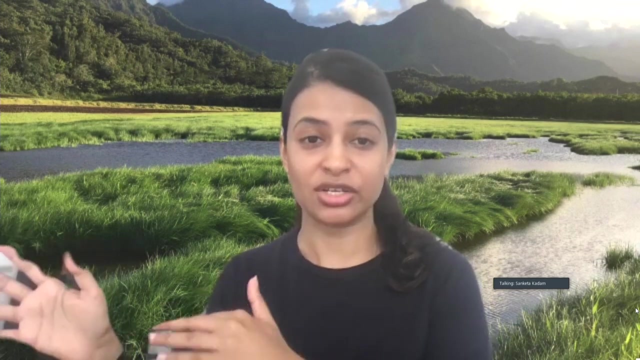 Yeah, So when we're looking at the climate models for Atlantic circulation, the models aren't predicting it for at least the next hundred years. So when we are modeling the existing climate system and when we're looking at particular tipping point, we try to gauge what's the current status and how it will change in the 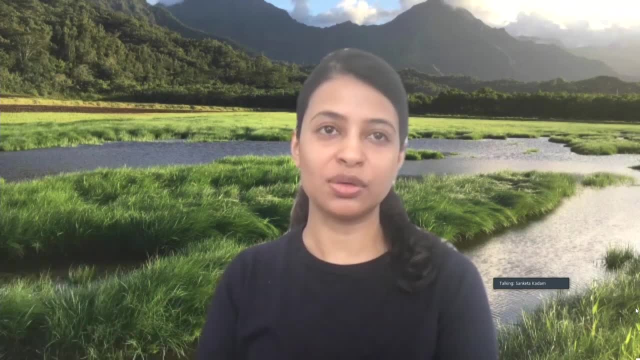 future. But again, it all depends on really what the warming levels are right, Like when we were looking at the Atlantic circulation, the scientists and the modelers. they were only looking at the climate levels And the modelers were not looking at the climate levels. 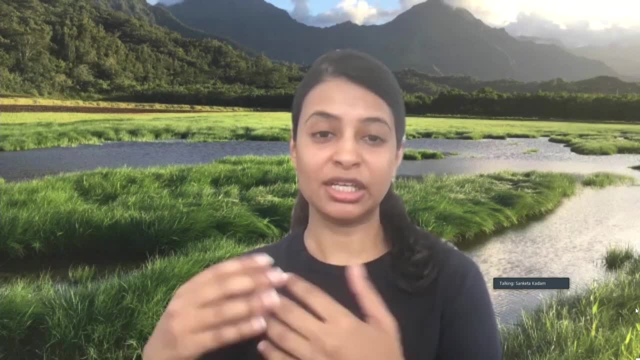 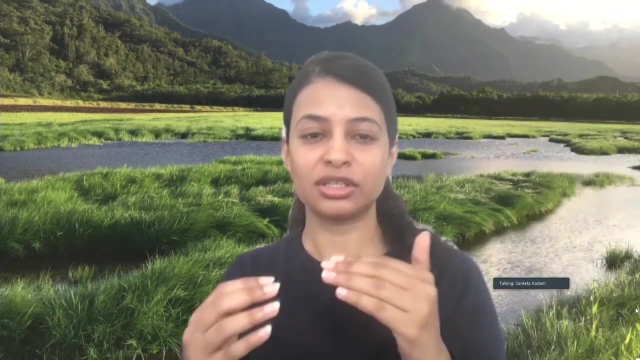 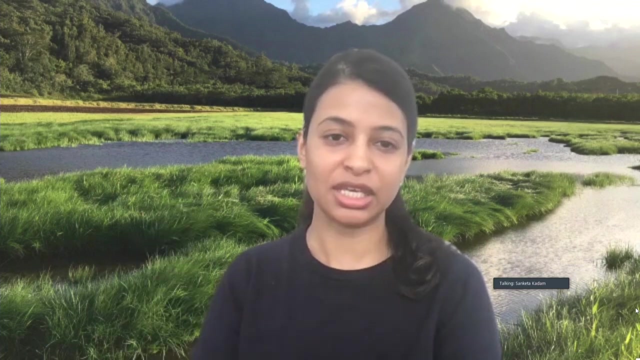 the scientists and the models only see it completely shutting down or failing only after we reach a certain degree of warming. So again, the uncertainty around tipping points really comes from where we are, what the level of warming is and how the systems will react to that level of warming. 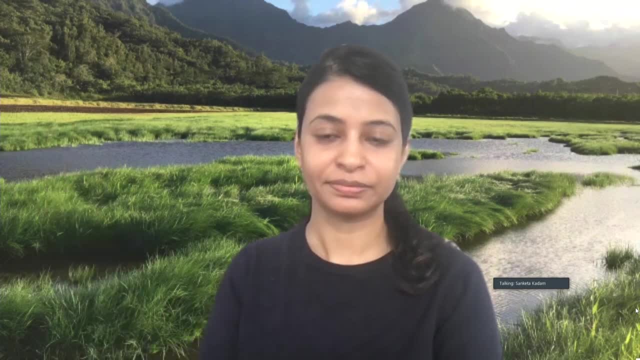 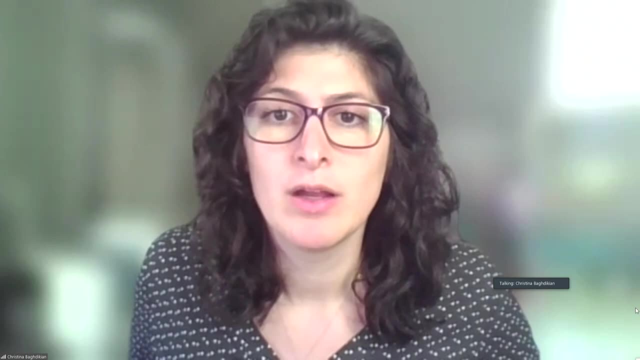 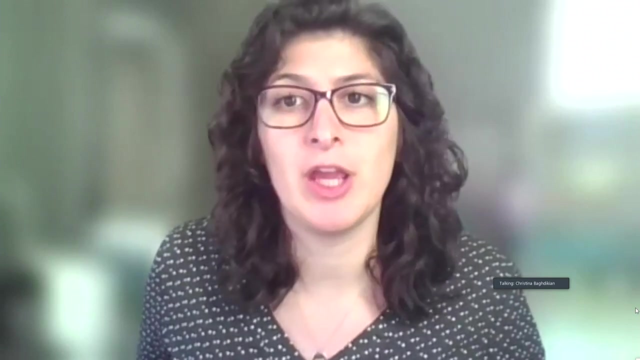 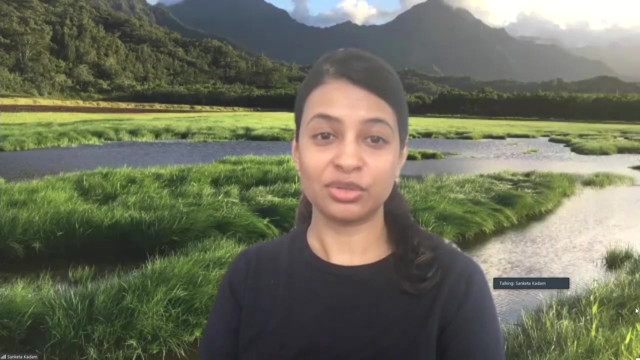 whichever path we follow into the future. Awesome, Thank you. I'm just trying to interpret the next question. I think I know what the question is: Does NASA have a carbon capture group or engage in carbon capture research? Well, now that I know that's a good question. If they do, then I really need to find out, but not that I'm aware of. 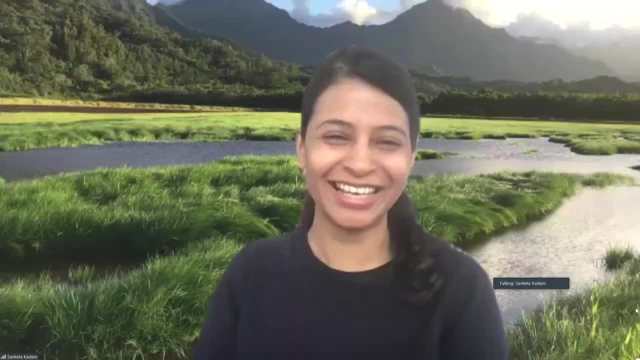 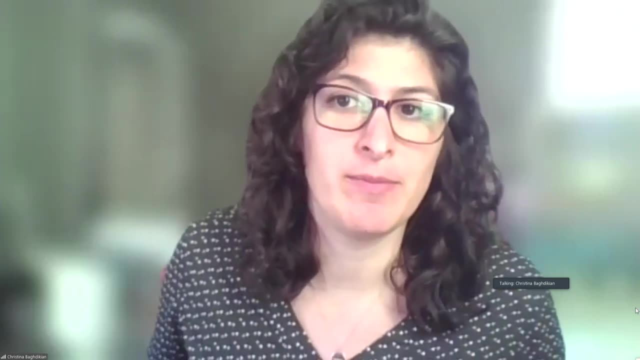 Awesome. Okay, Let us know if you find out. Okay, So how can I like this question? How can the How can the younger generation school kids participate in your program? Is there any website information that you can share, or just your email? 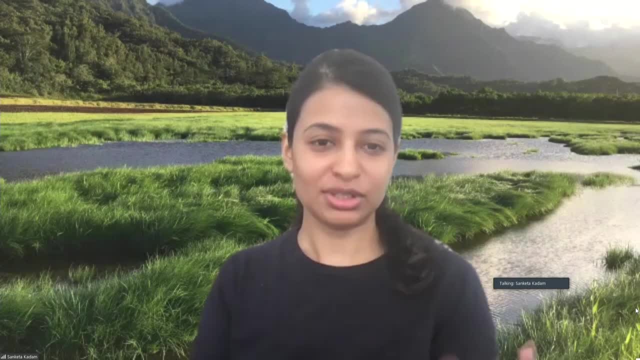 Yeah, that's such a great question, Oh my God. So, like I have the last link on my slide, which is called the ARSET A-R-S-E-T ARSET training And they have a bunch of different trainings on, you know, impacts of climate change. 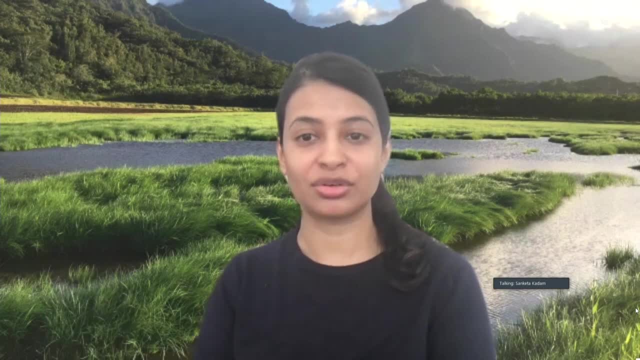 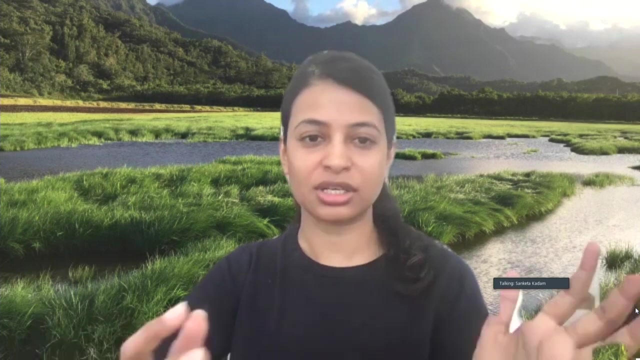 What does remote sensing satellite data tell us about climate systems? The actual training is called Climate Change Basics and Remote Sentence or something like that, But there's a whole two-part training on just the kind of thing that I showed you right now, which might be a little too much for school kids. 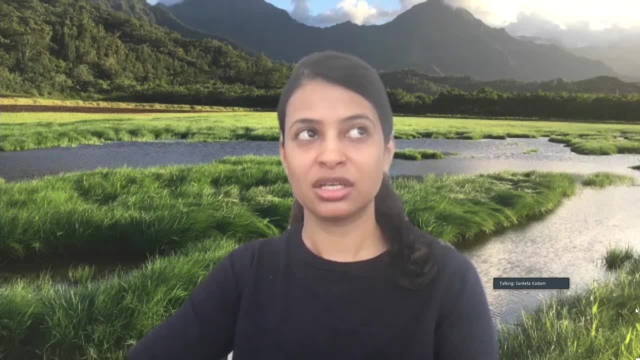 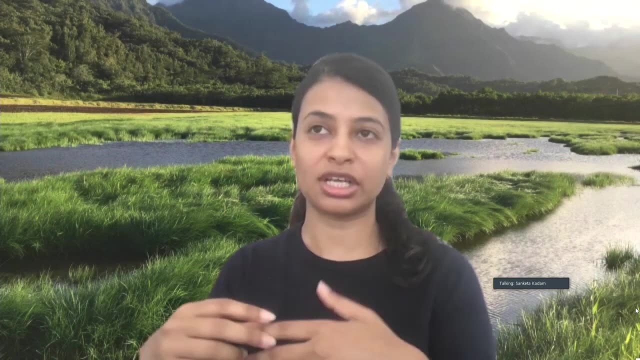 There is another program through NASA, GISS, called CCRI Initiative, where they actually go and teach or create awareness or give these trainings to K-12 teachers and the teachers in turn then try to talk about it in their classes. So we do have this program, which a lot of it is involved with training the teachers and training the high school teachers and K-12, I think. 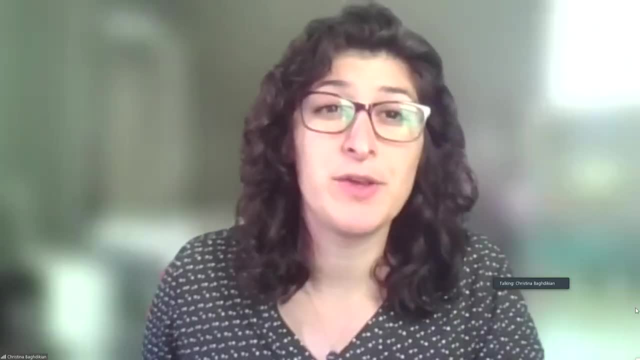 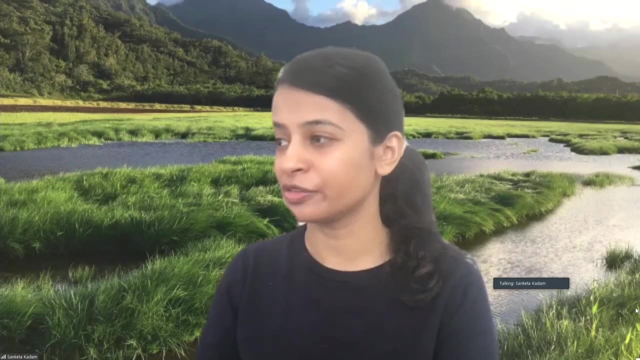 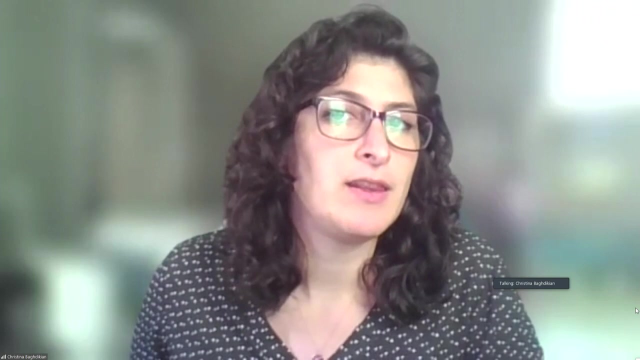 But yeah, we do have those programs. That's awesome. I think you said CCRI is the CCRI. yeah, They have a K-12 program and I can get more information on that. definitely, Okay, and do you want to show the last slide where you had that information while I kind of set up the next question? 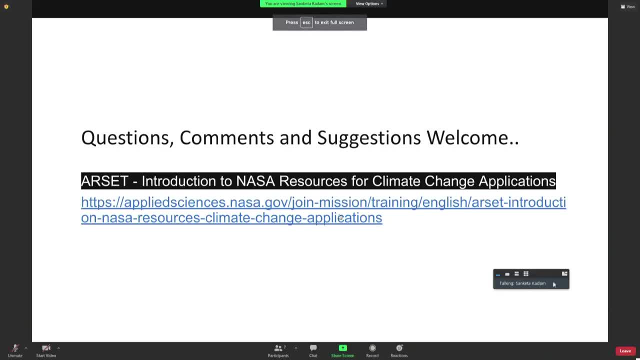 Awesome. So that's what it's called. It's the Introduction to NASA Resources for Climate Change Applications, But it has it's a two-part one. So the first is all climate basics. It's a lot more information. It talks a lot. 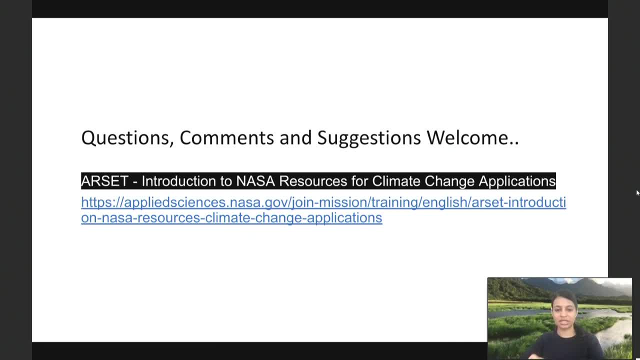 A lot more about using models, but also remote sensing, And they give a lot more examples which can be really tangible to understand. That's awesome. Thank you, Let's see. I think we have time for at least one more question. 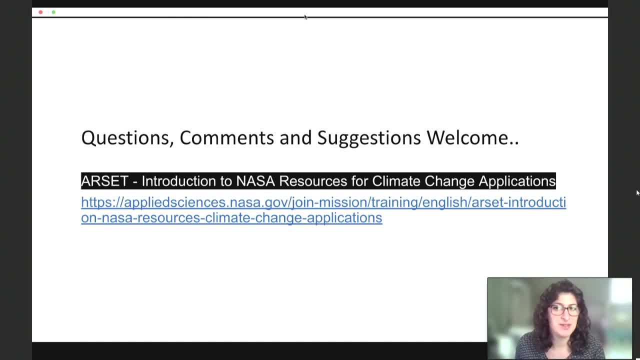 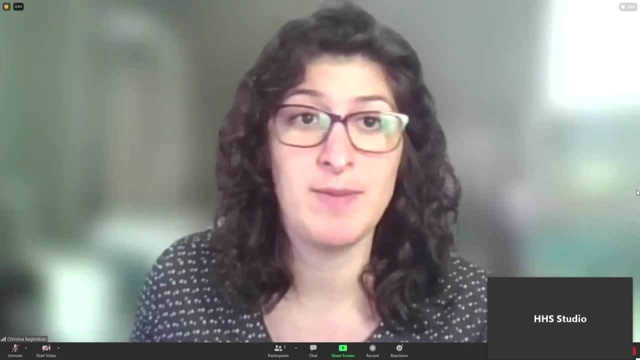 This has to do with changes from the pandemic. So during the last two years of the pandemic, many people have been working from home instead of driving to work. Has this had a measurable and maybe positive impact on On atmospheric gases and compositions? Yeah, there has been. 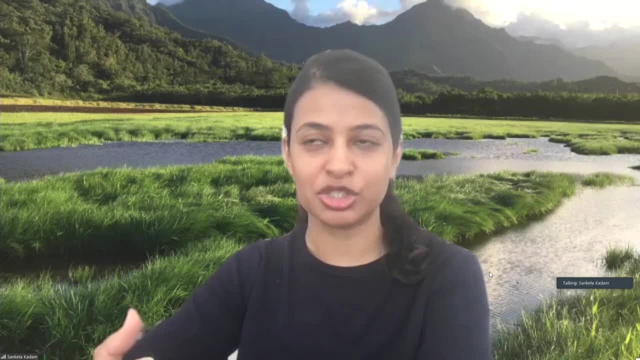 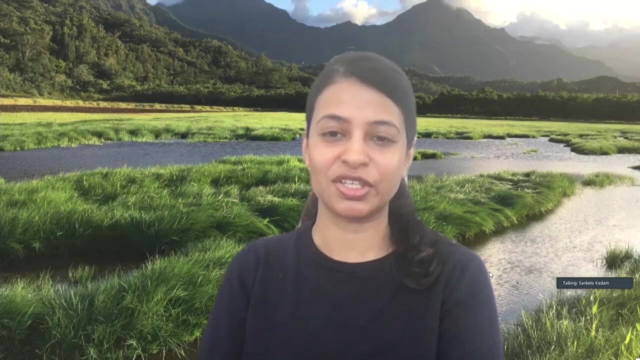 So there's this thing called the Keeling curve, which was started by the scientist John Keeling, I think, And what it does in Hawaii's Mauna Loa lab. what it does is really measures the amount of CO2 concentration in the atmosphere. 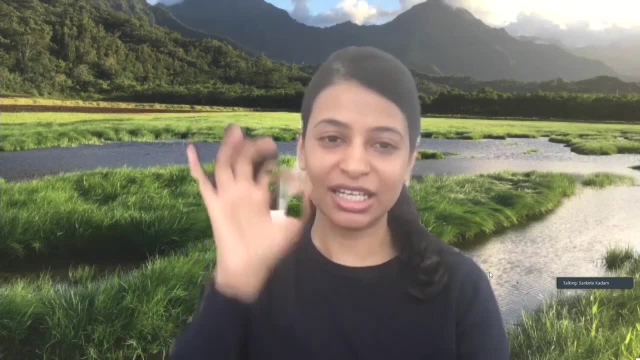 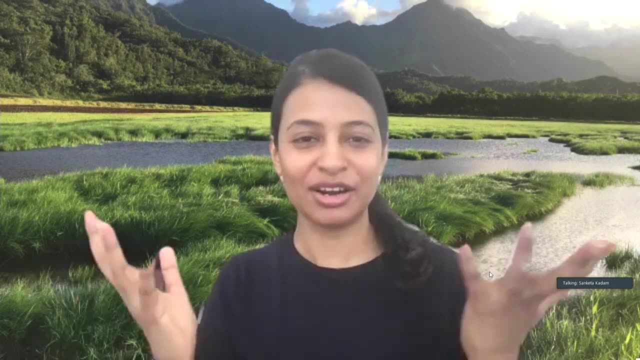 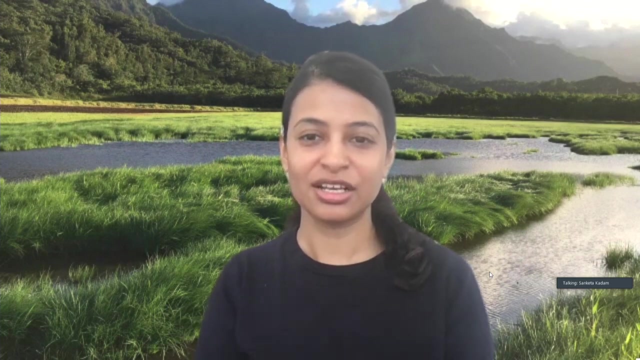 And they update it every day. So there was a little tiny dip in 2020, but we're up again, So didn't really make quite a lot of difference. It's a tiny little dip, but you can definitely see that. you know, the pandemic had some sort of impact. 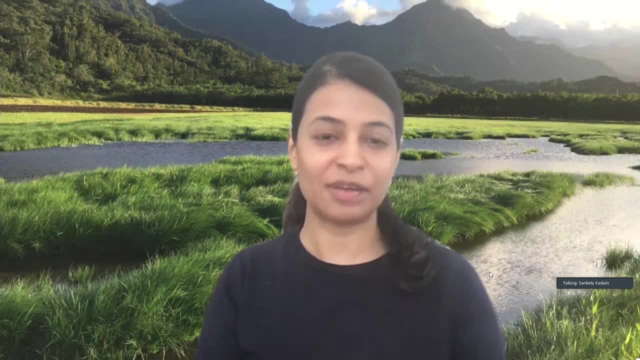 There was, there were studies- I'm not studies, but obviously I mean I have family in Delhi- that we saw a difference in the air quality, because Delhi now has the worst air quality. It's one of the cities that has worst air quality. 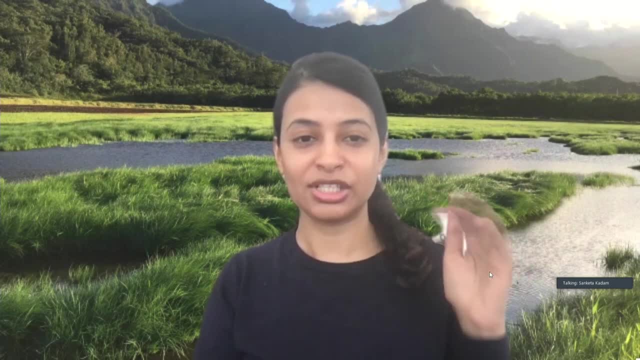 And during the pandemic it had really slightly improved. But yeah, that was some of those observations that people saw in their day-to-day life. It's little changes, but I think we reverted back to what we were before very quickly Excellent. 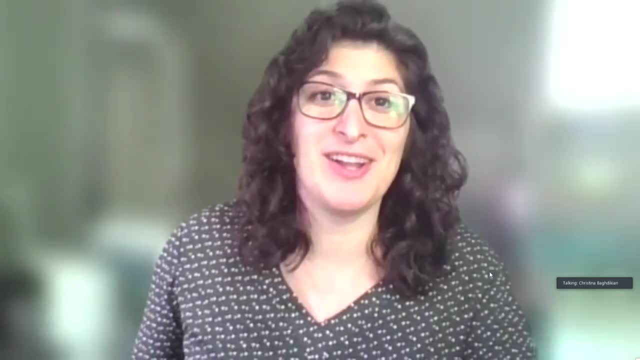 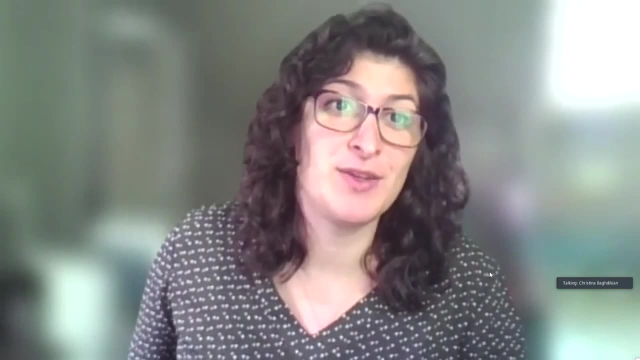 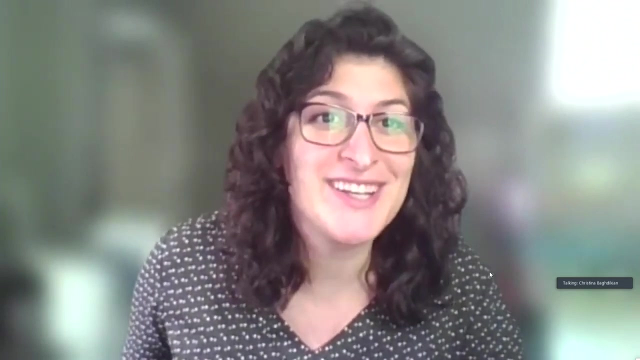 Thank you so much. I think we all learned a lot today, and from both your personal experience and also your professional experience, research and expertise. So thank you so much for coming today. Thank you to all the folks who signed on and joined us. 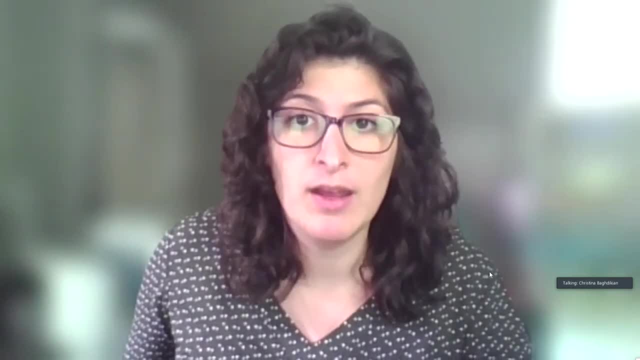 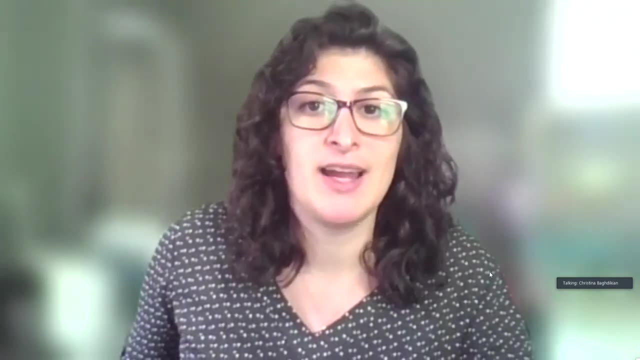 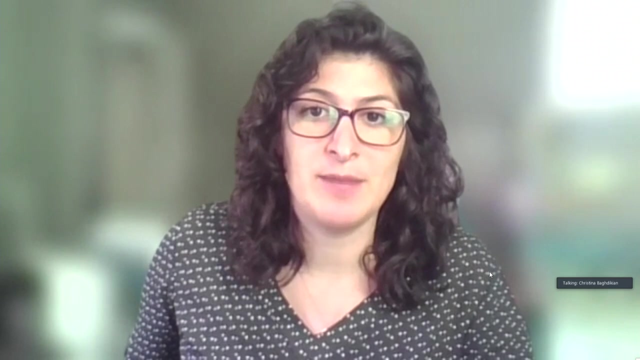 Really appreciate the attention and time and the questions coming in. Before we close out, I do want to remind everybody to join us the same time tomorrow to hear from climate scientist and award-winning science communicator, Tom de Liberto from NOAA, who will discuss climate change impacts, adaptation and resilience. 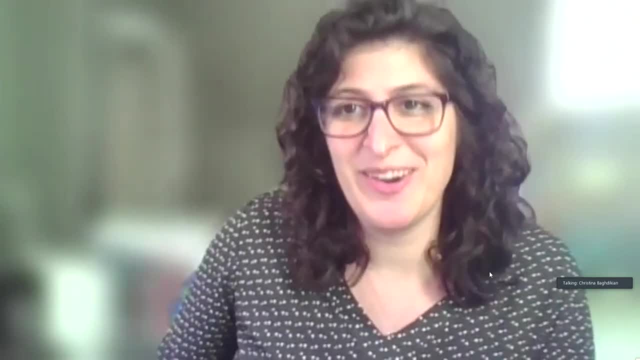 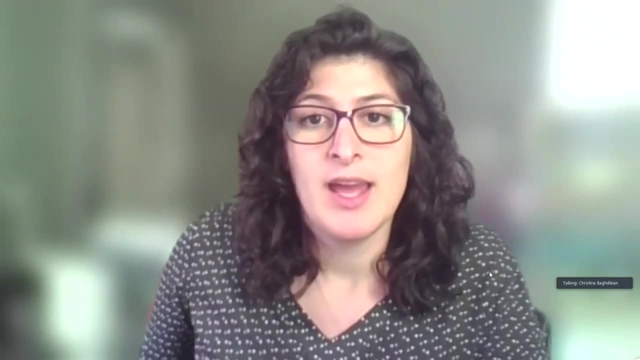 And on Thursday also at noon, to hear from our very own, from HHS, Dr John Valdez, who is the interim director of the Office of Climate Change and Health Equity, and he will discuss climate change and health equity at HHS. 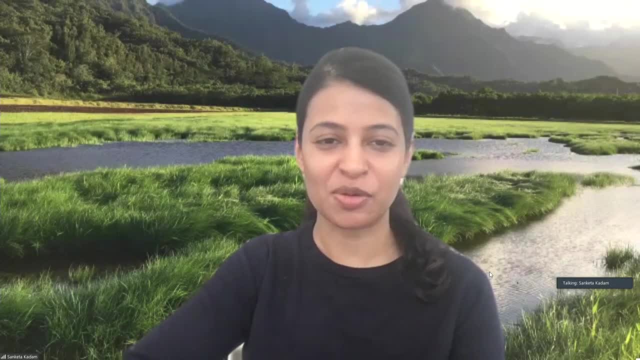 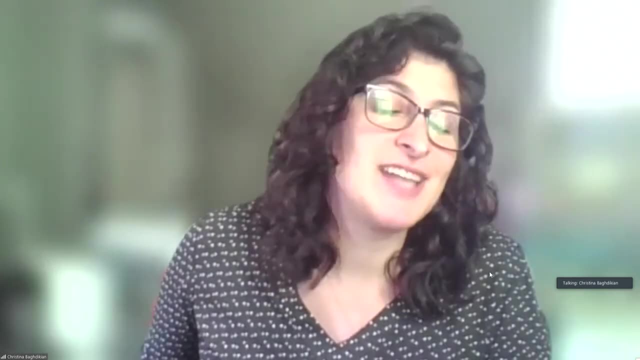 Thank you. Thank you so much for having me, Thank you for giving me this opportunity. It was fun And all the questions were great. Thank you everyone. Sankita, you're awesome. Thank you so much. Have an excellent day. 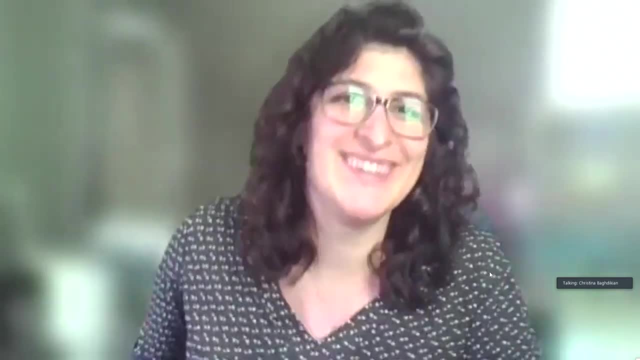 And I hope everybody has an excellent Earth Day week. Bye everyone, Bye. Have a good day.